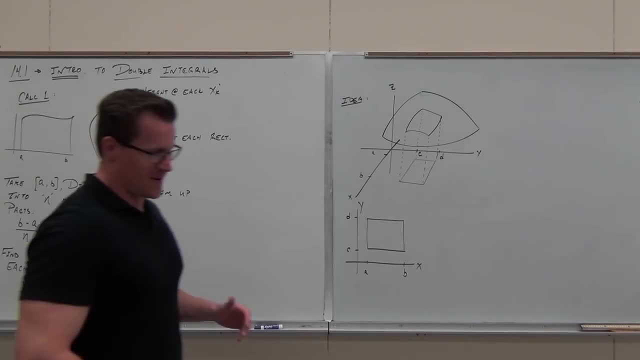 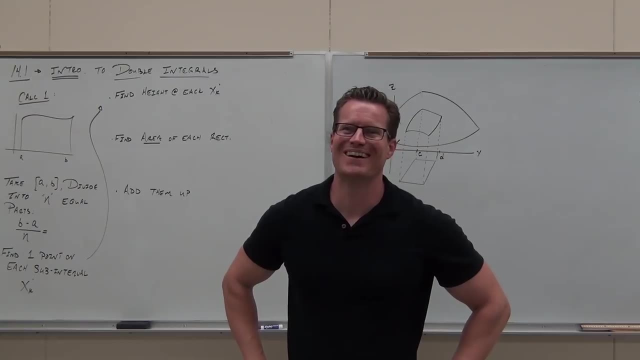 So we have a brand new world. I'm going to give you an introduction on these things called no, it's not a thing. You're joking, Leonard, It's not. no, Yeah, double integrals. Say double it. Yeah, C double. We can do double integrals. Now, what in the world do they mean? 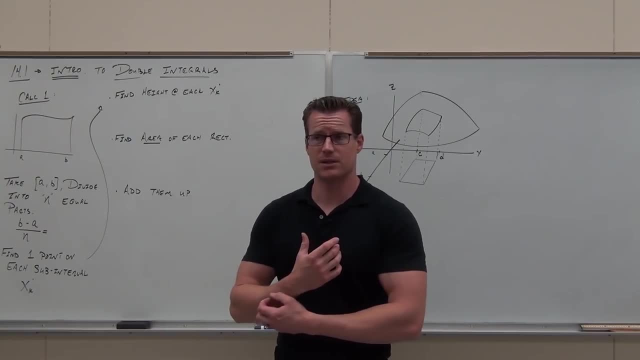 and how are we going to do them? That's what this lesson's about. It should be a quick lesson. all right, We're not going to spend too long time on it, because I want to get to the actual practice of doing double integrals. But I do want you to notice the connection to Calc 1.. We're 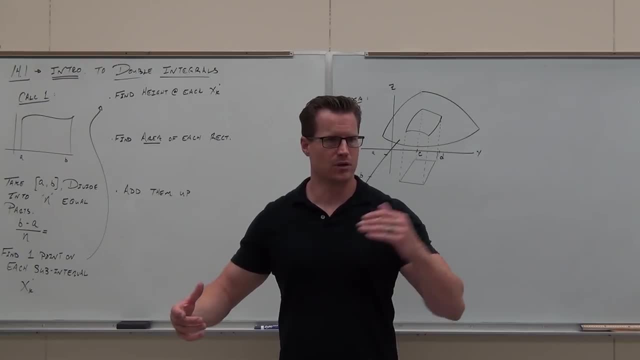 going to walk through how Calc 1 is very quickly, maybe five minutes. Then we're going to build double integrals from the Calc 1 idea. Does that make sense? So Calc 1, the second part of the calculus question from Calc 1, first part was find the slope of the tangent line to a derivative. 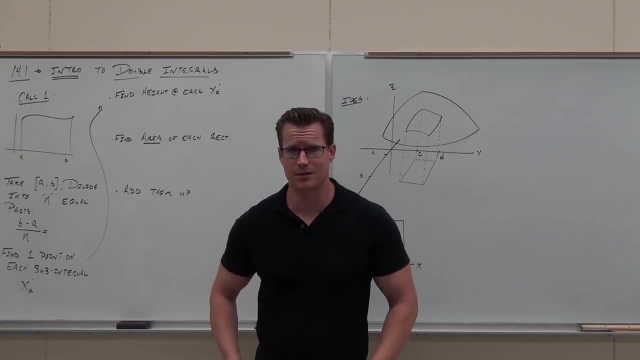 point. We nailed that with derivatives We've done that. a freaking ton in this class. The second part of the calculus question from Calc 1, first part was find the slope of the tangent line to a derivative point. We nailed that with derivatives We've done that. a freaking ton in. 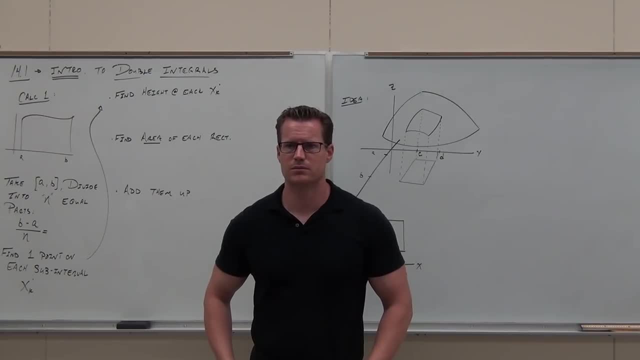 this class. The second part of that two part question is: how do you find the area under a curve And how we did it in Calc 1 was like this: We took a finite interval from A to B under a continuous curve And what we did was we cut that interval into a whole bunch. 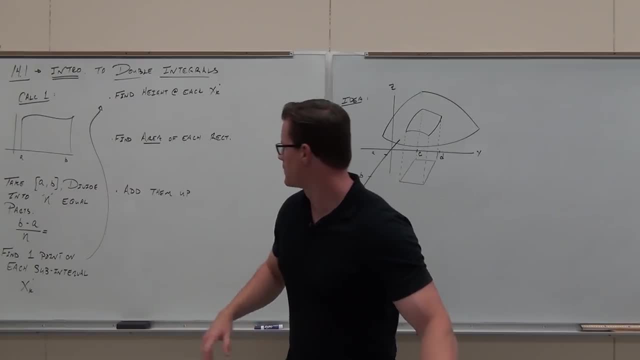 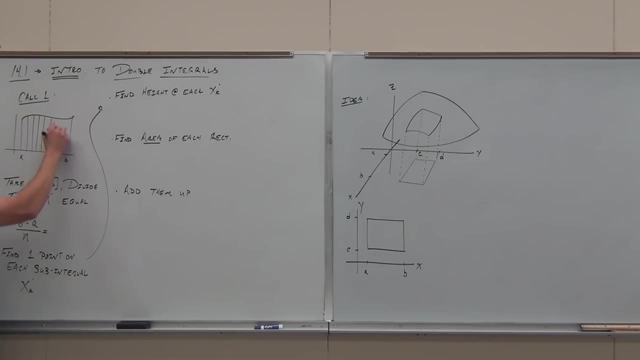 of little segments N of them. So we took A to B and we made a whole bunch of little segments N of them. So we took A to B and we made a whole bunch of little segments N of them. So we took A to B and we divided it into N equal rectangles. 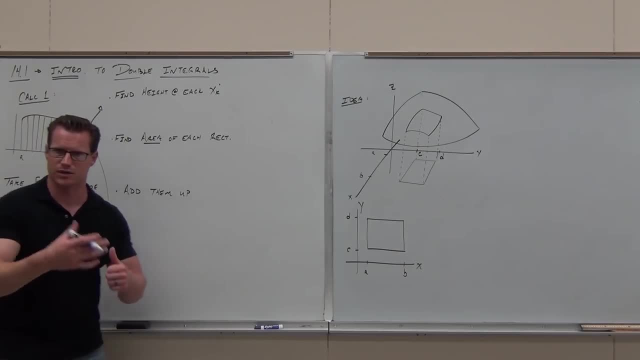 So we took A to B and we divided it into N equal rectangles. So we took A to B and we divided it into N equal rectangles. Is this ringing a bell too at all? It's called Riemann's Sums. We'll get there in a second. 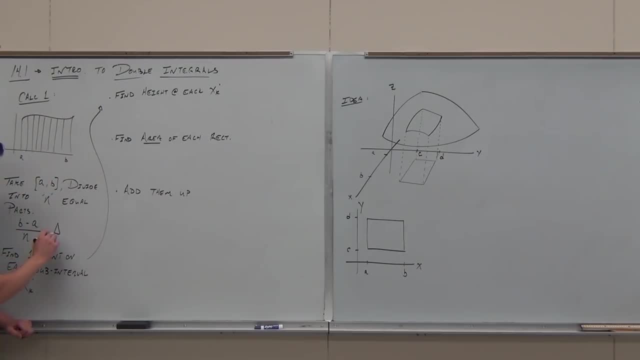 Okay, So B minus A divided by N would give. if I take this interval and I divide it by the number of equal partitions in there, I'm going to get the width for each partition. This is the width of each rectangle, Is that? 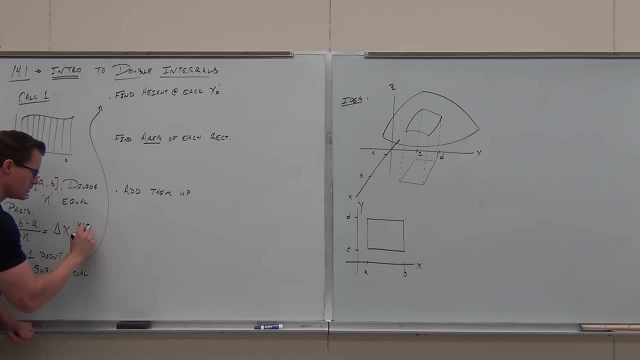 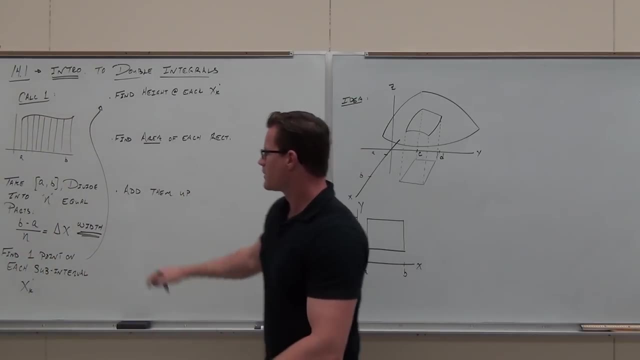 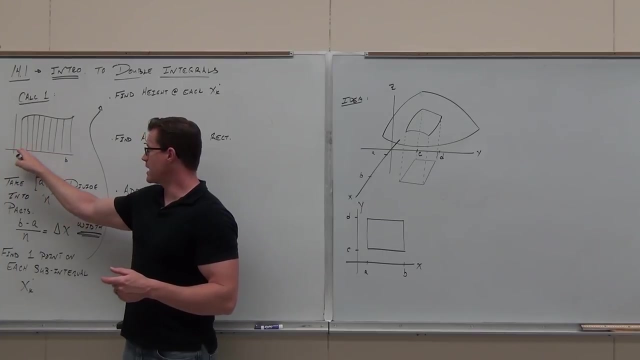 clear for you. That's how the math works here. Width of each of those: they're all the same, all the same width. Okay, fantastic, Let's find one point for each of those subintervals. So at each point on here on the x-axis, I'm going to have one x value. We call that x sub k dot. 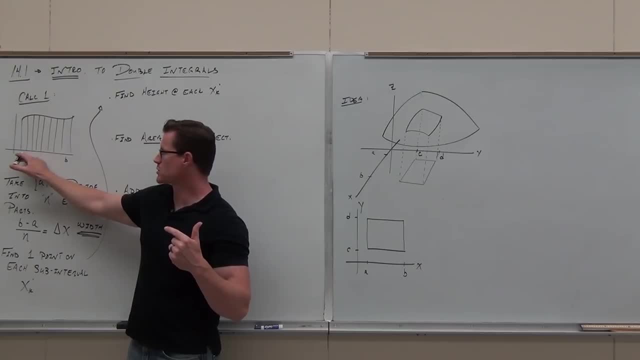 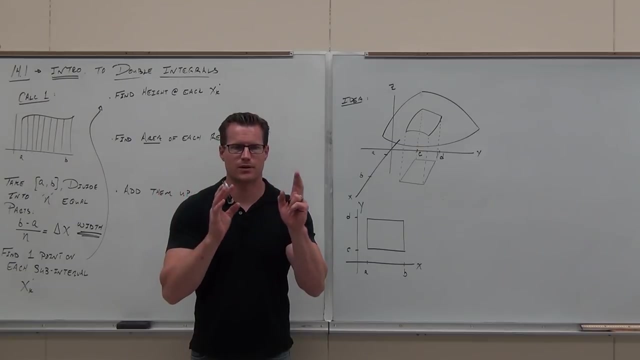 What that means is that for each one of these intervals- one, two, three, four, five, whatever- I'm going to find the x for each one of those. So the x in the first interval, x in the second, x sub k, the x for each interval, And the dot means it can be anywhere. It can be anywhere in. 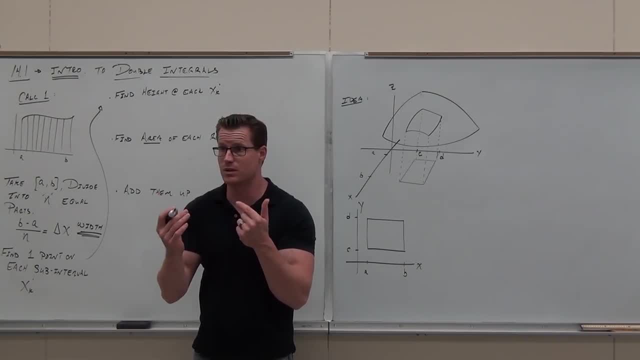 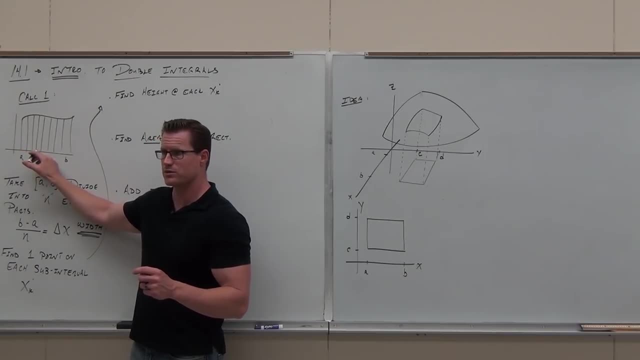 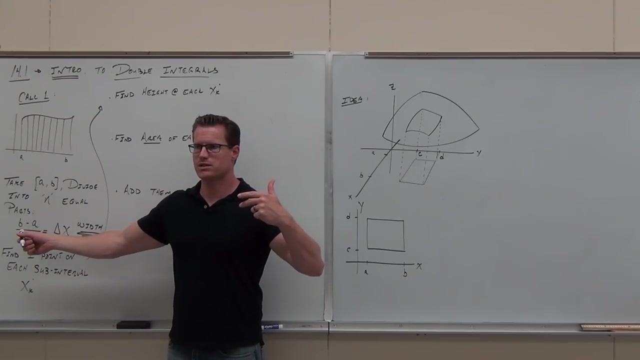 there left, right, center, somewhere between. We typically pick the center, but it doesn't really matter. The dot means it's an arbitrary choosing of some point on each little value. So cut it into a whole bunch of partitions. How many N of them? A lot of them, A lot of them. What's the? 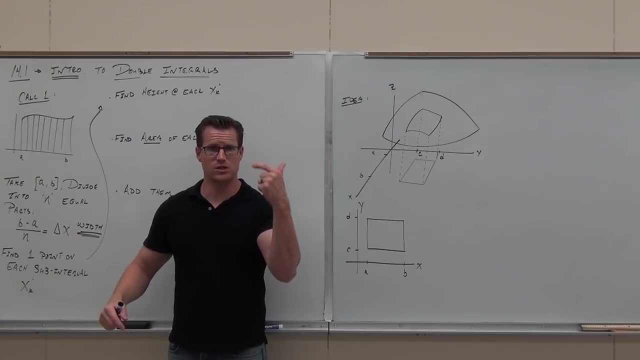 width of each one? Well, it's an interval divided by the n. That gives you the width for each segment. Okay, that's a width of a rectangle. You guys get it. Well, to find area, we need a width and we need a height. 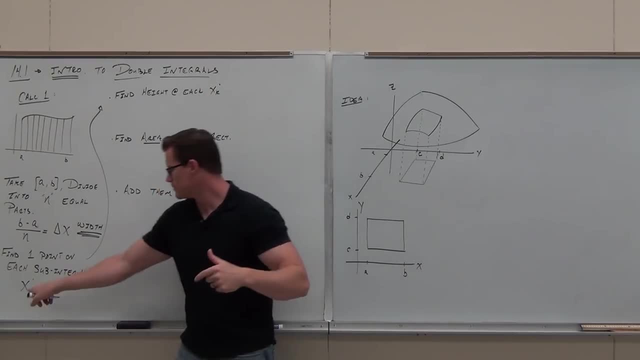 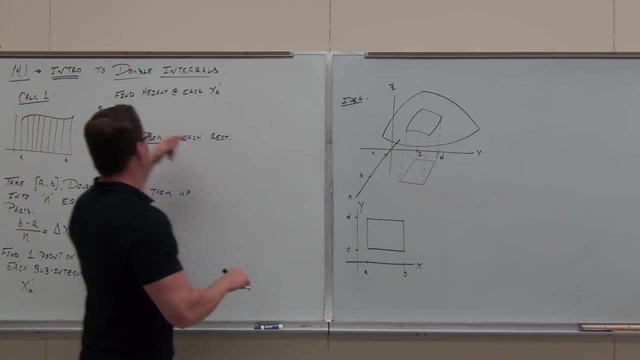 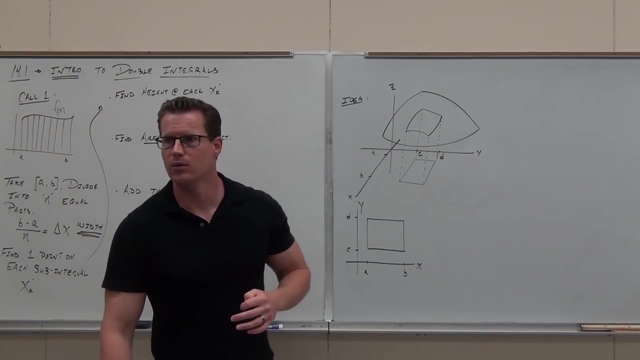 How are we going to find a height? Let's pick a random point in there For each interval, each interval. pick a random point: x, k, dot. Now find the height at each of those points. Okay, find well. what for the history of the world gives us heights? 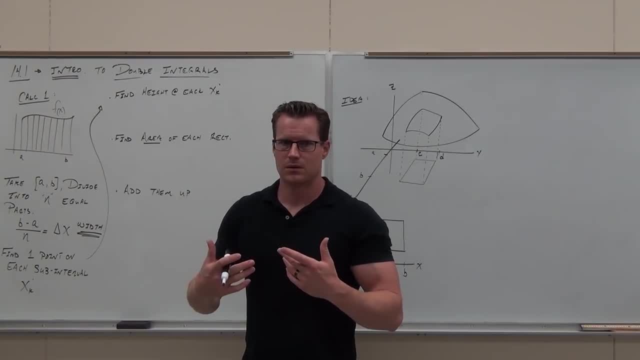 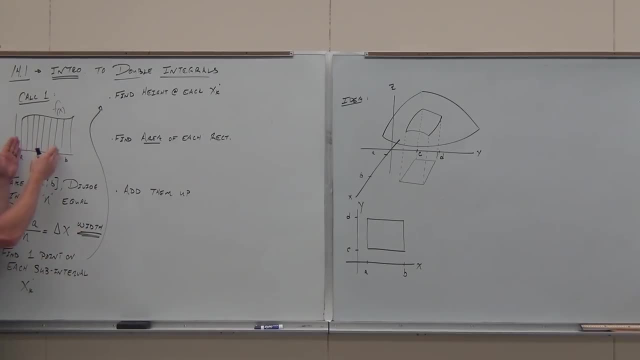 How do you do it? How do you find heights of points? What do you do? Plug it in, plug it into the function. So if I have a whole bunch of different intervals and a point for each of those, on each of those little, 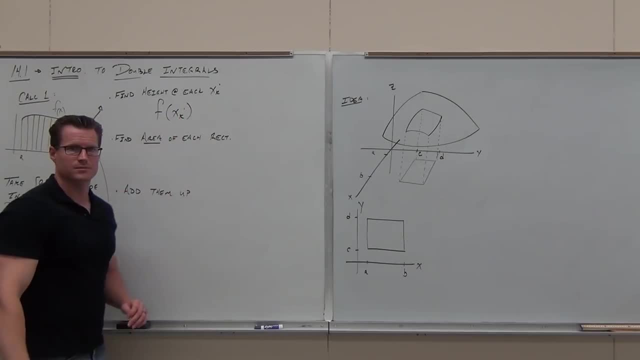 subintervals and I want to find the height at each of those points. I'm going to find the height at each of those points. Does that make sense? Now, some of you guys are learning Calc 1 for the first time because it's never shown to you What. 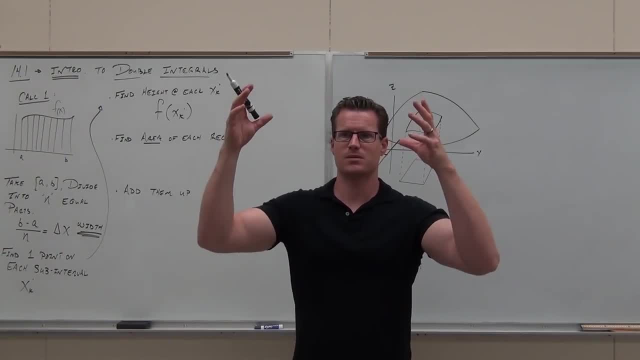 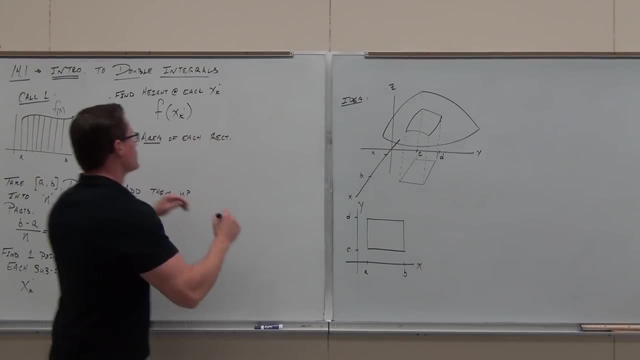 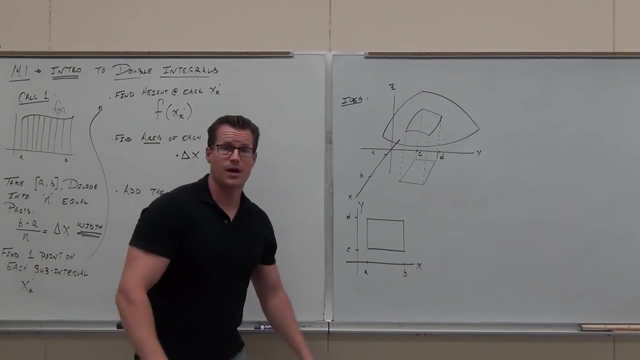 Subtitles by the Amaraorg community. Subtitles by the Amaraorg community. Area is width times height. What's the width for each of those subintervals? That's what we call them. They're all equal. So if area is width times height, I now have the width for each one. 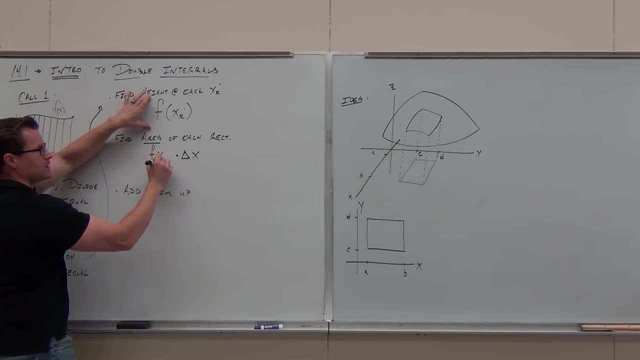 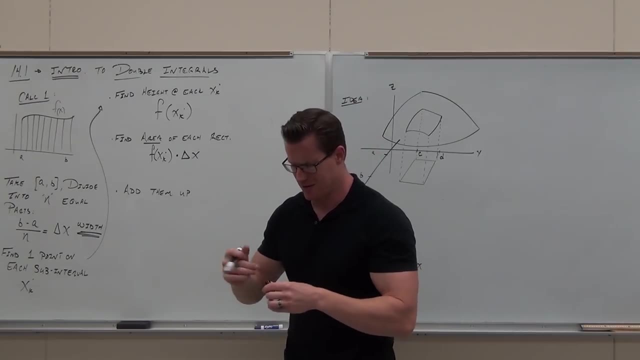 They're all the same. I now have the height for each of those rectangles. Does that make sense to you? If you need the rundown again, here it is. Each of these little subintervals is delta xy. Every height can be found this way. 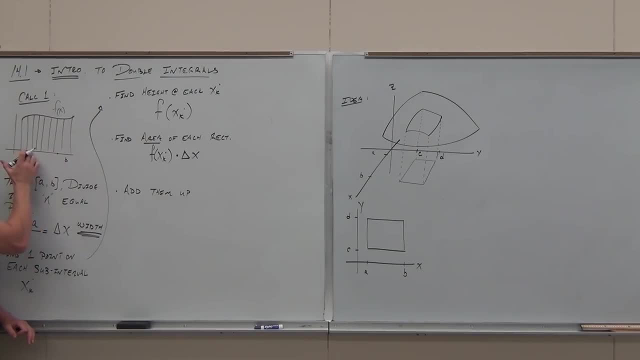 Pick an x sub k. x sub 1,, 2,, 3,, 4,, 5,, 6, x sub 7 dot here. x sub 8 dot. x sub 6 dot. Pick a random point in there: xk dot. 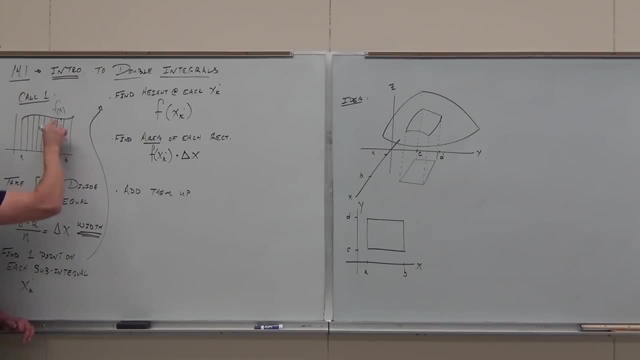 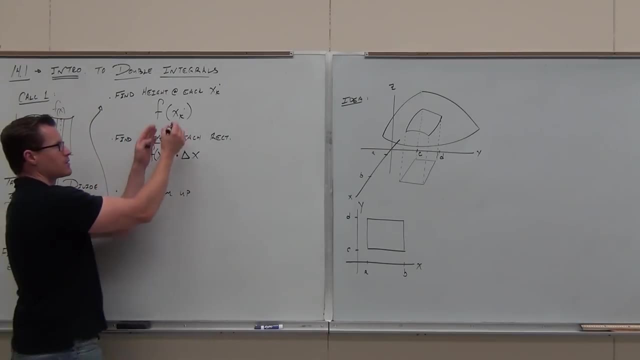 Find the height Basically just plug it in and then use that height as the height for the rectangle. Okay, so I have Width times height. Here's the height of each rectangle. We're picking that to be the rectangle Times the width. 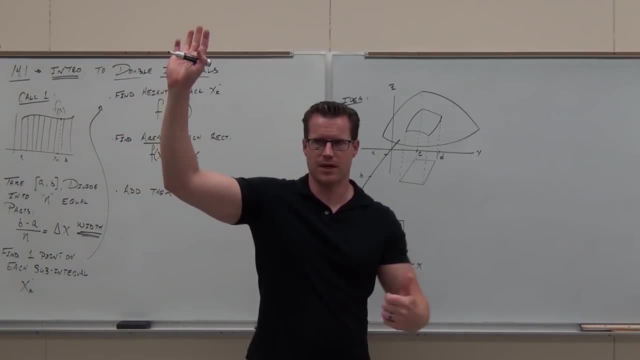 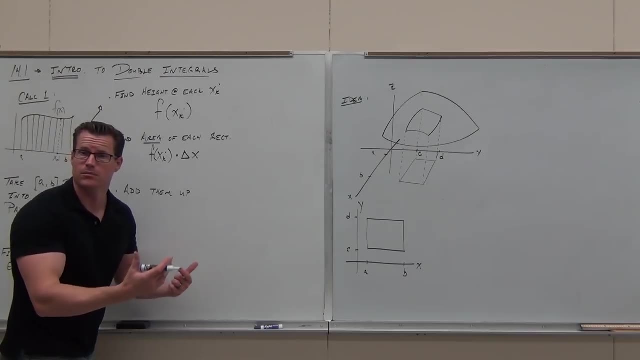 That's the area of each rectangle, so it makes me feel okay with that one. That's it. Now add them all up. How many are there? N of them. There's n of them, N different segments. That's how we found delta x. 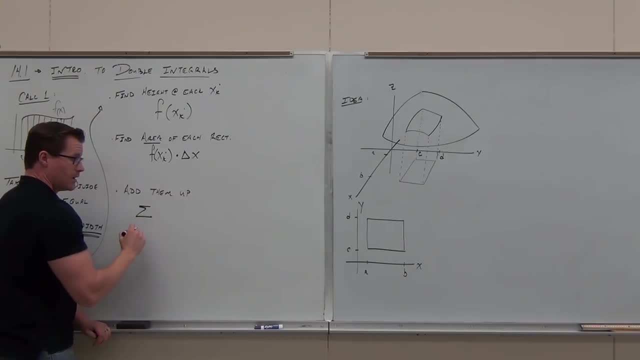 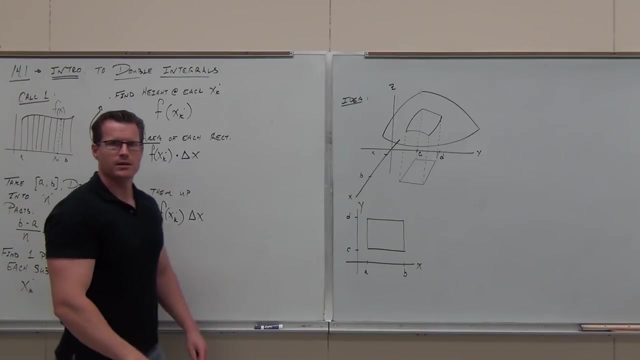 N different heights. Add them all up, From k goes from the first one to the nth one, wherever you saw it. Add up what Well. add up every single height times width, every single area. Now, here's the perfect thing about this. 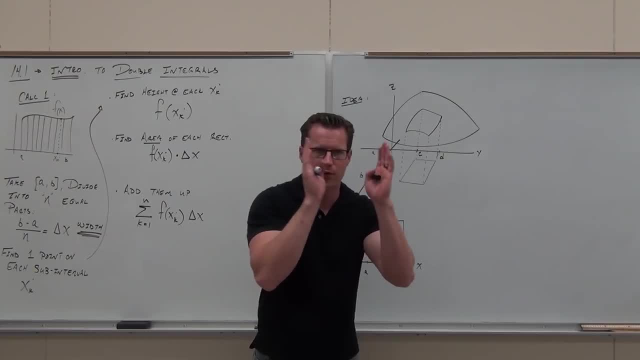 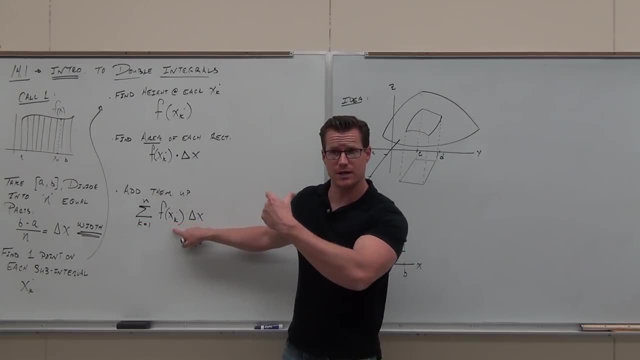 Because we're adding the same width over and over, and over and over again. you can factor it out Basically. this works this way: Add up all the heights. You've factored out the delta x, you've factored out the width. 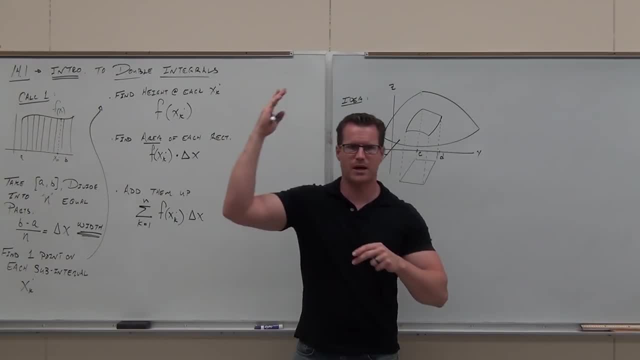 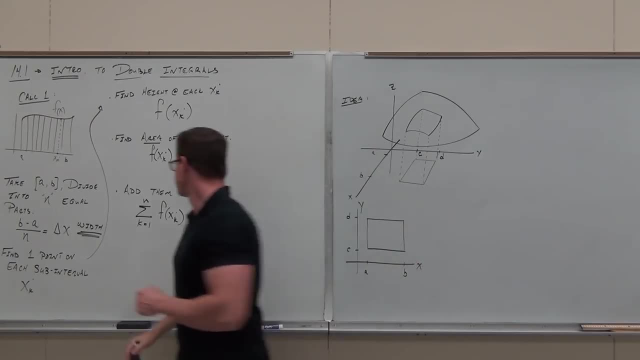 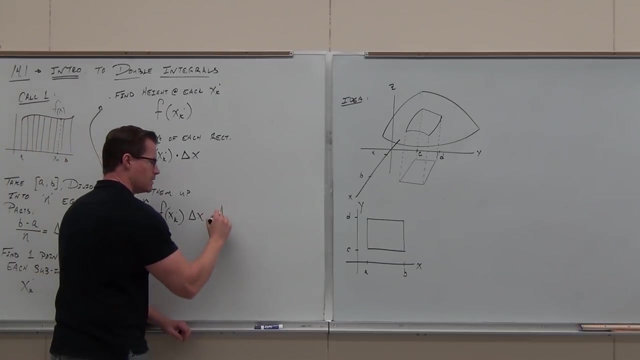 Add up all the heights, figure out that sum, multiply by the width, And it's effectively the same thing as adding all the areas. So it makes me feel okay with that one. Now, this is for sure, if I can spell it, an approximation. 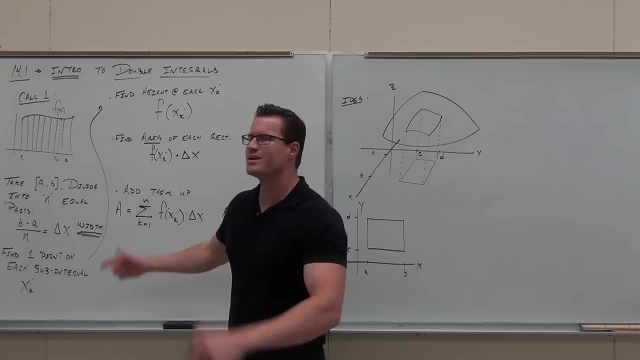 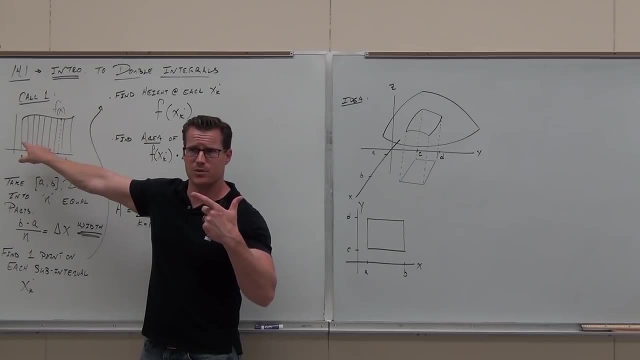 You see, it depends. It says: how good is this approximation? Well, you can see, it's an approximation. Think about it. If I do this, If I do this, If I divide this into a finite finite, here's a key word: a finite number of segments, subintervals, finite numbers. 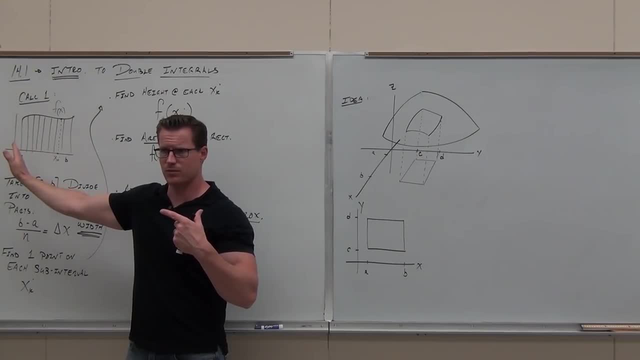 And I choose a random point in there for every subinterval And I find the height at every random point on every subinterval And I find the area. by multiplying the width times the height get an area. Is there going to be error? 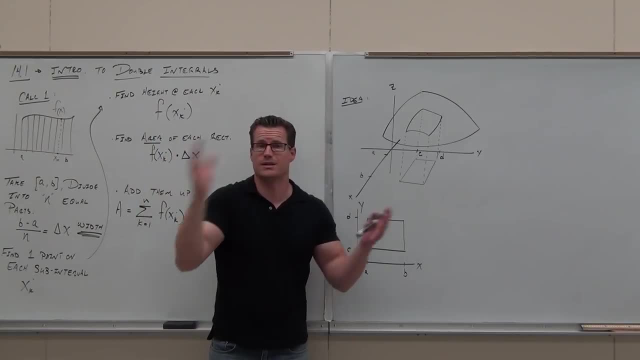 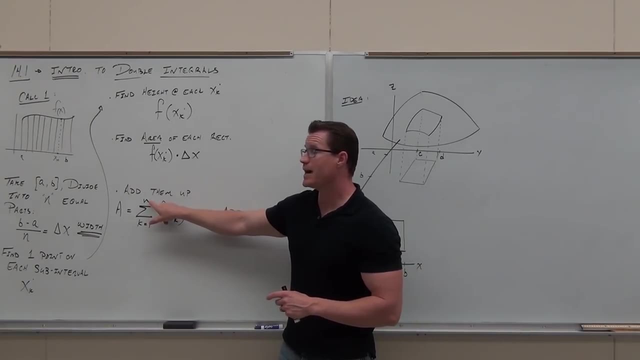 Yes, because this rectangle doesn't model perfectly the curve. It doesn't work that way. So how do I make it better? If this is, if this is an approximation, because I have a finite number of ends, how do I make it better? 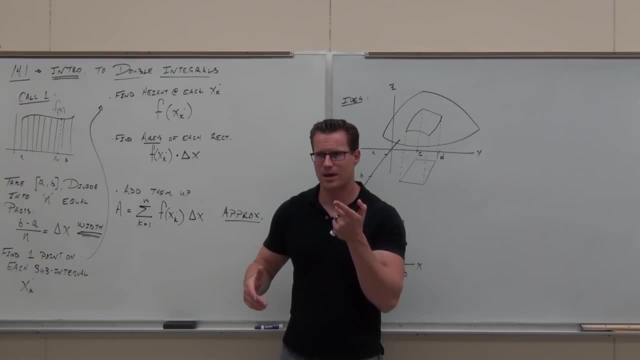 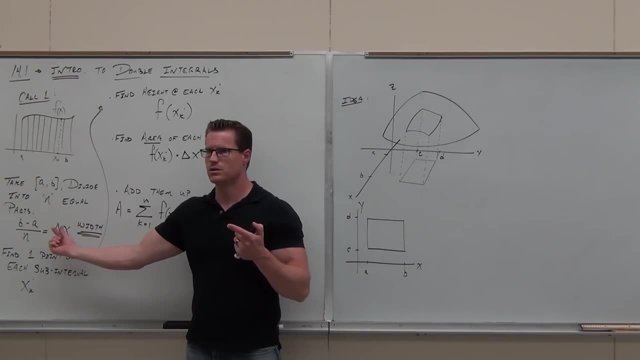 I need an infinite number of ends. Does that make sense? How do I let this be an infinite number of ends? Kind of think backwards here. I need to let the width go to really little. If I let the width go to really little, there's an infinite number of ends in there. 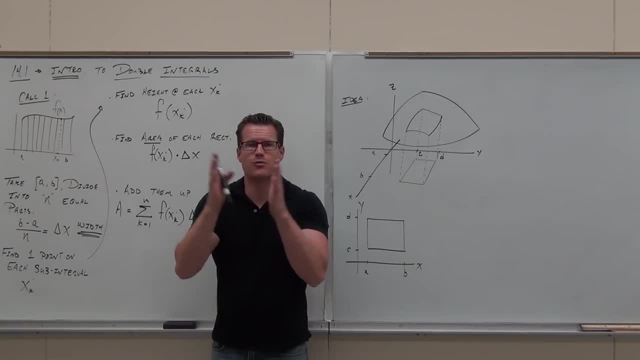 Does that make sense? Now we're just going to put Let n go to infinity. Let the number of rectangles go to infinity. That packs in a whole bunch of rectangles and makes the width of these rectangles really really close. to what number? 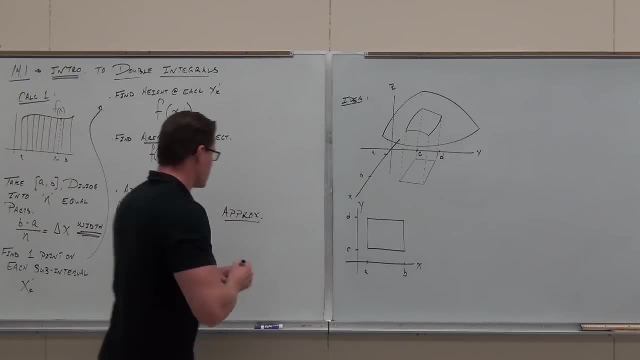 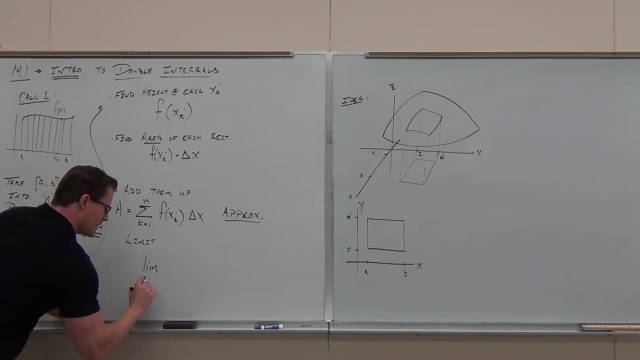 Zero, Zero, Zero, Really close to zero. So if I take a limit and say I want the rectangle, the number of rectangles, the number of subintervals, to go to infinity, And then I do that, Then notice that 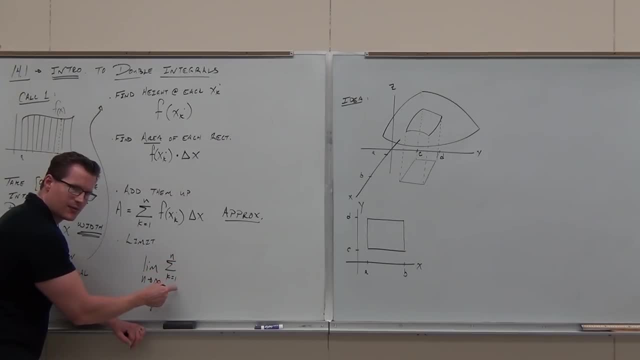 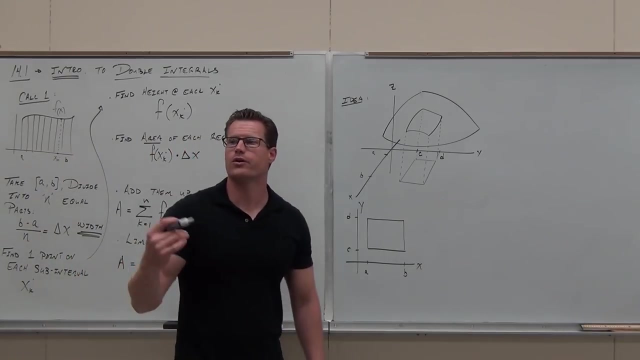 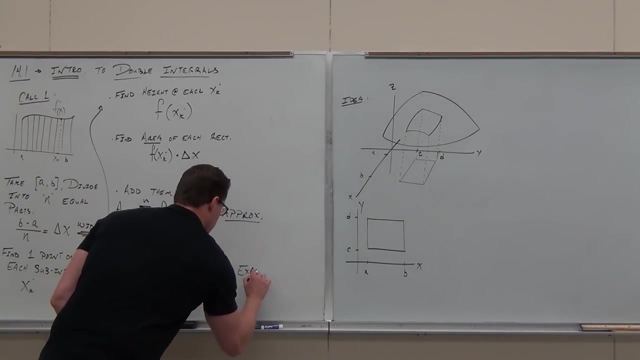 K doesn't go from one to a finite number. K adds from every rectangle to the infinite number of rectangles in that space, And what we get is no longer an approximation at all. This is exact. So long story made short. I think it took about what? 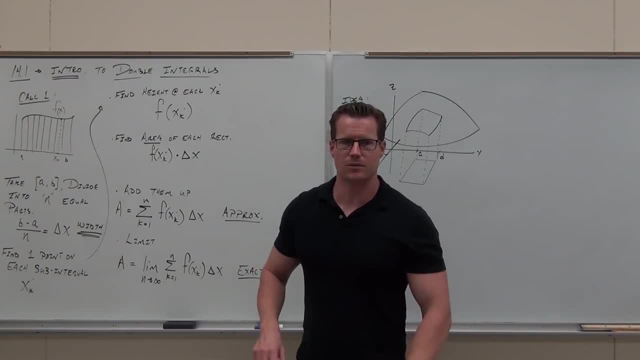 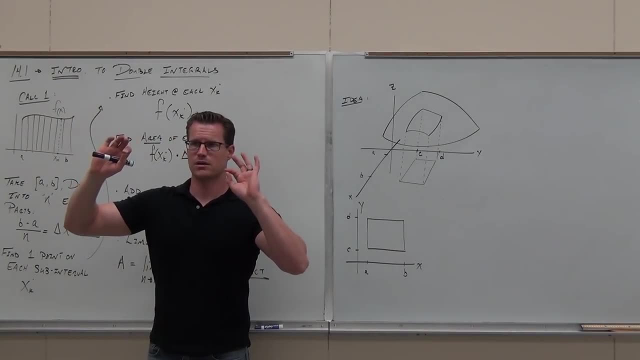 Five, Five, six minutes, hopefully. Here's a long story made short. Calc 1 does this. Calc 1 says: cut this finite area into a whole bunch of rectangles. How many? Well, ultimately infinity. All right, Cut it up into equal lengths. 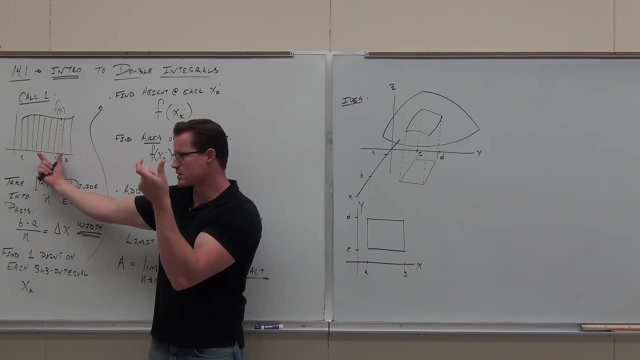 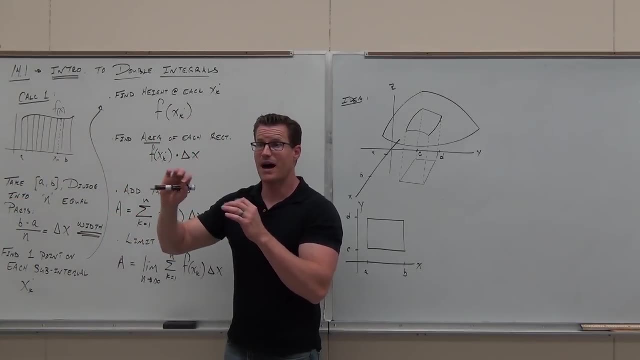 Well then, if I take b and divide it by the number of equal lengths, I get my width, delta x. Find a point on each one Cool Random point, That's the dot. Find the height of each of those rectangles. 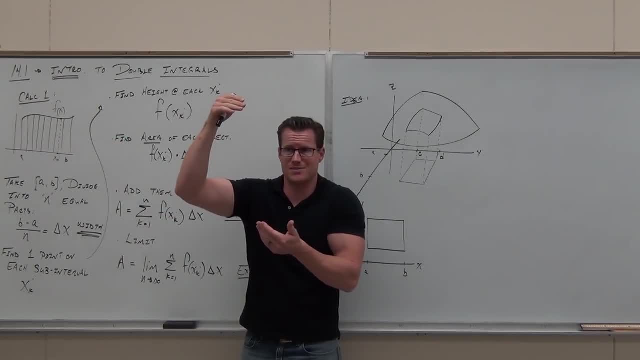 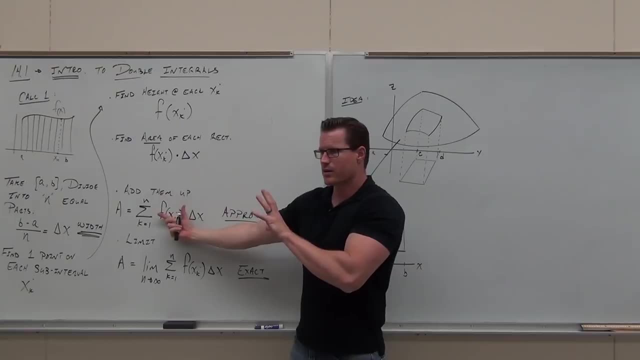 Well, just plug in xk dot and use that as the height. Does that make sense? Then we go: okay, take width times height, you get area. Add up all the areas, No problem, We can do that. Now that's an approximation, because I have a finite number of them. 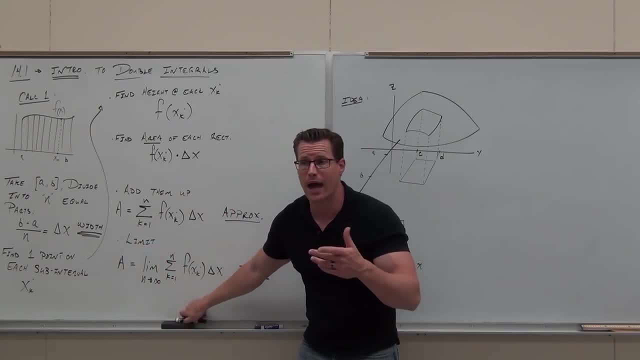 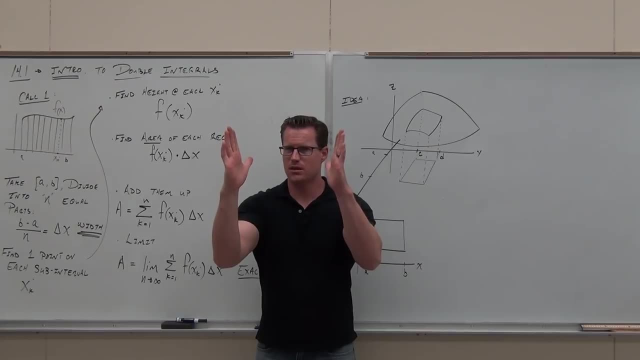 Let it go to infinity. Now, there's not a finite number. Now what happens is there's infinite rectangles in there And because you chose your point randomly, it doesn't matter where it is when you take that rectangle and you start squishing it. 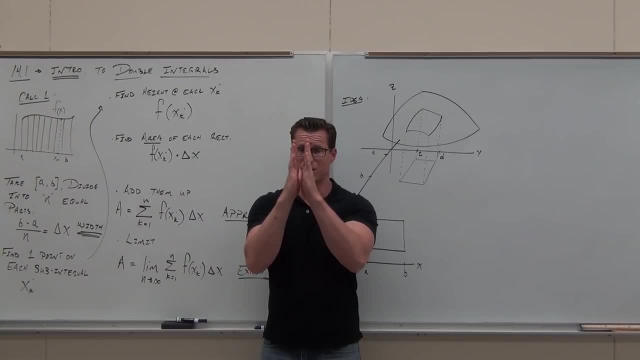 That random point starts getting squished really tight right, Really really, really close, so that it doesn't matter where you picked it, because it's going to be so close together, it doesn't matter at all. Then we get like almost these: ah, they're so close to zero, but they have a little bitty teeny. 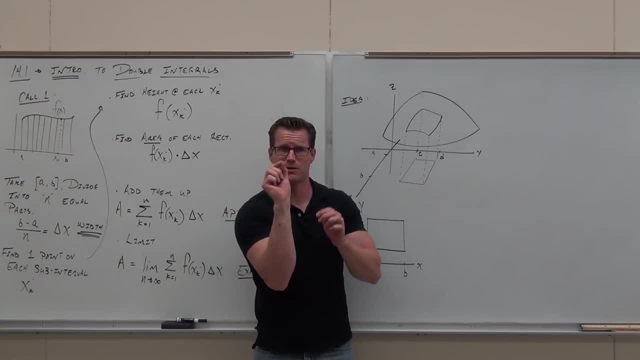 teeny, teeny, teeny, tiny width, because if you don't have width, you don't have area. So they have a little teeny bit, but it doesn't matter where that choice was. xk dot. This is exact. 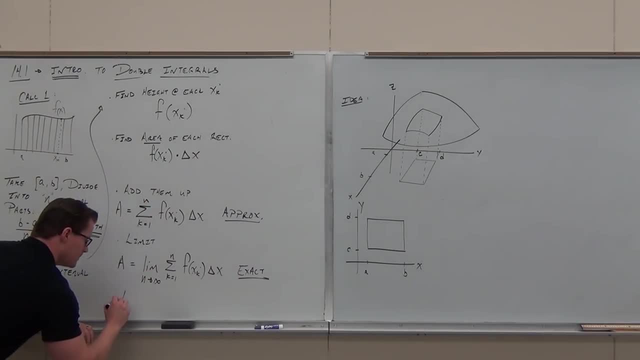 This right here is the definite. This is the definition of what an integral was. An integral is a limit of a sum. It's why we get an S. That's an integral. it's an S. It's a sum. an infinite sum is an integral. 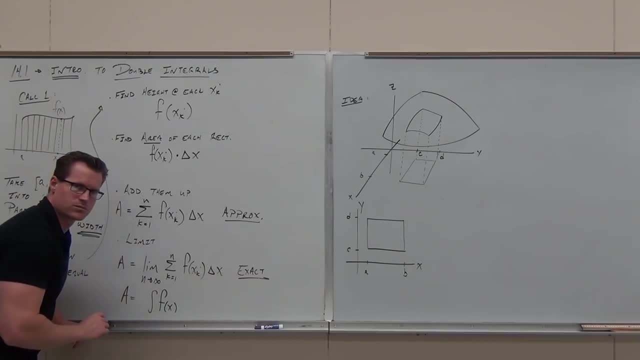 Of what A function, with x as the variable chosen at random, but it doesn't matter, it's anywhere along the x axis. Anytime we let a dx approach- sorry- a delta x approach zero, we get a dx out of it. 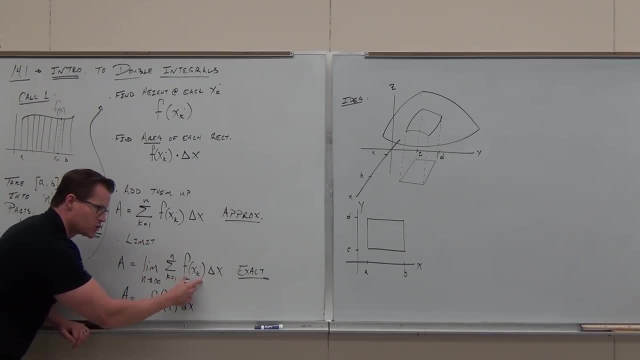 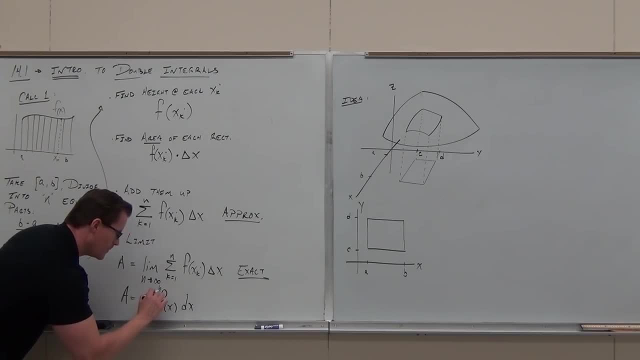 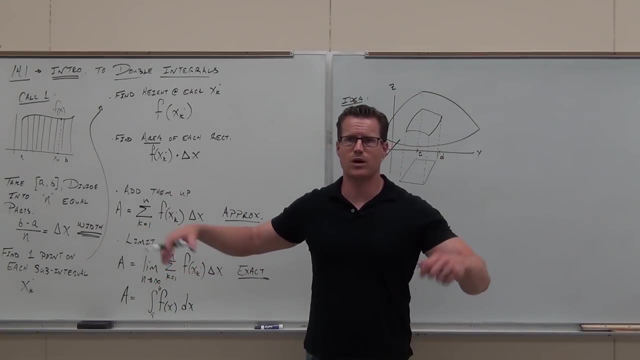 That's all of calc one, in a nutshell, for areas, And they go from b to b. That right, there is the definition of how integrals are even constructed. Did it make sense to you? Yeah, That's calc one. Now let's go to calc three. 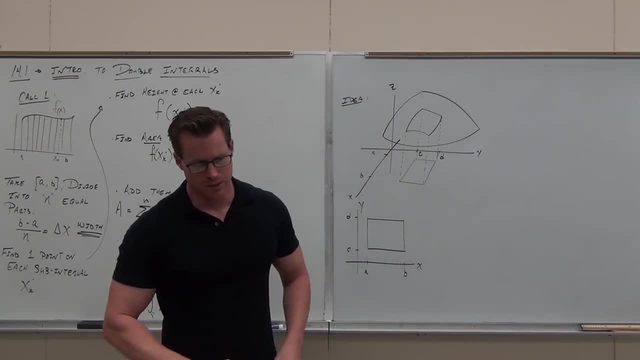 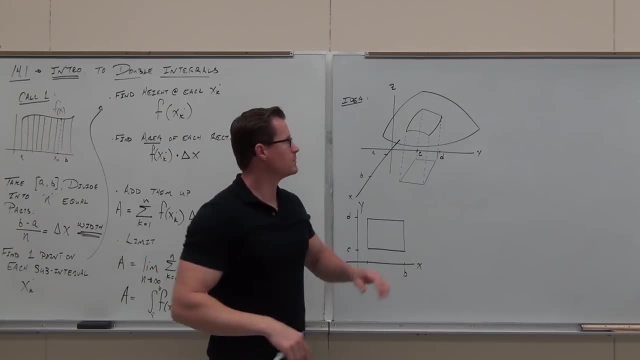 All right, What's the idea now? Well, one variable was area under a value. So if you have a curve, what's two variables going to give? you Can't be area One variable. area Two variables extends the dimensions. 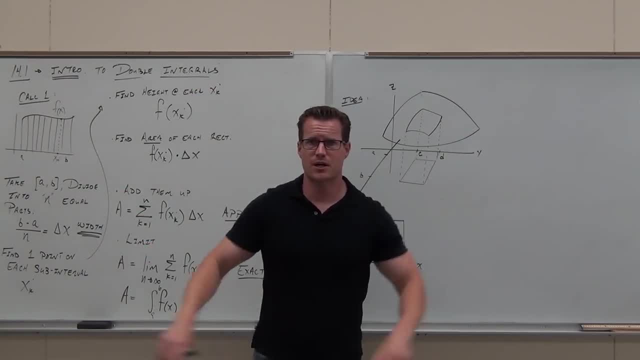 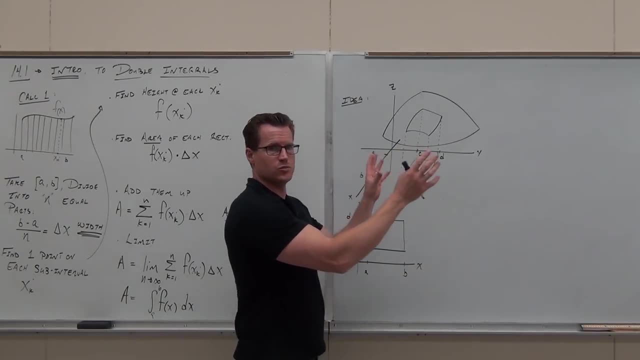 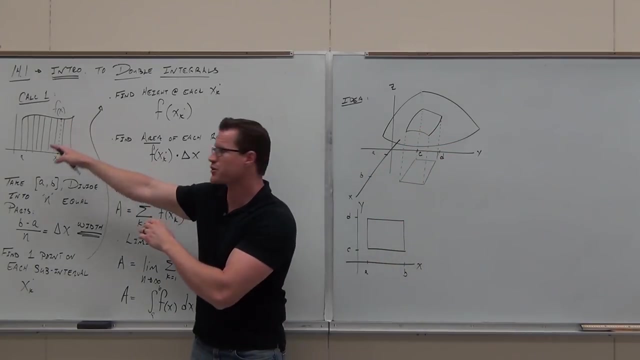 If one variable gives you curves, two variables gives you surfaces. If one variable gives you area, two variables gives you volume. Right now, the idea is find the volume. find the volume underneath the surface as bound by a region. Find the area under the curve as bound by a region. 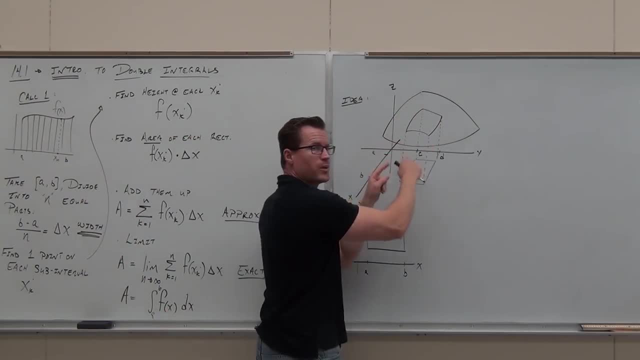 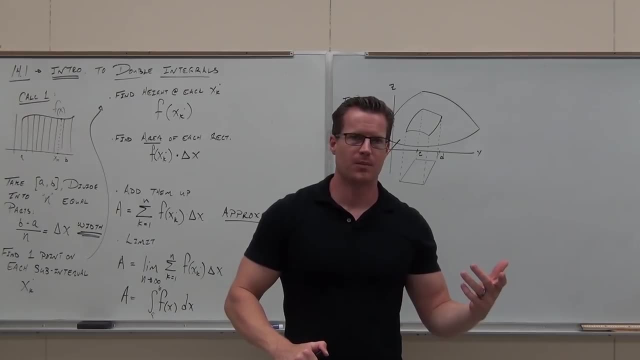 Find the area under the curve as bound by a region. Find the volume under a surface as bound by a region. You have to extend everything one dimension. Does that make sense? That's cool. That's what we're about to do. I'm going to build it for you. 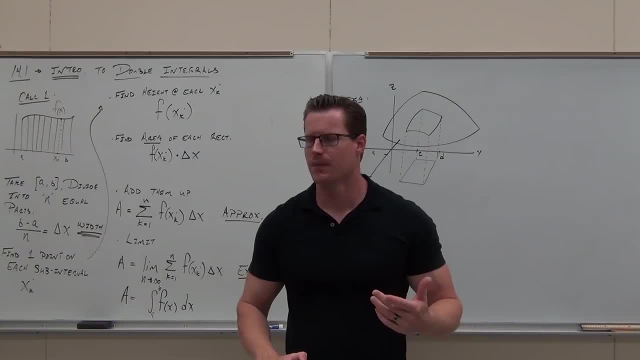 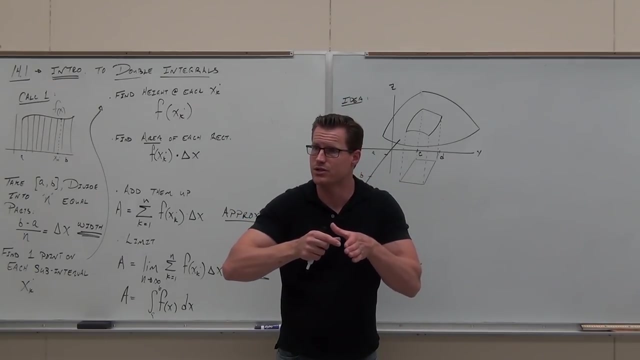 It's not hard, but you need to see it at least once to see where it comes from. okay, So here's the idea. We're not finding height and multiplying by width anymore, because that ain't going to give us volume. We're finding height and multiplying by area, the surface area of every little region down there. 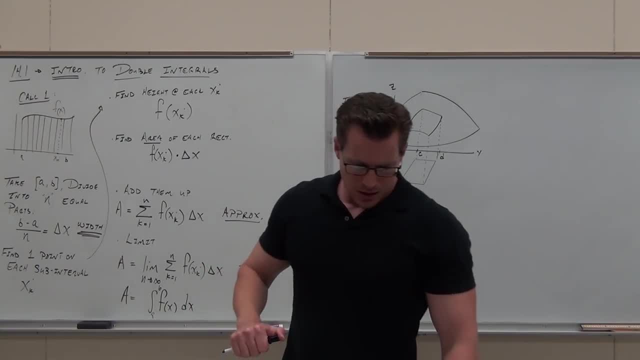 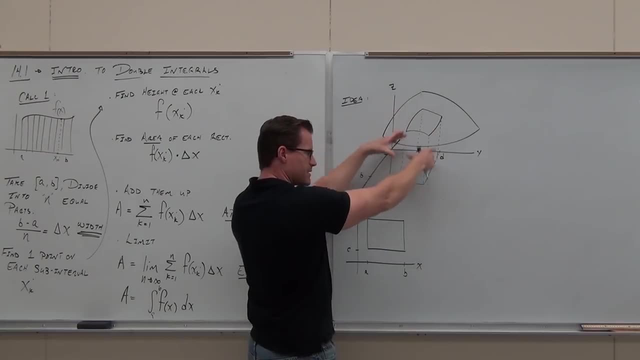 That's what we're going to do. That's what we're going to be doing now, So I'll build it for you. Let's take the region under some surface. So here's my surface. I cut a little region and I'm going to set this down here. 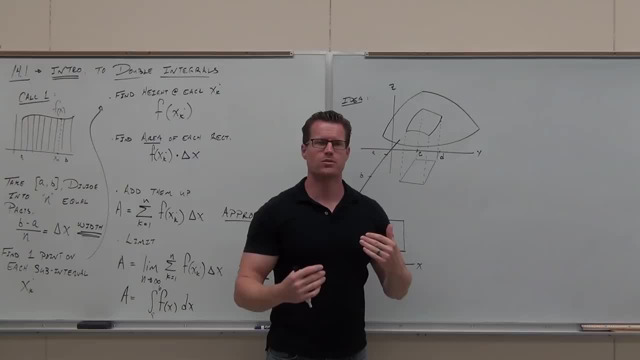 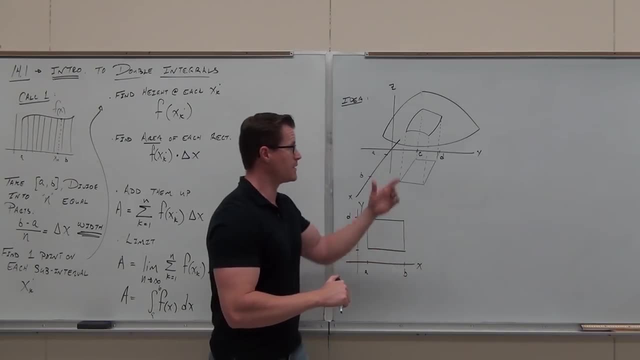 And right now? for right now I'm just dealing with rectangular regions. to make our lives easy, I'll show you how to deal with non-rectangular at the very end. Right now we're just dealing with some rectangular regions. Can you see that on the xy plane I'm going to have a rectangular region? 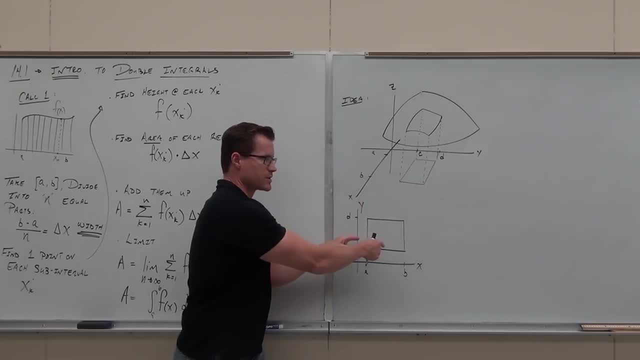 Yeah, there we go. Yes, There we go. Yes, That's what this is. So x goes from a to b, x goes from a to b, y goes from c to d, y goes from c to d. Are you guys with me? 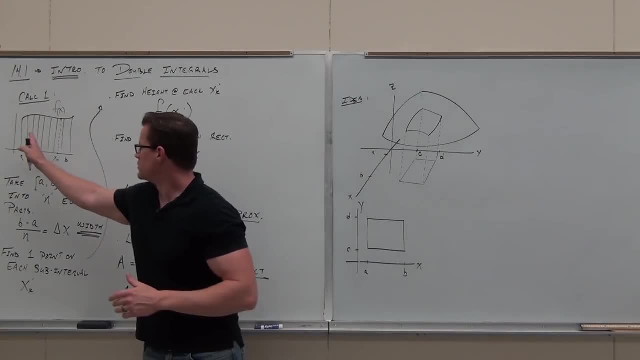 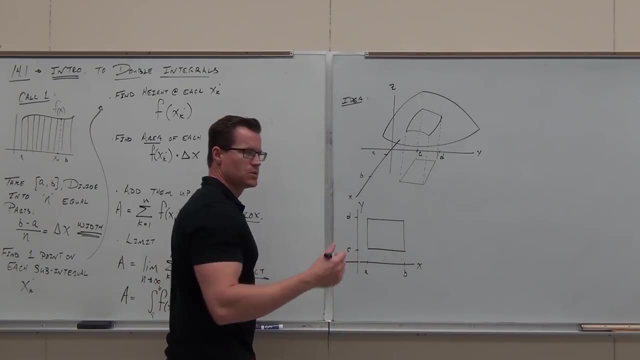 Now, instead of segmenting this just along the x, I now have to segment this just along the y, So I'm just going to choose this: to cut this twice and cut this once. It doesn't matter. The more cuttings, obviously, the more accurate. 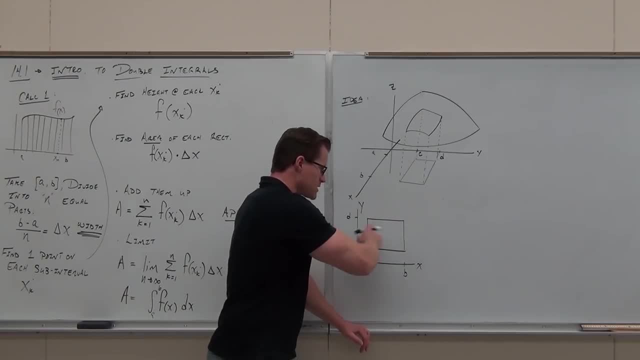 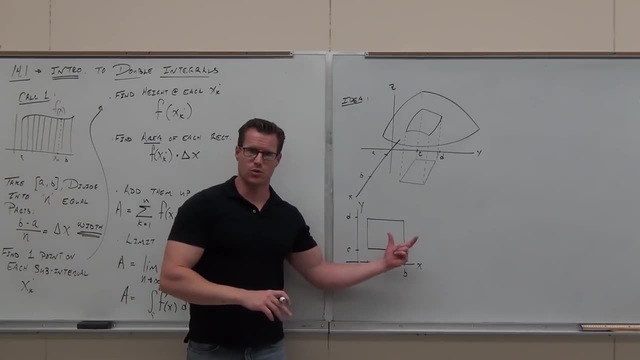 But just to give you a picture of this, I'm going to cut this into two segments: One segment here and one segment here. And the key is? the key is: just like I wanted equal subintervals here, I need equal rectangles here. 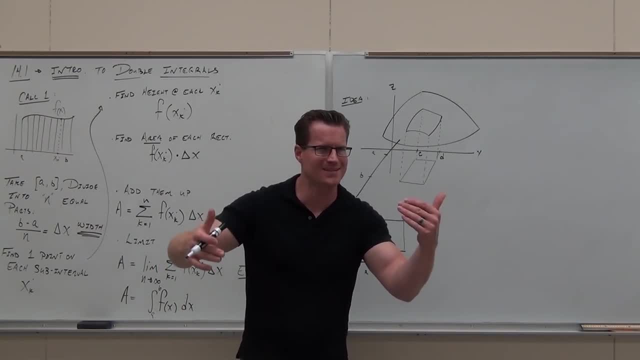 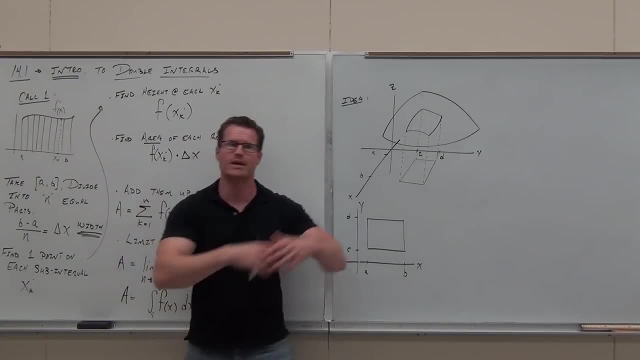 Do you guys see that the extension of the dimension, just like Calc 1 to Calc 3 does, Instead of just having length, now I have length times width, Instead of just having a distance, here, now I have an area. Instead of just getting area, now I get a volume. 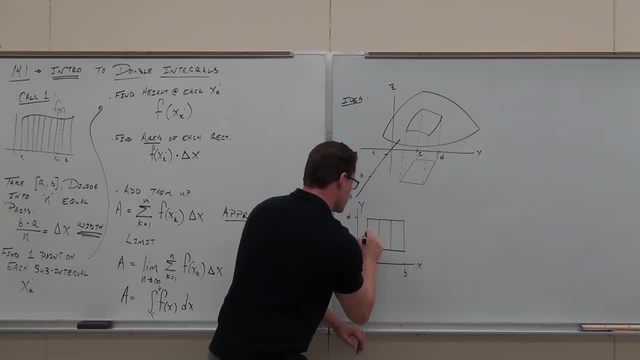 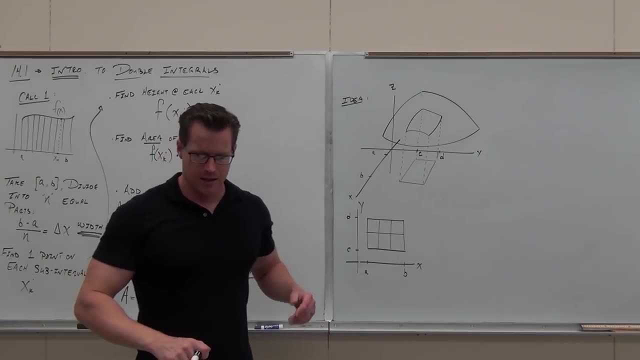 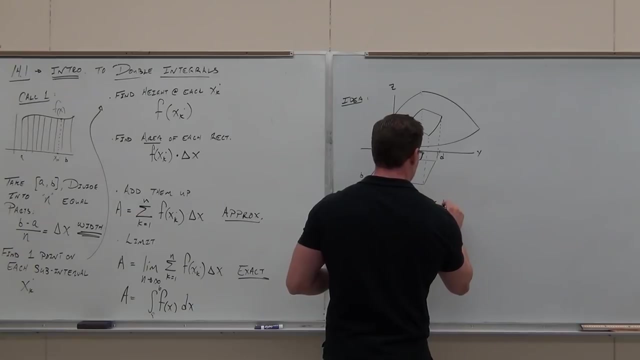 So I'm going to cut this here and here. So we're going to take that rectangular region and we're going to cut it. But the key is I need the rectangles to be equal size, Equal, equal, double, equal. sorry, 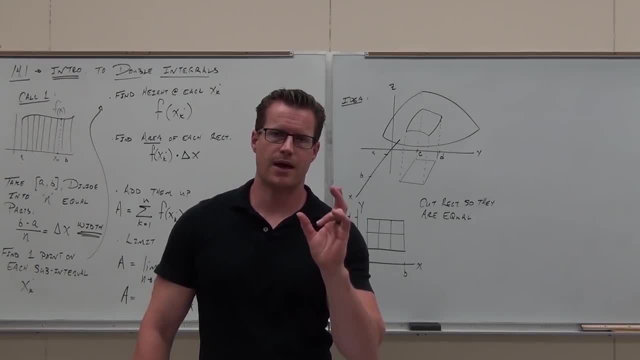 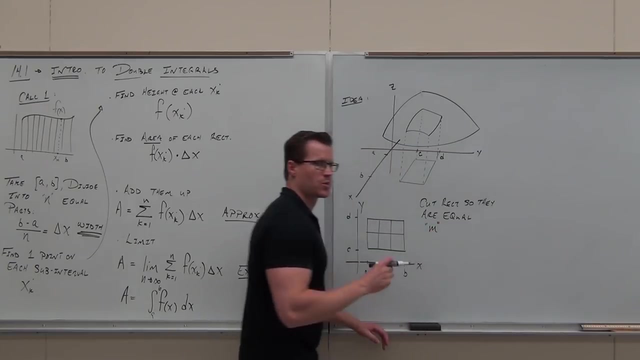 The number of partitions that you cut the x out of the number of partitions that you cut the y axis in is m. The number of partitions you cut the y axis in is n. So in this so m represents the number of partitions along the x. 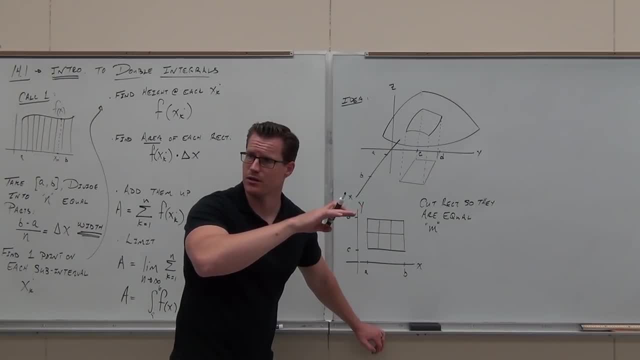 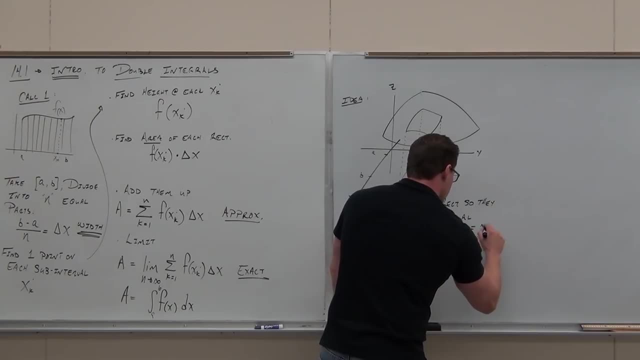 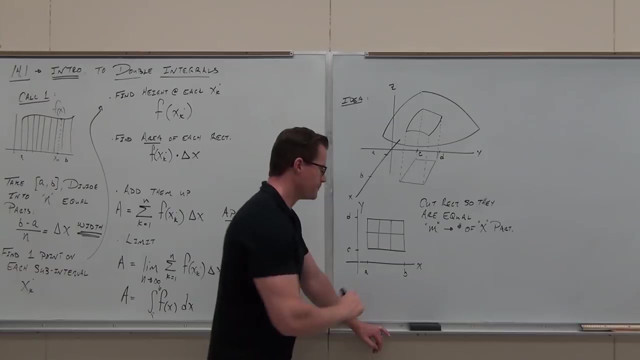 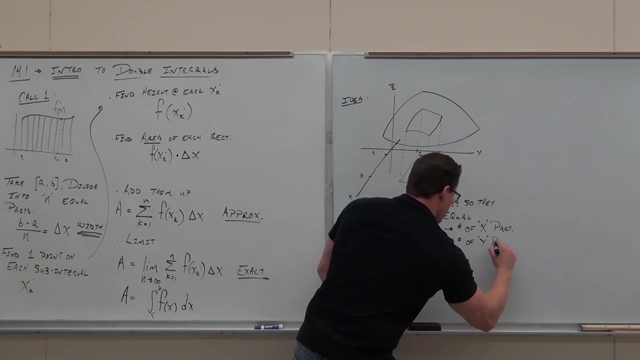 N. number of partitions along the y. Are you guys okay with the terminology there? Notice, all the rectangles are equal. That's what we want here. Number of x partitions- I'm abbreviating Y. number of, I'm sorry. n number of y partitions. 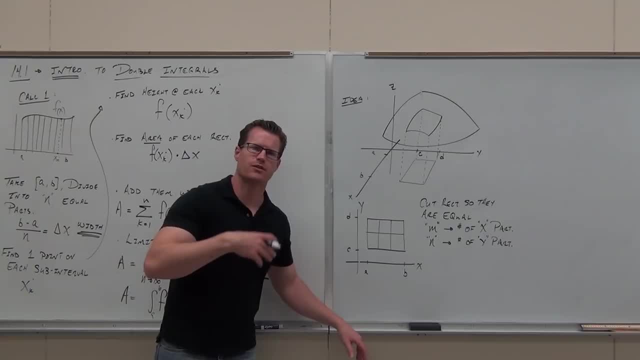 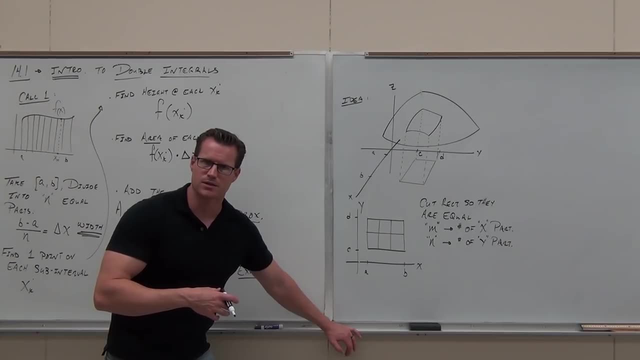 Everybody in the room right now, please. how many? what is our n? What's our value of n here? Is it 3 or is it 2?? It goes along the x axis. How many? what is our m? In this case, everybody in class right now. it goes along the x axis. 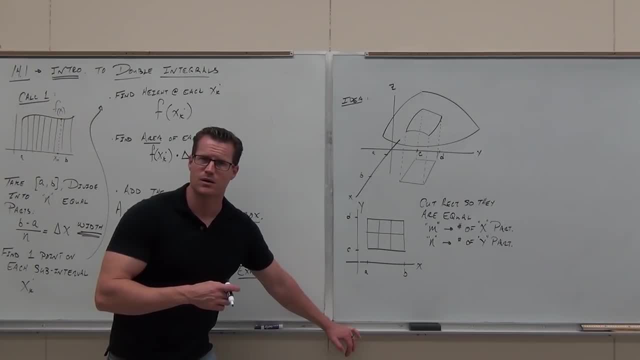 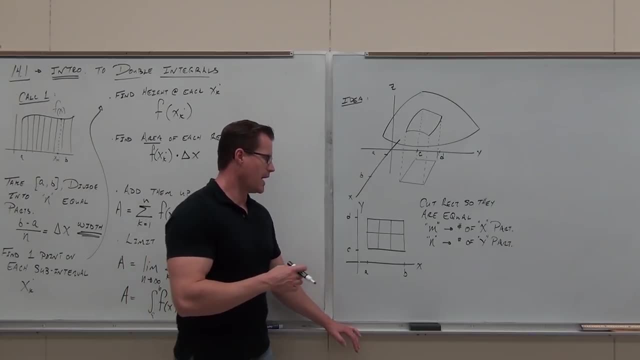 And the x axis, m is along the x. What's our value of m? Still not making sense. Okay, so how many? so here's our interval from a to b. How many times, how many partitions do I have from here to here? looking up: 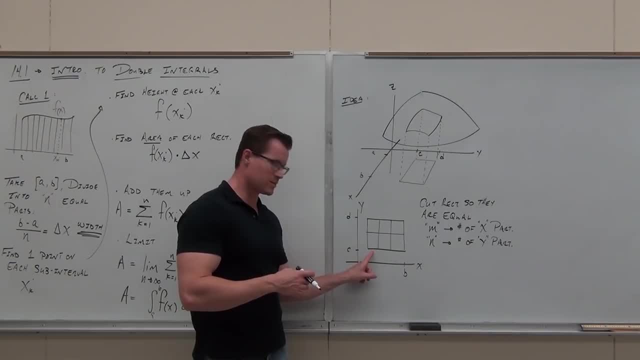 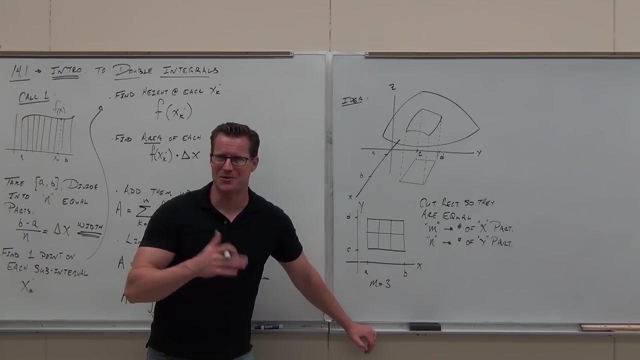 How many do I have? Let's count them. Here's one, Here's two, Here's three. M is three, M is three. We have three partitions going along the x. Now let's do the y. How many partitions do we have going along the y? 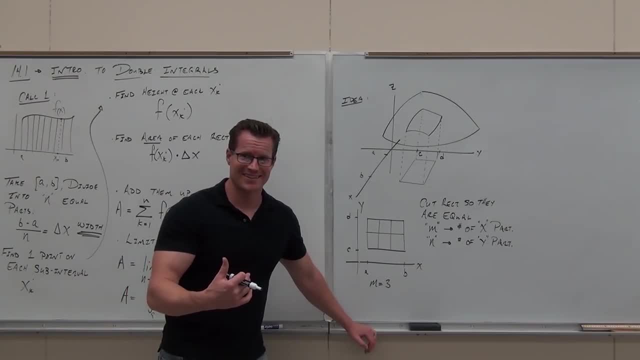 Two, Perfect, So your n is Two. Wait, is it m? Three, N, N, The m, the m? the m is three, The N is: Yeah, that's right, that's right. So it has to be okay with that one. 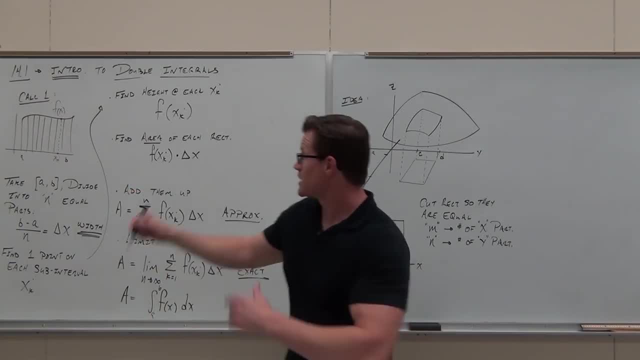 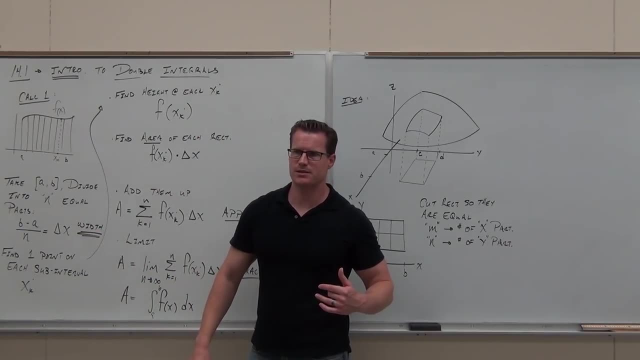 That's the idea Now. now, just like here, we picked a point- not really a point, though an X value. You can't pick a point along the X axis. You pick an X value along the X axis. You pick an X value for every single subinterval. 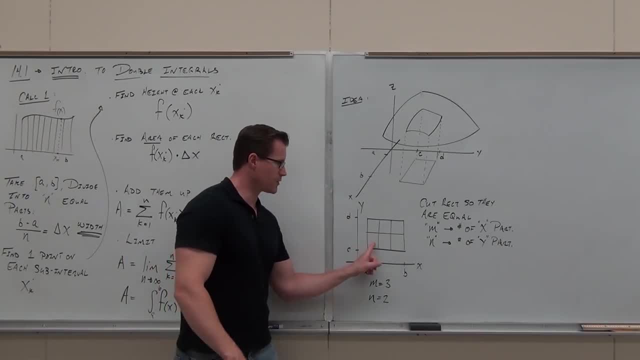 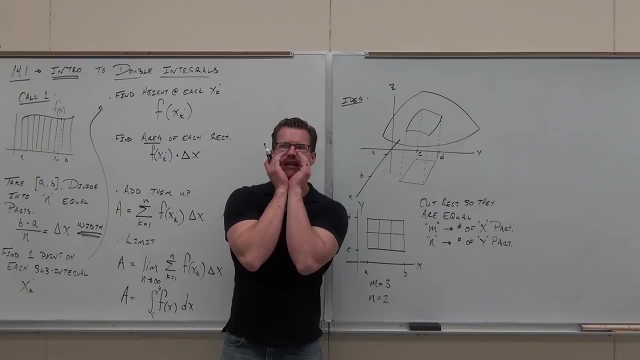 Here. we're going to pick a point for every subrectangle. Do you guys get it? We're going to pick a point on every one of these. How many points are we going to pick for this specific example? How many rectangles do we have? 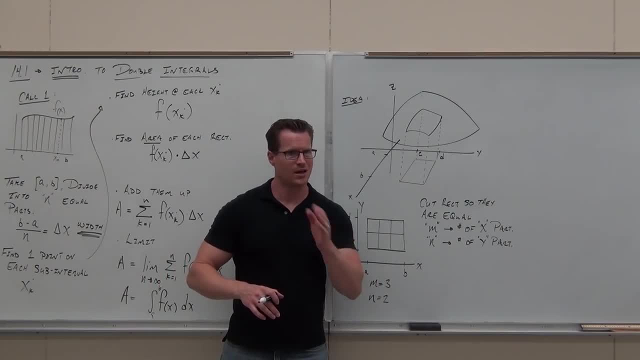 You're always going to have M times N rectangles, Do you see it? You cut the X into M and you cut the Y into N M times. M gives you the number of M times N. my M and M's are off, okay. 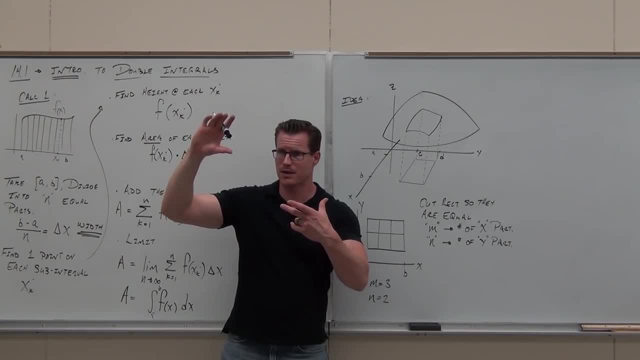 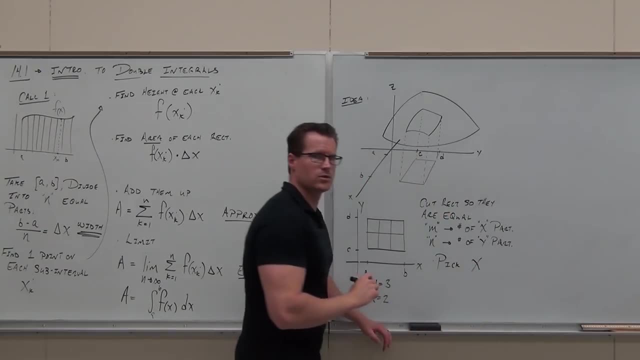 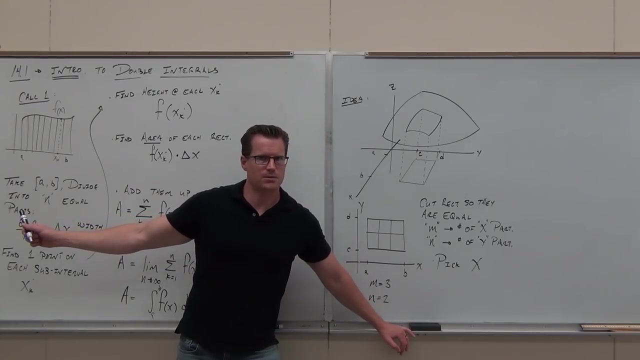 My M times N gives you the number of rectangles You're going to have to pick a point for every one of those. This is going to look like this. This is going to look crazy to you, but watch carefully. Instead of XK. well, now we need to be able to do this. 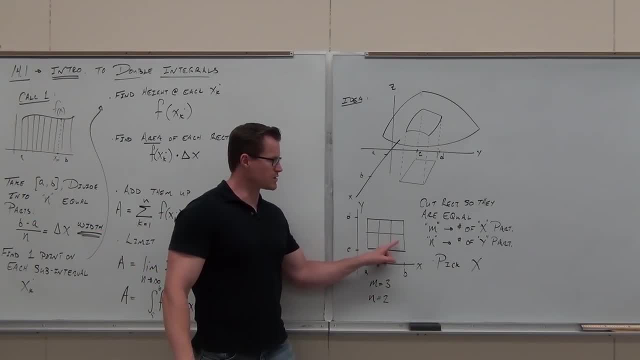 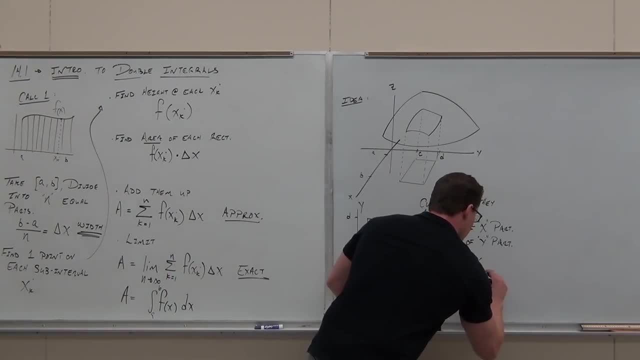 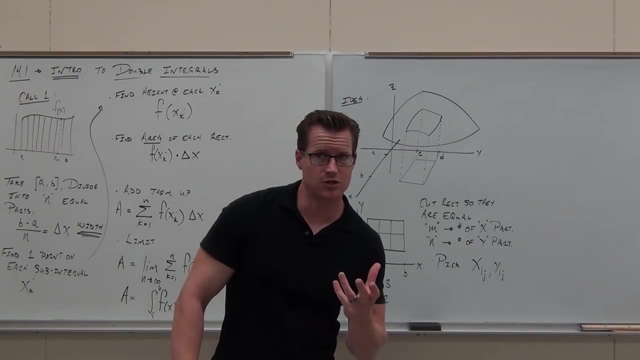 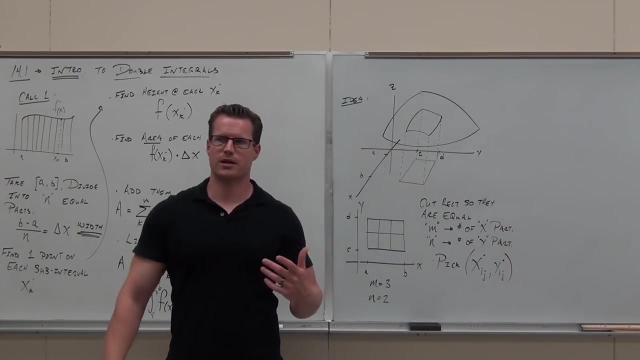 So we need X sub IJ, Y sub IJ. We're going to do right here. so if you'd look at theклад in this section here, if you would Y sub IJ dot, because they've got to be able to be arbitrary. 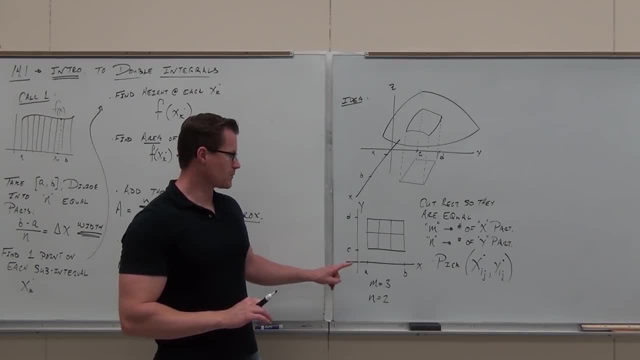 Here's what this means, because it looks really weird. but here's what this means. You would do X1,1, sorry, X- coordinate of the first rectangle along the X and along the Y and Y, of the first rectangle on the X and Y. 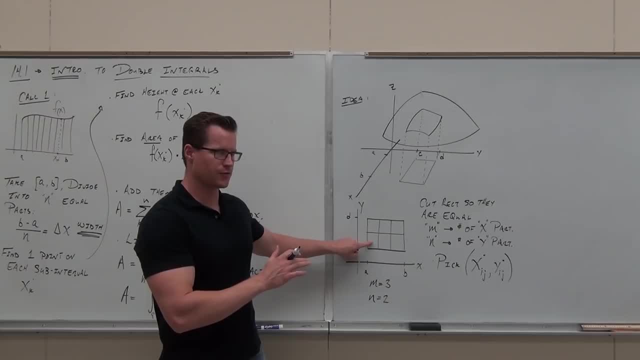 So you count up all of them. So we have X sub IJ. So we're going to do X sub IJ. We're going to do Y- Hello everyone. So we're going to do Y sub IJ. 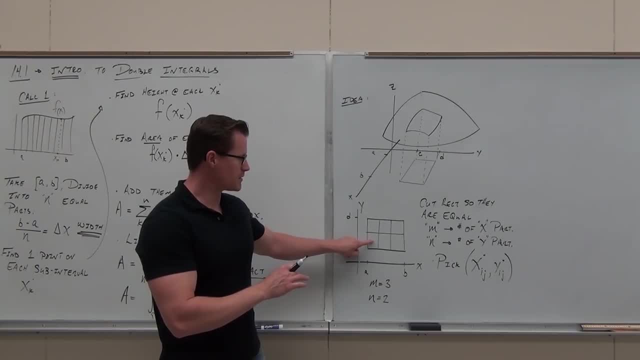 We're going to do Y sub IJ. count x in the first rectangle and y in the first rectangle, But then you'd go x in the first rectangle along the x and the second rectangle along the y, So this would be rectangle 1, 1.. 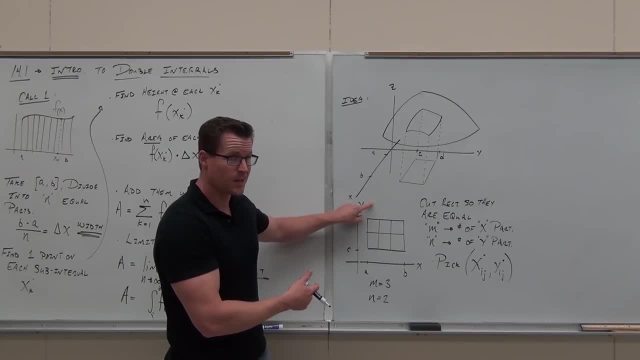 This would be rectangle 1, 2.. This would be rectangle 1, 3.. This would be rectangle 1, 4. if we had it, This would be rectangle 2, 1.. 2, 2.. 2, 3.. 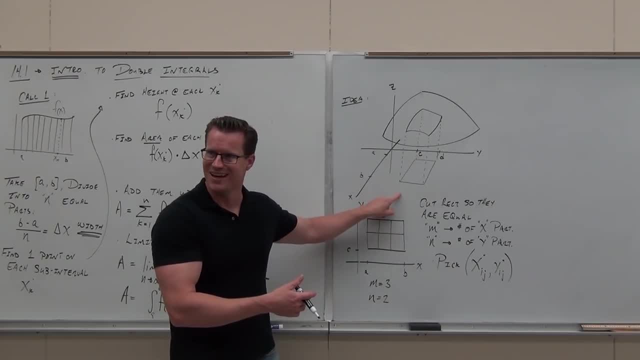 2, 4.. 3, 1., 3,, 2., 3, 3.. Do you get it? And for every rectangle: 1, 1, 1, 1, 1, 2, 1, 2,. 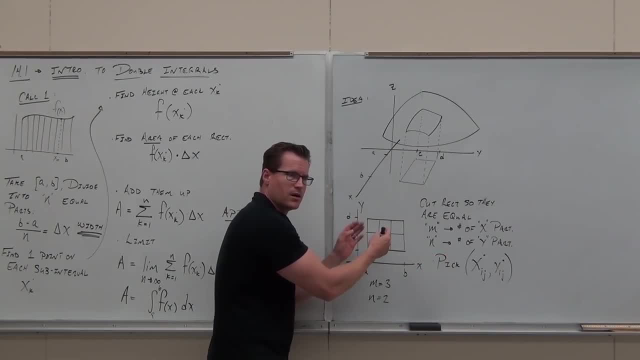 you pick a point, So somewhere in there, some x, y, in the first rectangle 1, 1.. Second rectangle 1, 2.. Yes, Can the point we pick in the rectangle be on the boundary or does it have to be? 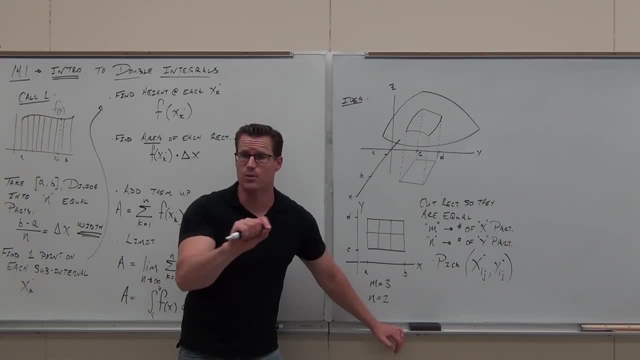 Yes, Typically we choose corner points or the center point, But it can be anywhere. The dot means we're arbitrary like this, And you can imagine if we let all these rectangles go, If all these rectangles get really, really, really little. 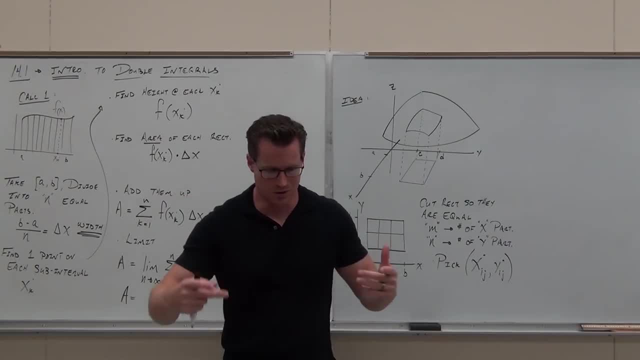 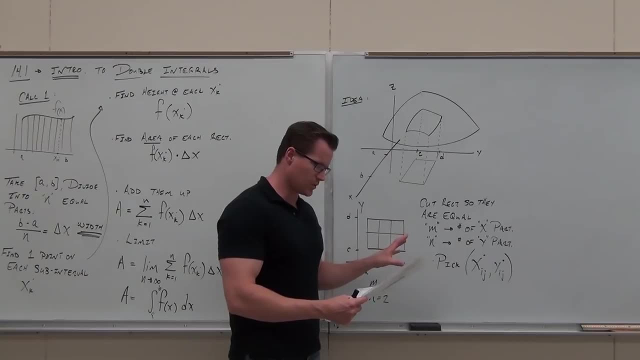 it doesn't matter if we were to pick our point. Make sense, It doesn't matter because we're going to do that. So m times n rectangle is very good. For each rectangle we find an arbitrary point. Pick a point, No problem. 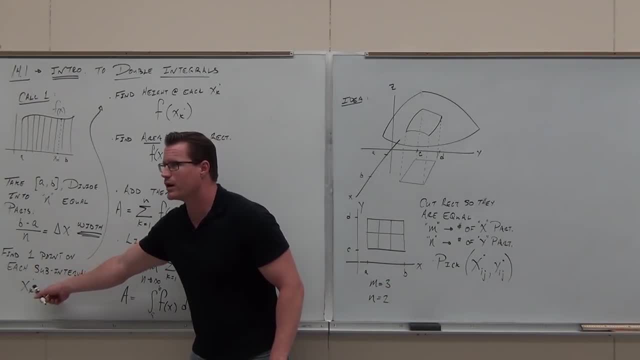 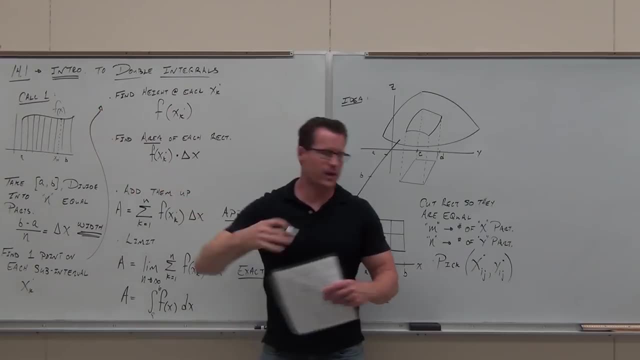 What do you suppose we're going to do now? Well, here we picked a point, And then what did we do? Come on, What did we do with the point? What did we do with the value? I should say: Plug it in to get a height. 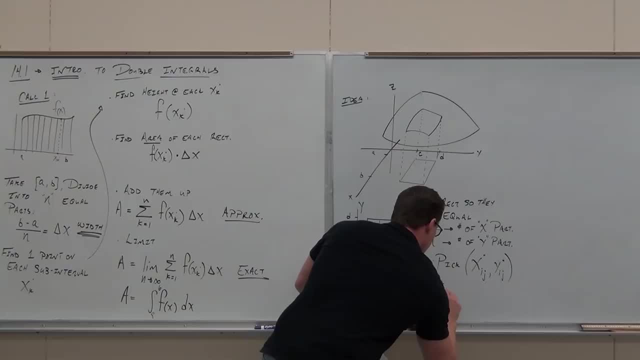 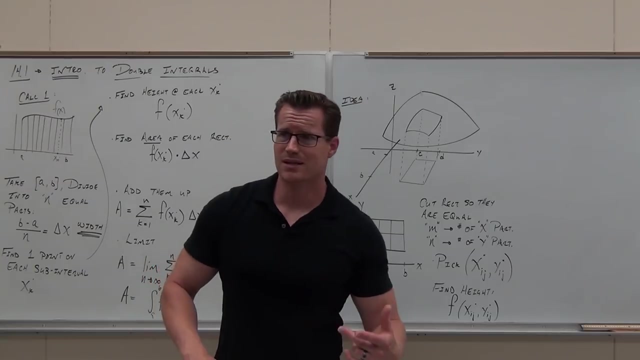 OK, so let's plug it in to get a height, Find a height. Well, that would be. functions always give heights. I know the notation's crazy because you're not used to dealing with double indices, But I do want you to be able to follow it how we're going. 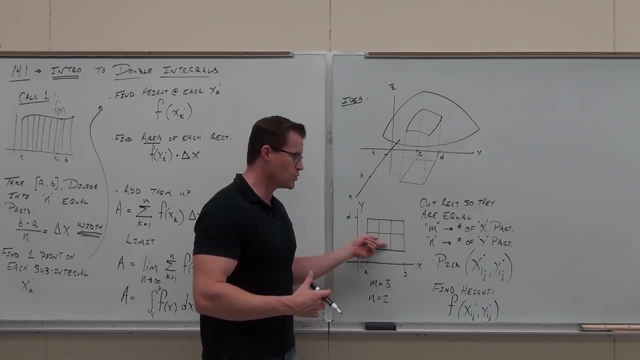 rectangle 1, 1.. Rectangle 1, 2.. Rectangle 1,. rectangle 2, 1.. Rectangle 2.. And every time we're in there, that's all that means, guys, In a given rectangle, you're picking a point. 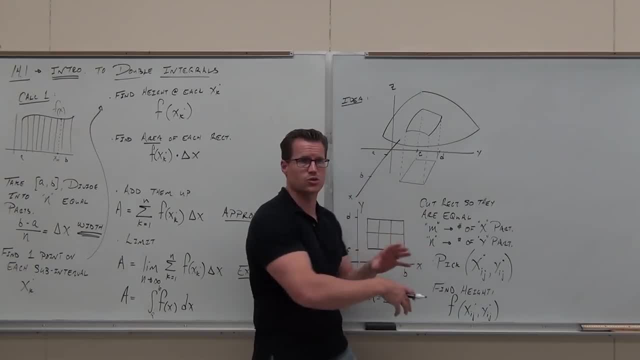 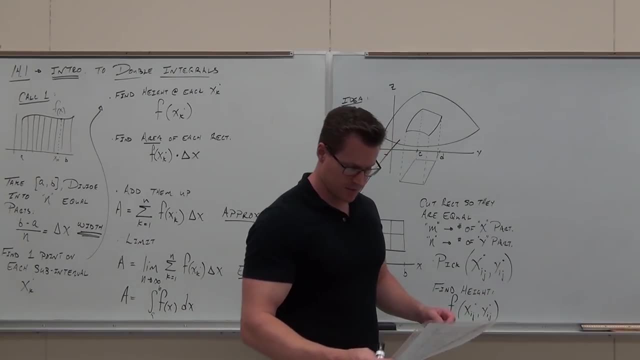 That's all I'm saying, And you've got to pick a point for all six of these rectangles or all infinity of the future rectangles. OK, Now we find a height, All right, so we get that. We typically, as was asked, where do we pick our point? 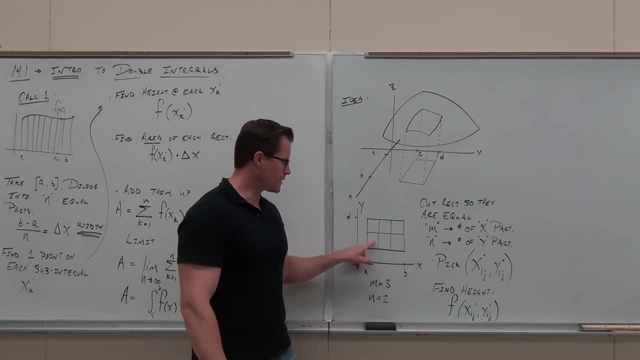 We typically choose to pick one of the corner points or the very direct dead center To make sense, To make our math easier. It's like: oh, I want you to pick that point right there. How are you going to describe that? 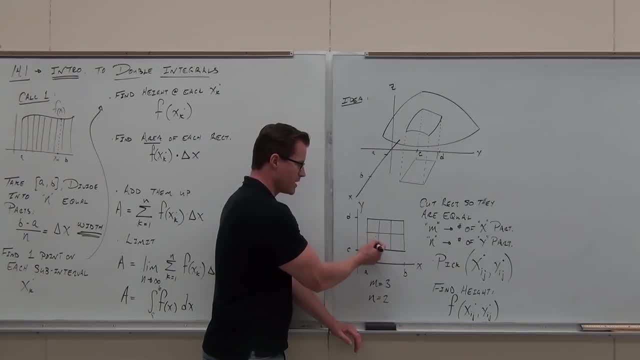 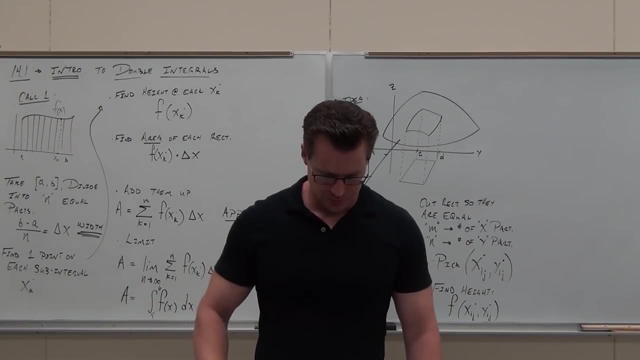 That's really hard. Here it's pretty easy to take this and divide it by 2, take this and divide it by 2 for the center. Here it's really easy if you want to pick a corner point. So we typically do that. 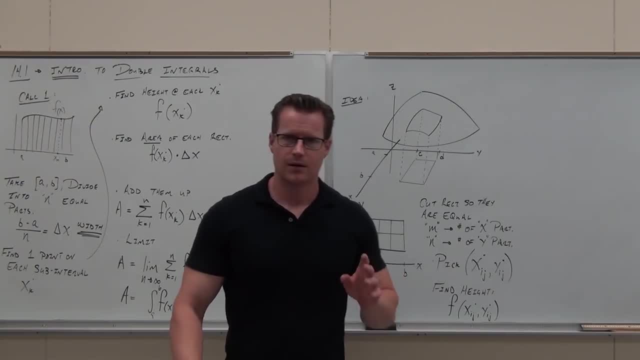 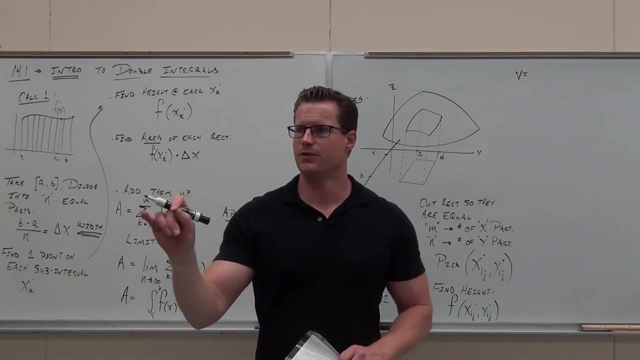 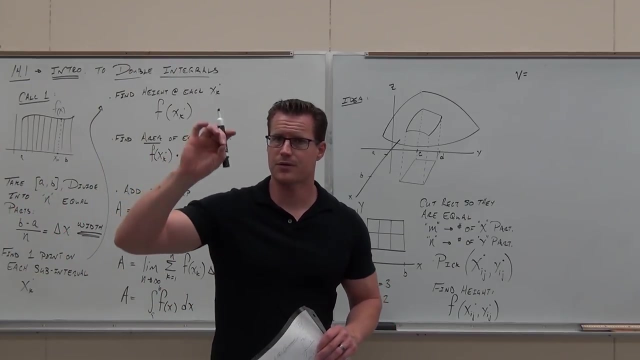 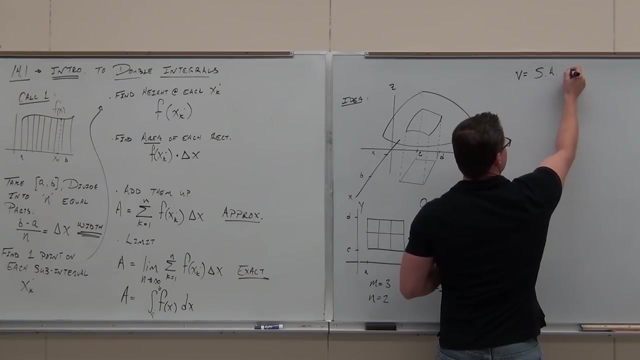 Now, finally, are we looking for area or volume, Volume? Volume Volume is the surface area of every rectangle and they're all the same times the height of each of the function at each arbitrary point. So volume equals surface area times height. 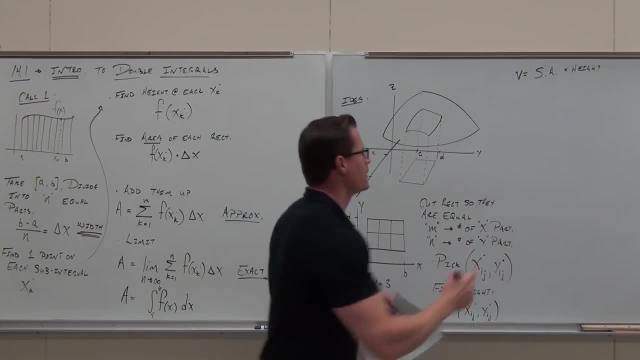 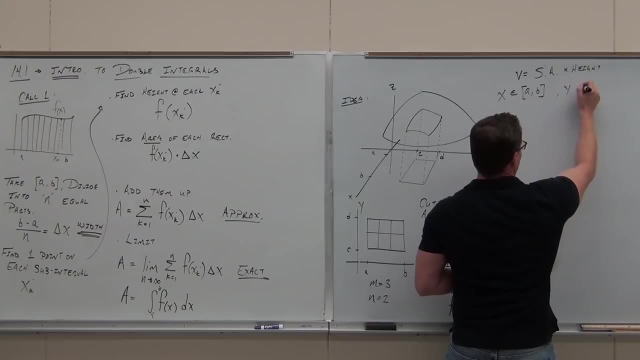 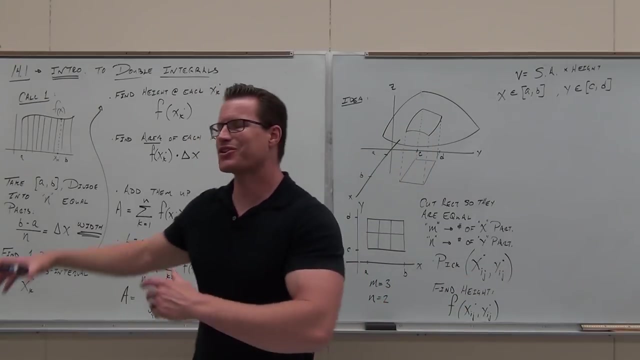 Let's work with that. Here's the math: If x is an element of on the interval AB, acting earthy for x, A, B and Y is on C, D, Let's start building this in there somewhere. So we're taking the follow me along, okay. 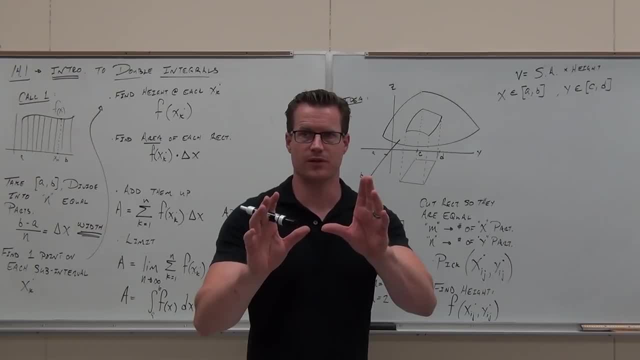 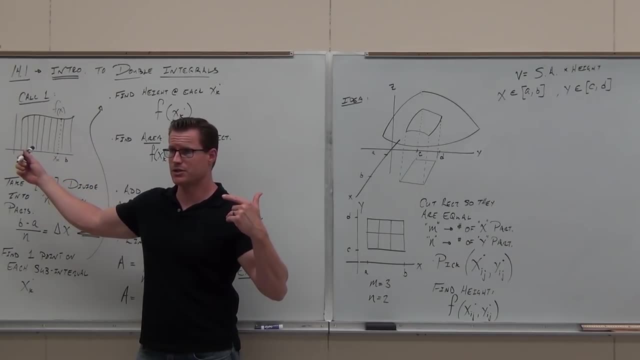 I don't want to lose you here. You've seen too much. okay, You've seen too many. You've got to learn it all now. This is just along the X axis, right? I took A to B. I cut it into N. In this case, X had N with it. 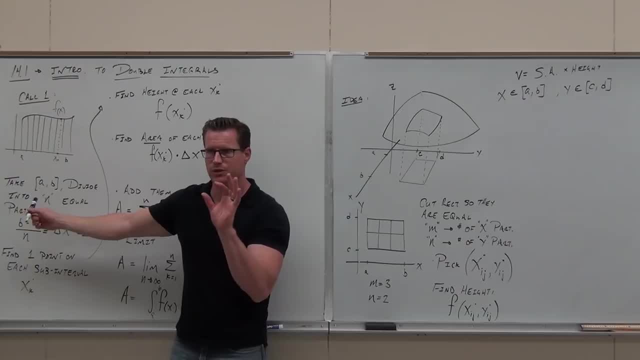 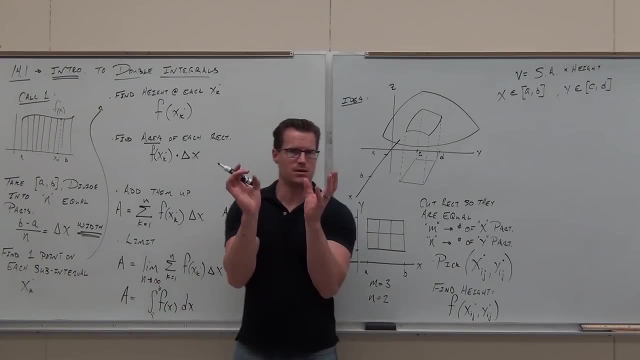 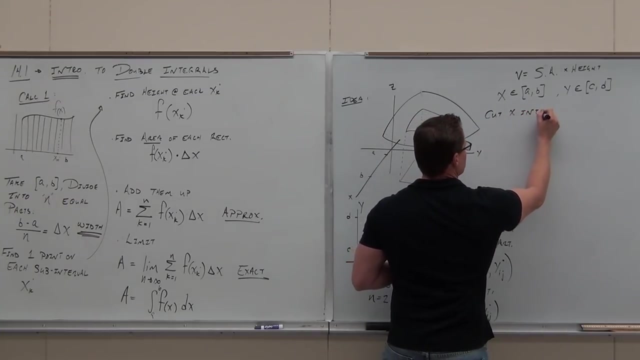 N intervals. The width of each one was B minus A divided by N, and it gave us delta X, correct? We're now cutting X into M. just a different change of just a letter change. We're cutting X- the interval of X- into M subintervals. 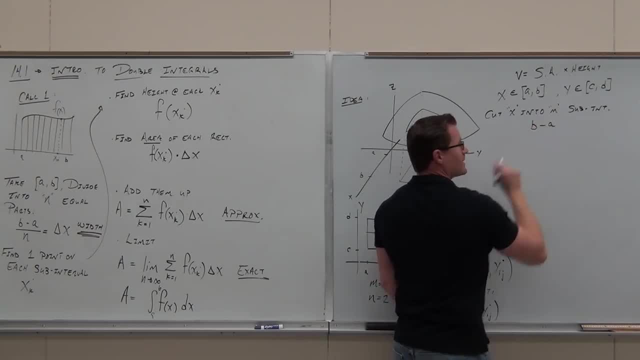 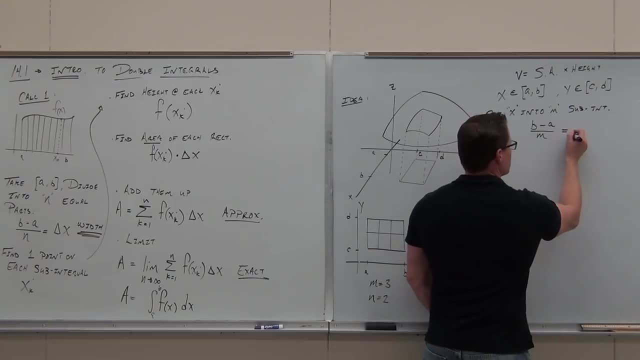 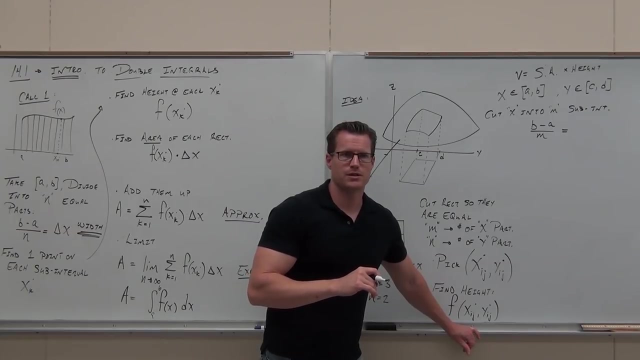 So X is still going from A to B. We're still cutting it. Different letter, but we're still cutting it. This is going to give look carefully. look carefully, because here's where all the money comes. okay, This is going to give us the width. 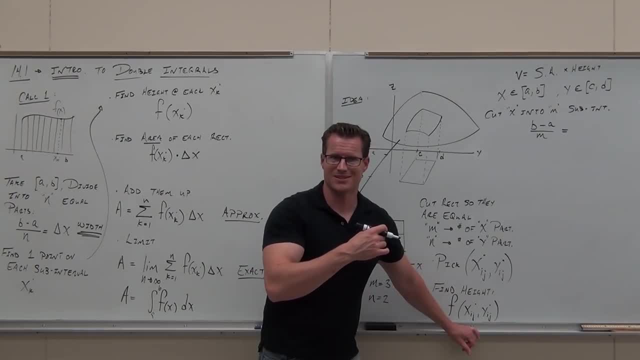 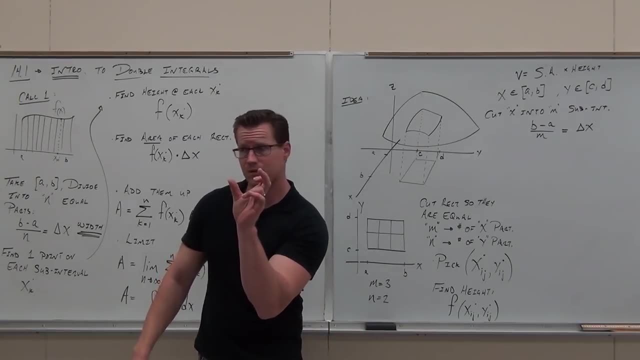 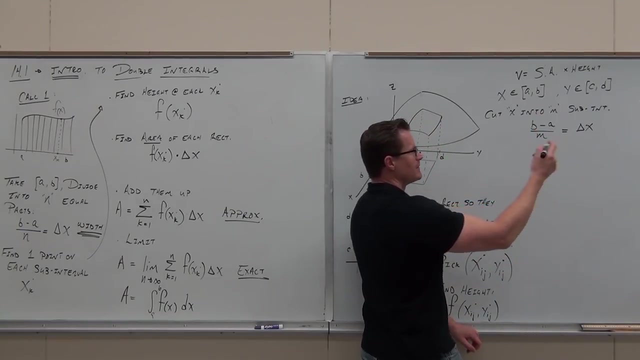 of each rectangle along the X axis. Does that make sense? That is the width of each, the width, Just like this Width, of each rectangle along the X axis. But now we're also cutting Y, B minus C into how many, how many cut-ins here? 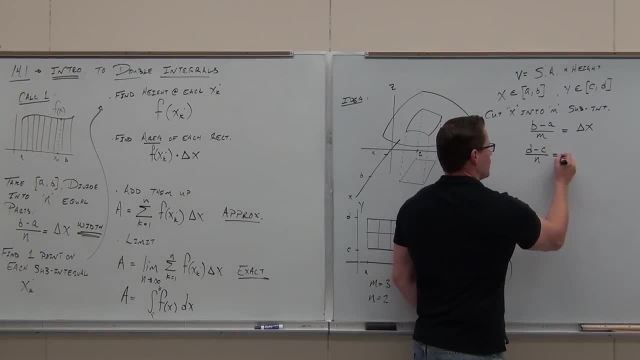 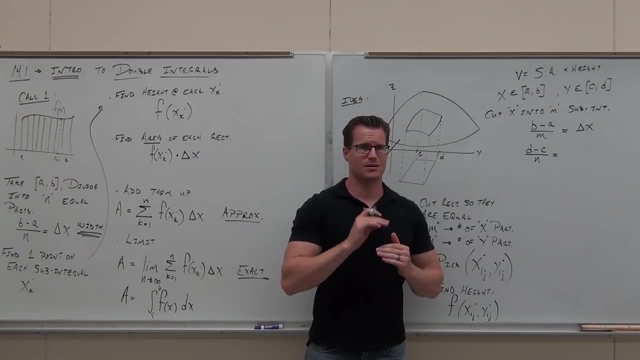 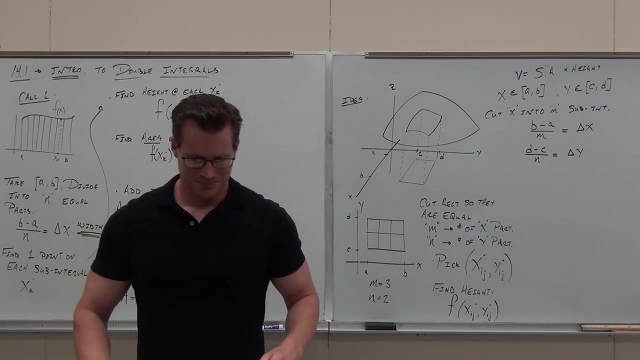 For Y. How many? Oh, This is going to give us the. if this is the width, then this is the height: The height of each rectangle along the X axis. This is going to give us the width of each rectangle along the Y axis. 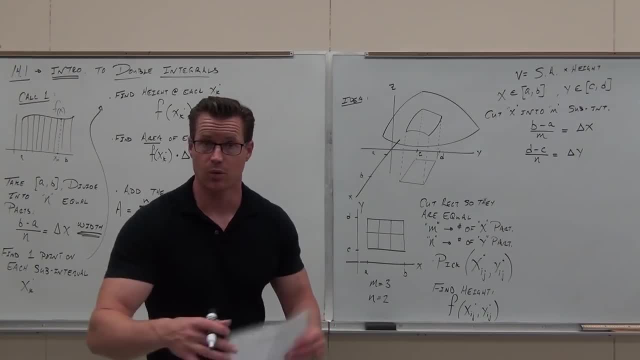 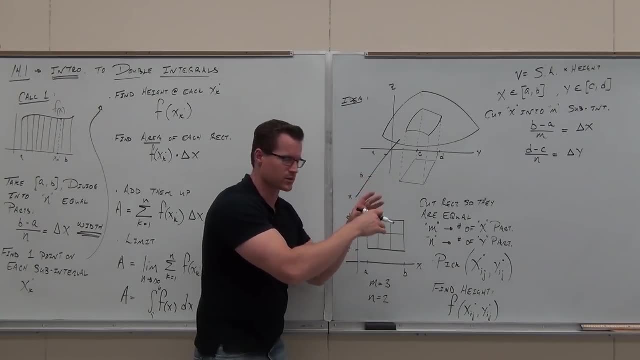 Are you still with me, Are you sure? So, so again the idea: drop it down, rectangle the region, Cut in a whole bunch of rectangles. How are we going to do it? Well, if you cut it into rectangles, 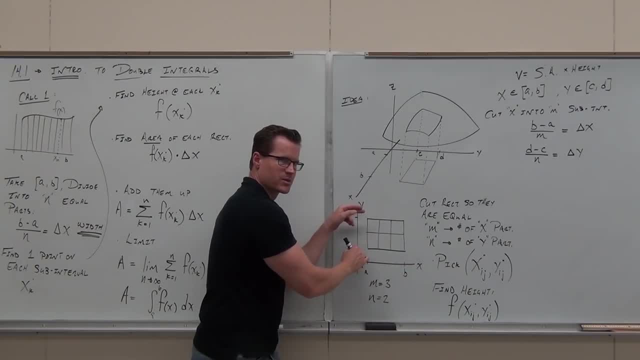 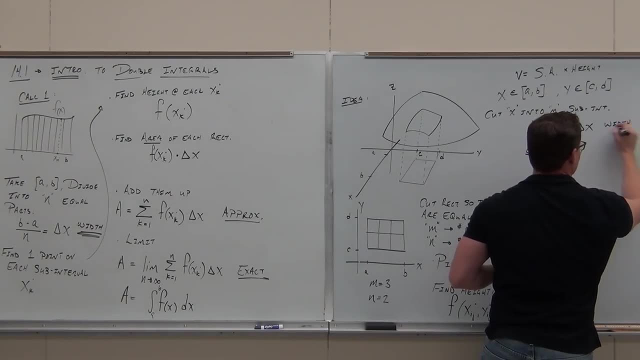 then there's going to be a certain number of segments along the X, certain number of segments along the Y. Cool, The width of each one here is delta X. This is your width, The height of each one. notice, they're all the same. 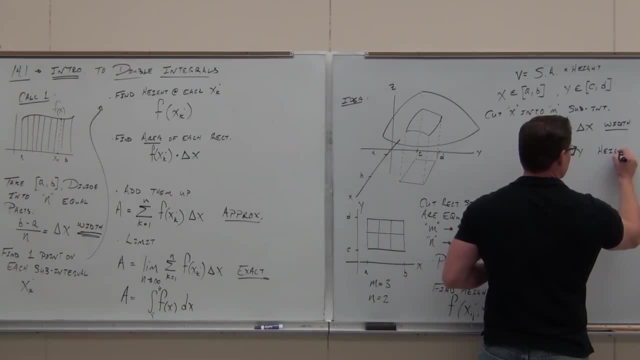 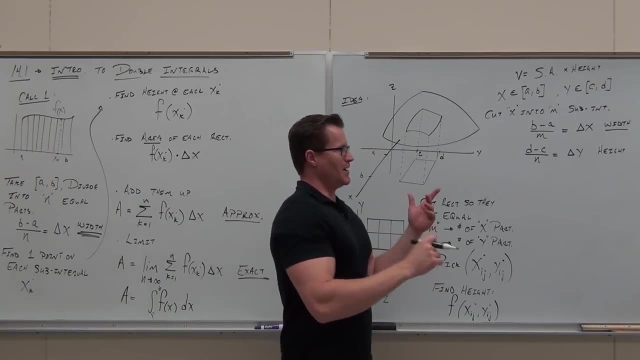 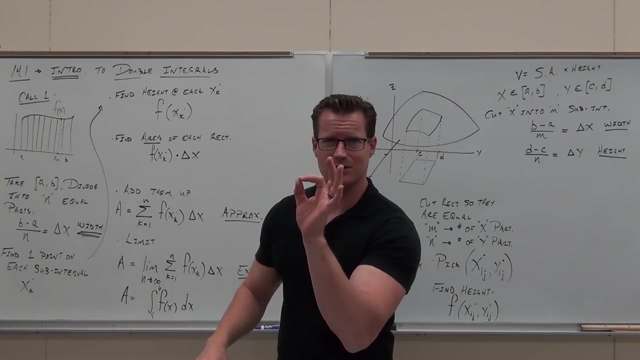 The height of each one is delta Y. We are almost done, Trust me, almost done. Hey, if your width of a rectangle is delta X and your height of the rectangle is delta Y, can you find the area of each rectangle? 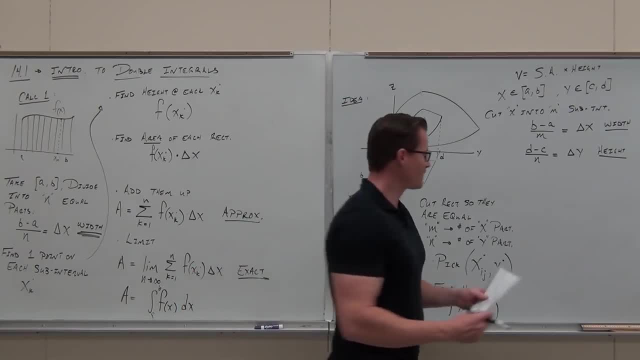 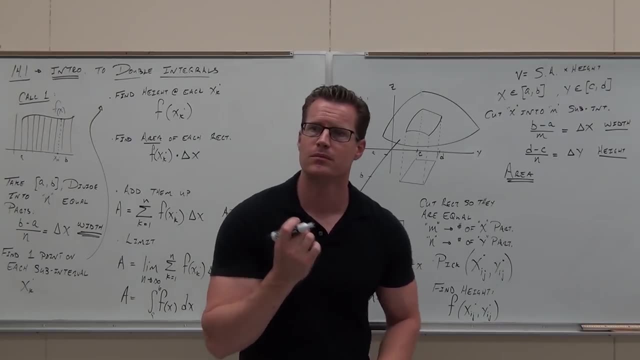 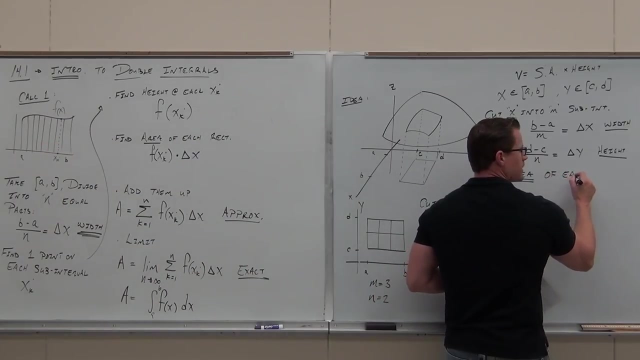 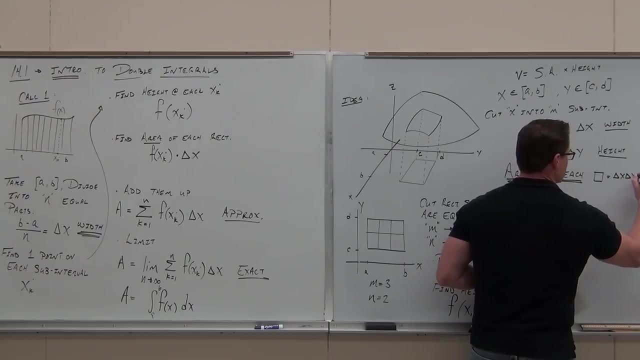 Boom. How True or false. The area of all those rectangles are identical, Just like the width here was all identical. The area of each rectangle is delta X times delta Y. Oh man, we're almost done. We're almost done. 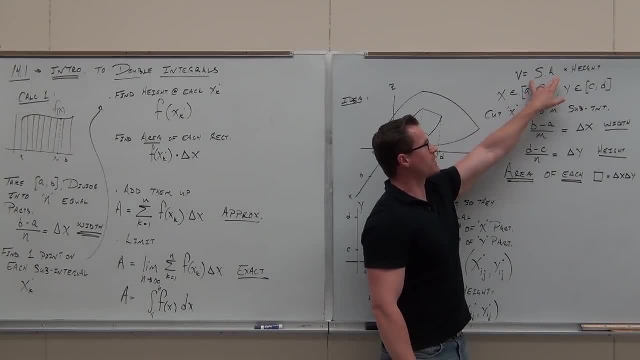 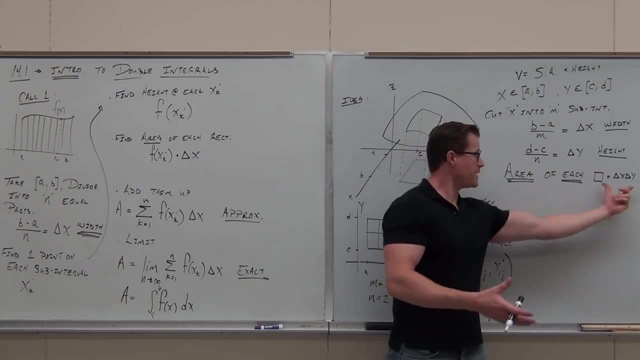 The cool part: if volume is surface area area, just think area. if volume is area times height, do we now have volume? We now have the area right there. Do we now have the height above each rectangle at an arbitrary point? 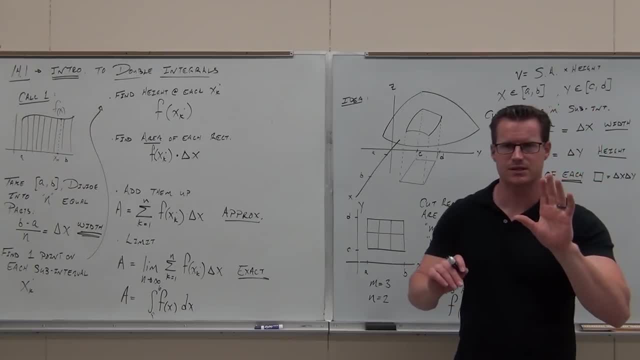 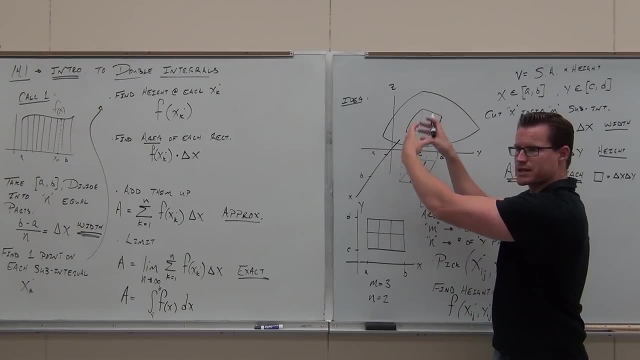 Yes, Therefore the volume. please listen the volume. so this is under here, right? We've cut it like this- The volume of each one of those rectangular prisms. we pick a point somewhere in here, We find the height of that. 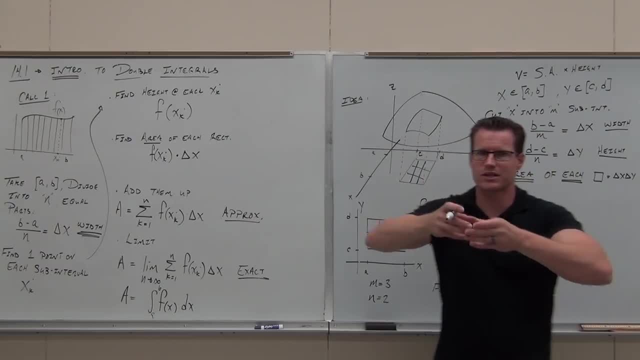 Area times. height gives us a volume, The volume of each of those little. we call them cubes. if you want the rectangular prisms with a weird top, The volume of each of those rectangular prisms is height at an arbitrary point for each rectangle. get it. 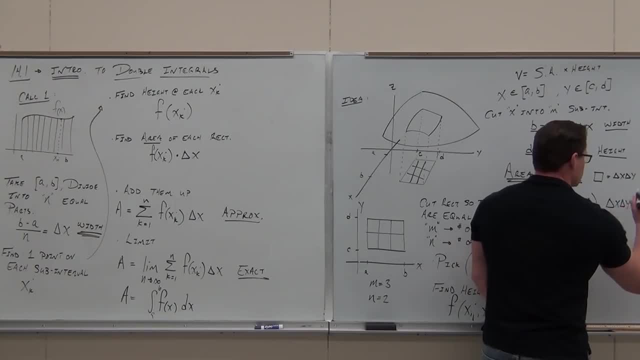 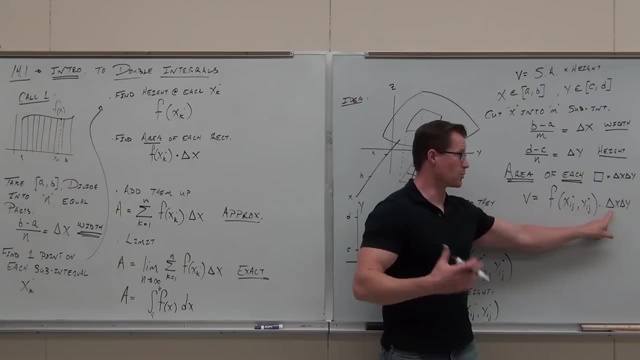 Times the surface area of each rectangle. Do you see that's giving you volume. Look at the board, Look Length, or well? So width times height of the rectangle times the other height. Length times width times height, that's volume. 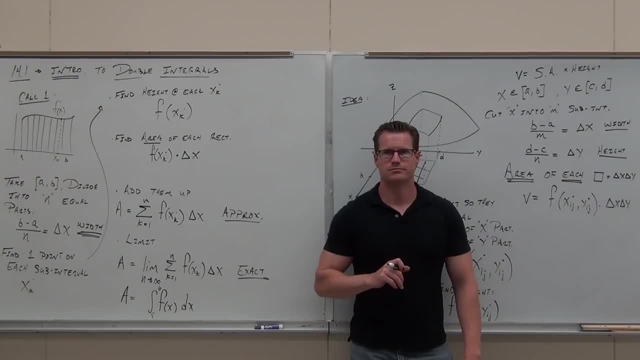 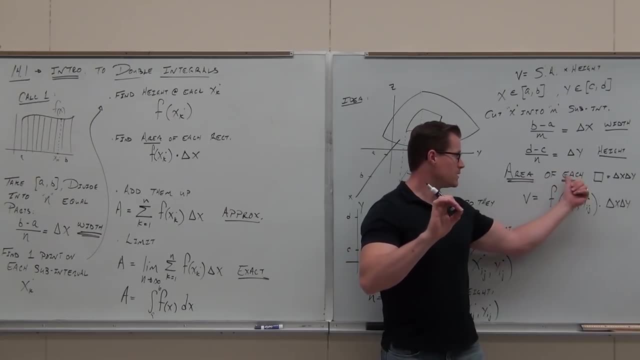 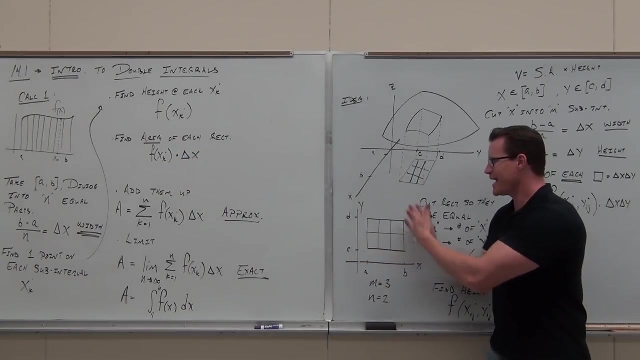 True or false. This is exact, True, False, False. That's false. This is the volume. please listen carefully. this is the volume of each rectangle, Just like this right here is the area of each rectangle. How many rectangles do I have? 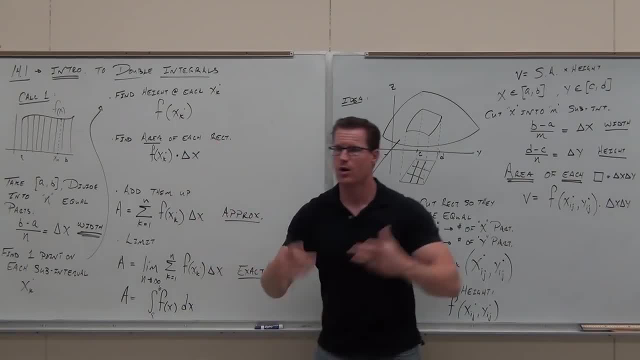 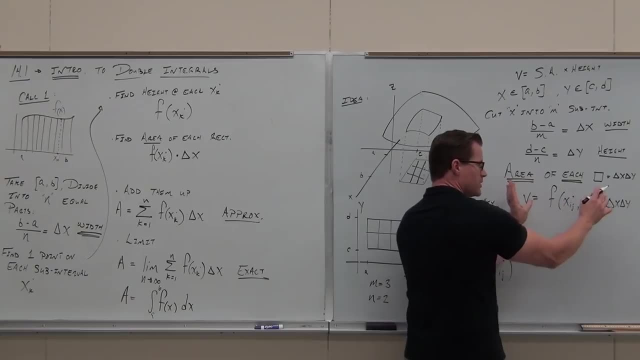 A lot of them. What are we going to do with the area of each rectangle? We're going to add it up. What are we going to do with the volume of each rectangle? What are we going to do? So if I have the volume of each rectangle, then the volume. 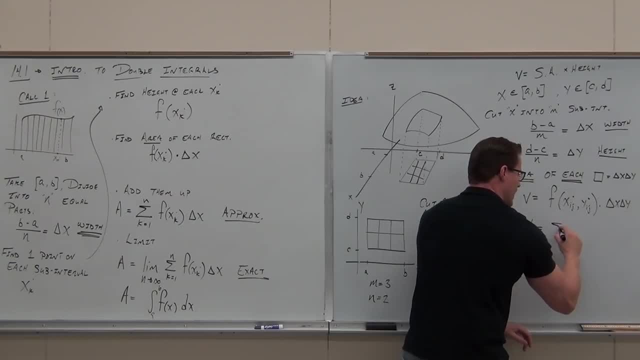 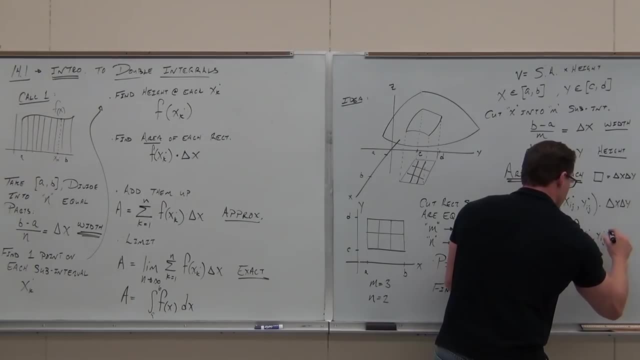 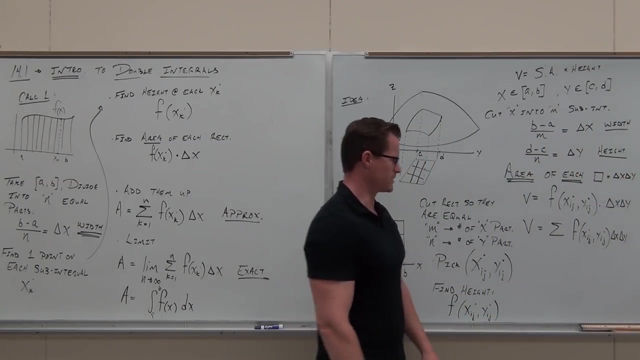 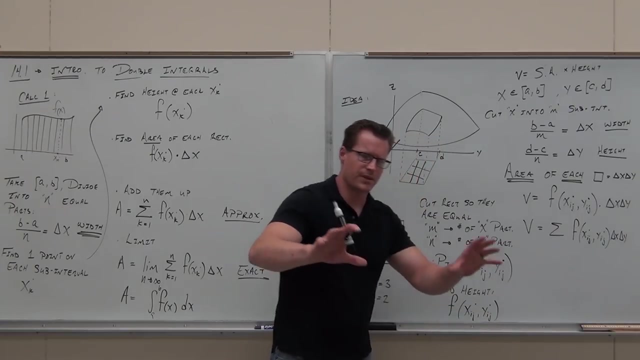 of the entire area under the surface is going to be. let's add them up. Oh wow, But wait a second. Add them all up. But here's the whole magic. Here's where a double integral comes from. You're not even listening. 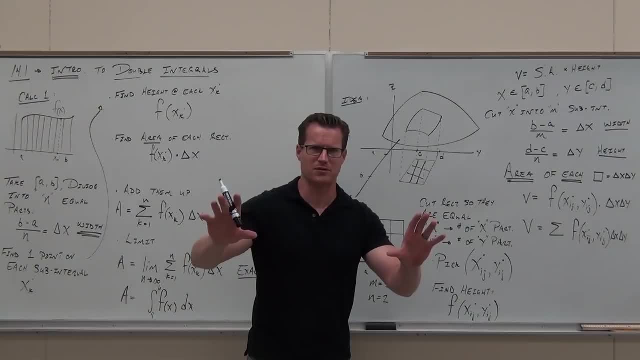 You should be listening. This is the cool part. It's all cool part. It's the coolest part. Gosh, darn it. Oh, exciting, Let's start speaking in squeaky voice. You're a monster. I practice that on the weekends. 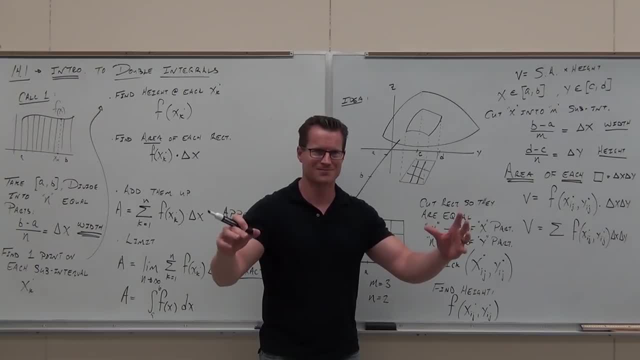 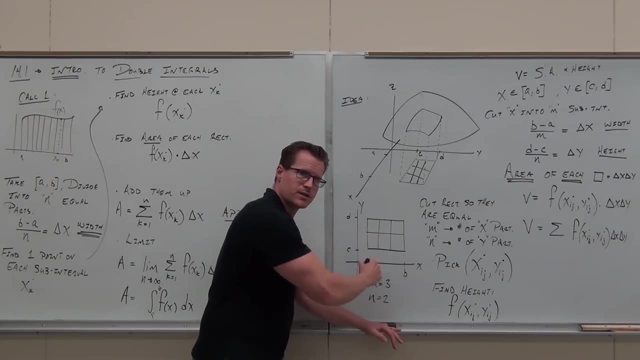 We watch kiddie movies and I just practice all the weird voices. Hey there ready. No, I can't do that. I can't do that. Look If you're at. If you're adding across two different dimensions, you need two different sums. 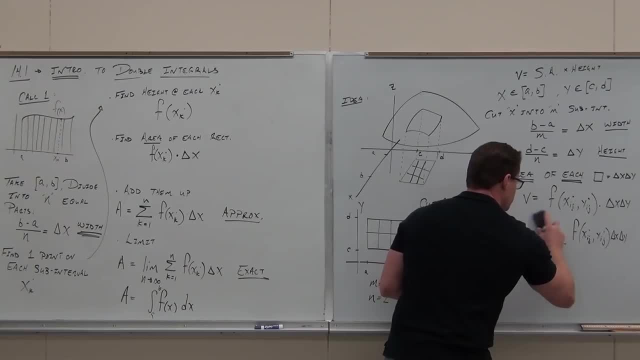 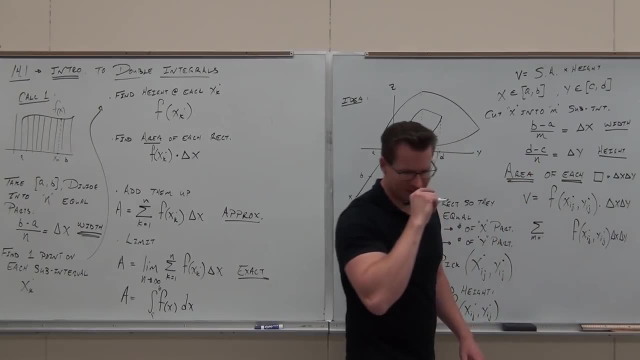 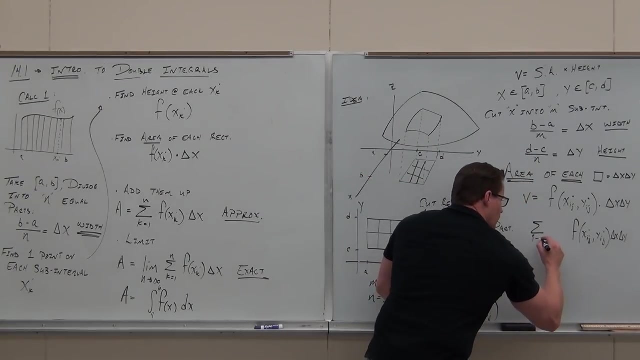 We need to do this. We need to be able to do How do I want to write? Yeah, I'll do it. I'll do it this way. We need to be able to let our I's start at 1 and go to M for X. 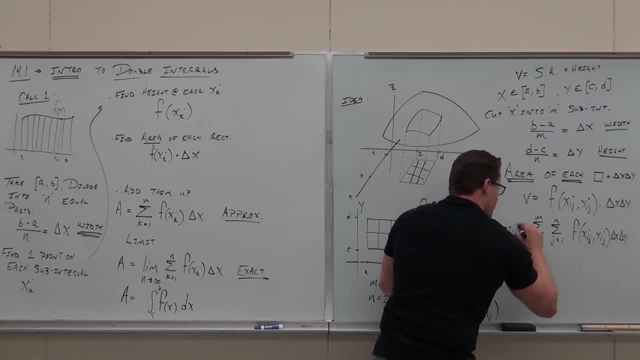 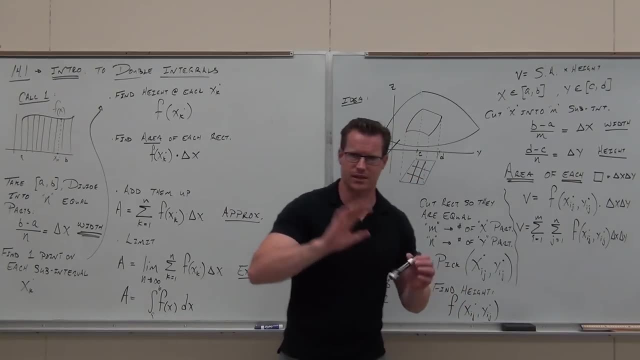 and let our J's start at 1.. I want to start at 1 and go to N for Y. I want to talk about this. I want you to understand this. I don't want you to. Don't skip this. Okay, Don't miss this. 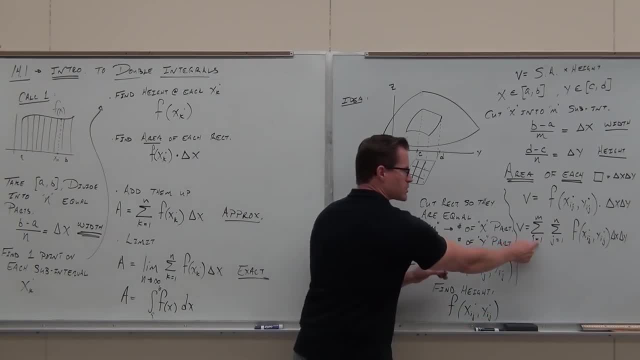 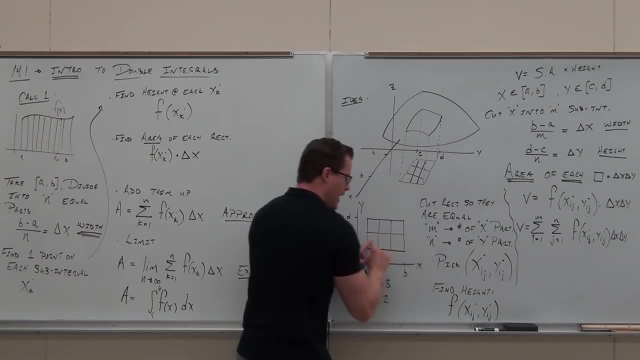 Watch what has to happen. Watch what has to happen. It says you're going to start at the very first rectangle, but for every time you have the I equals 1.. Do you understand that I would go 1,, 2,, 3,, 4,, 5,, 6,. 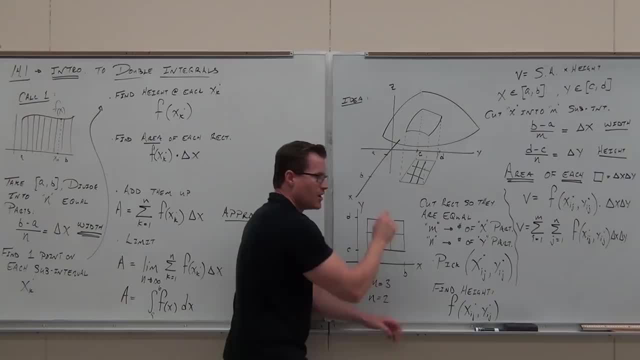 and J would go 1,, 2,, 3,, like a grid. Do you guys see that For every time I get one of these I have to run through the whole gamut of those? So for I equals 1,, I go. oh, I equals 1,, J1.. 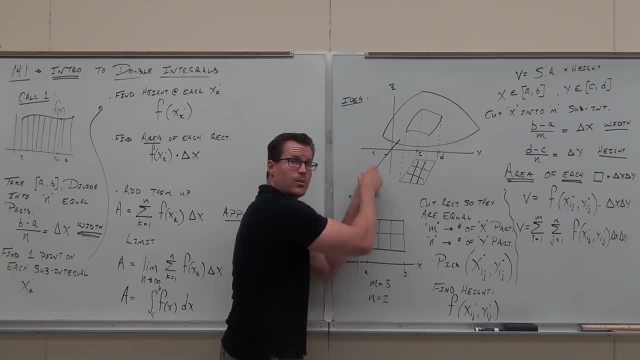 I1, J1.. I1, J2.. I1, J3.. And I have to add up all that row column, add the whole column. Then I have to let this go to 2.. But when I let it go to 2,, now I have to start over. 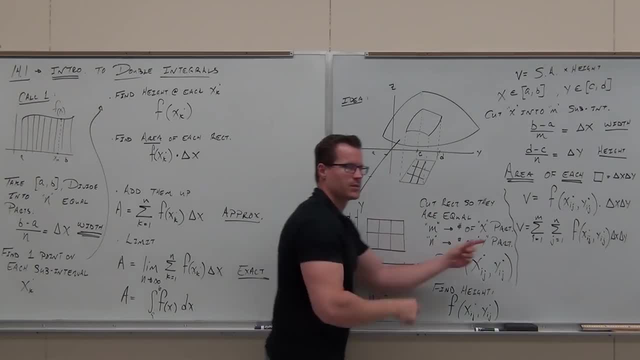 2,, 1,, 2,, 2,, 2,, 3,, 2.. Then I have to go 3,, 3,, 1,, 3, and that's how we do it. We add up a double sum. 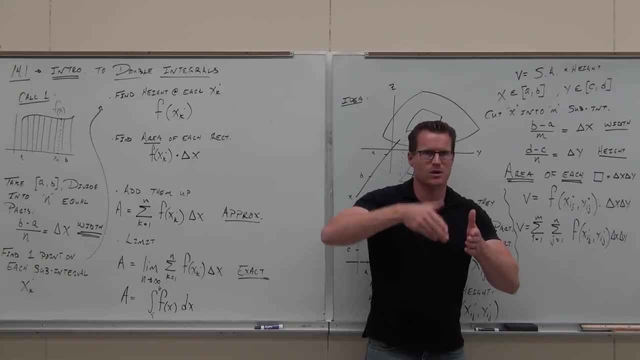 That's what we're doing. We're going up the whole thing. We're going up the grid of rectangles And every time we switch we have to go up the grid again. That's what that says. I don't know if you're okay with that one. 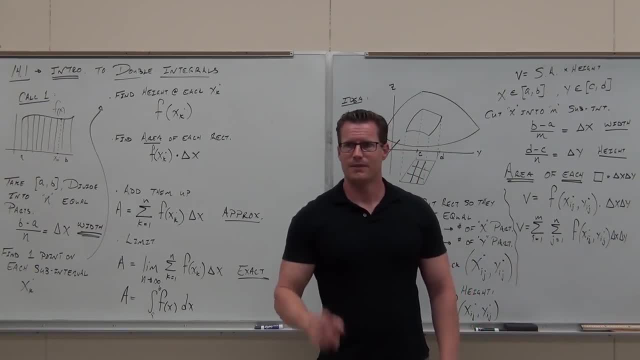 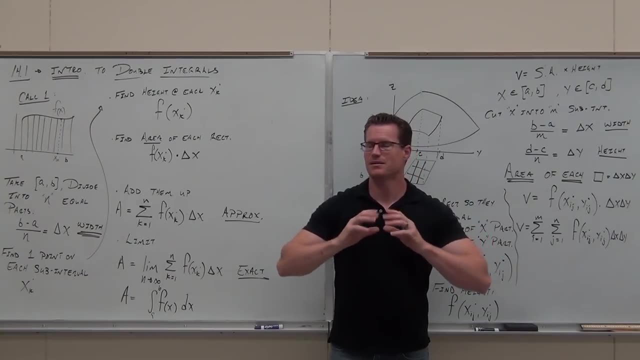 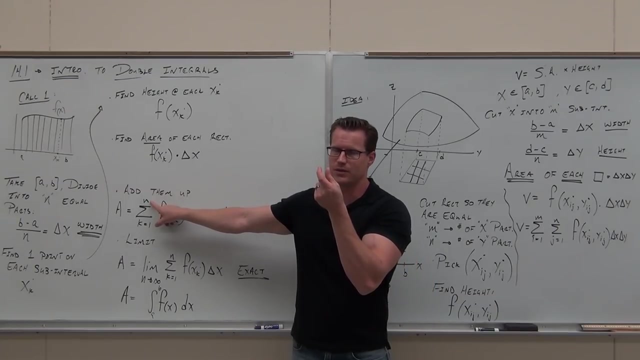 Now we'll ask: is this exact? That's an approximation, because I have a finite number of them. Oh my gosh, for all the money in the world which I don't have, How do I make it better If that's finite? I wanted the widths to go well, not the widths. 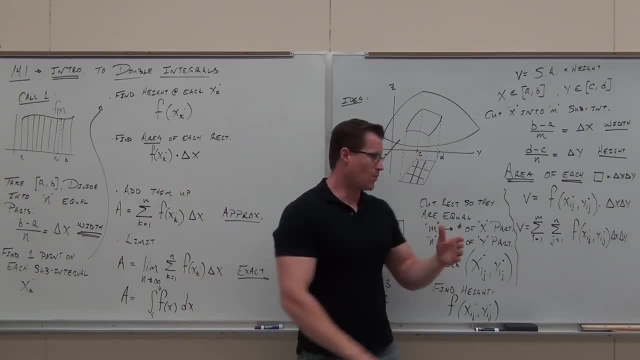 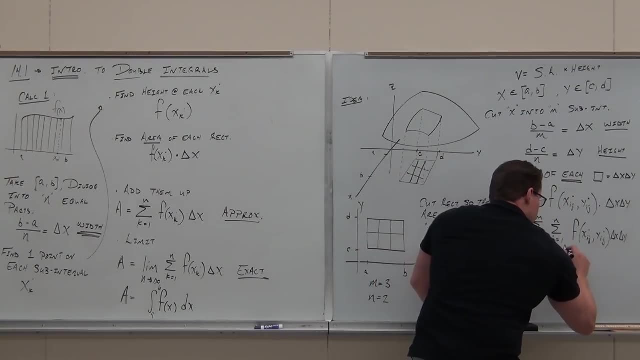 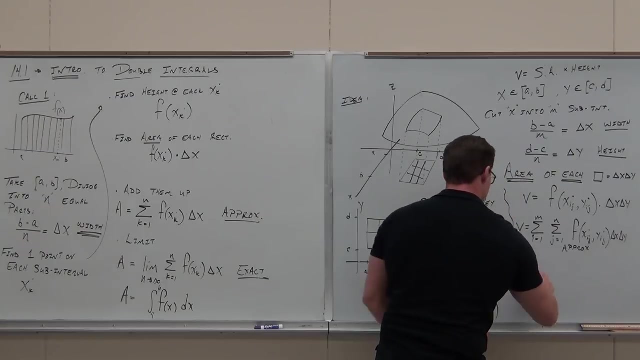 I'm sorry. I wanted the number of rectangles to go to infinity. I want the number of rectangles to go to infinity. So this is an approximation, because it's finite. I'm going to do it over here. It's too important for me. 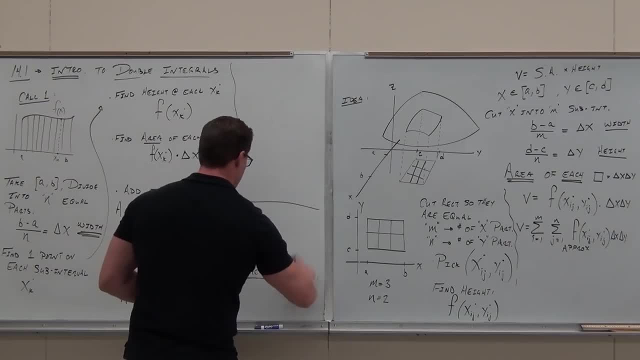 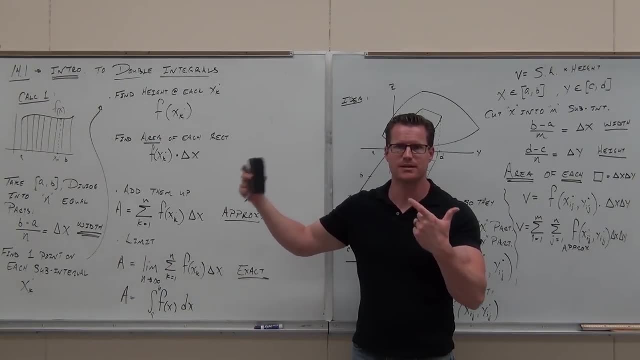 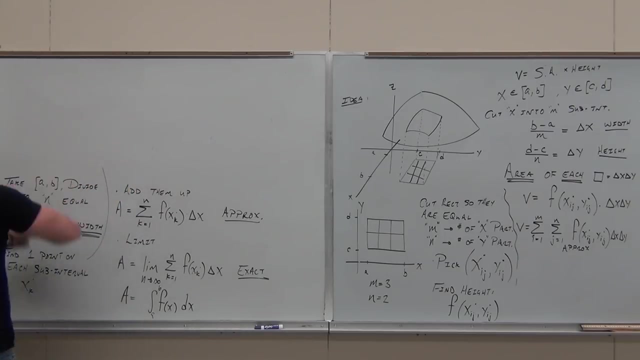 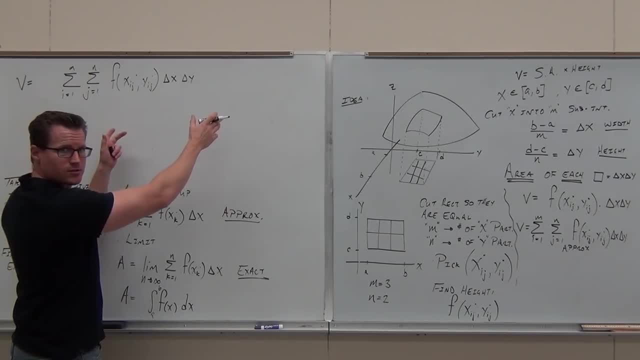 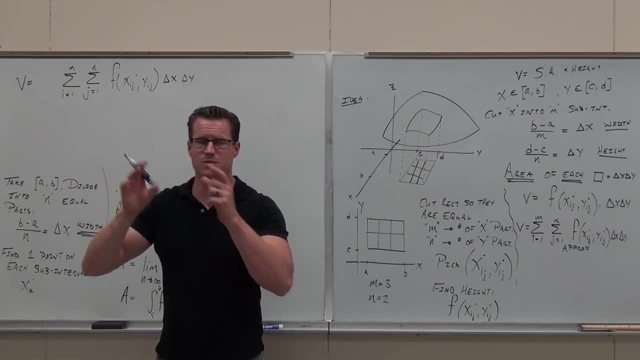 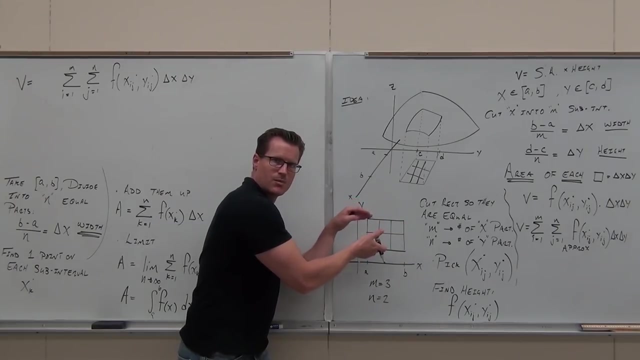 see if you were paying attention. Some of you guys have your eyes closed. Good, that's great. Exact or not Approximation: How do I make an exact? I let the number of rectangles go to infinity, which means I let this go to infinity, let the number of segments along x go to infinity and the number of segments along y go to infinity. It means that the arbitrary point doesn't matter, because our rectangles are getting so close together. it doesn't matter where you pick it And the way I do that. I take a limit. 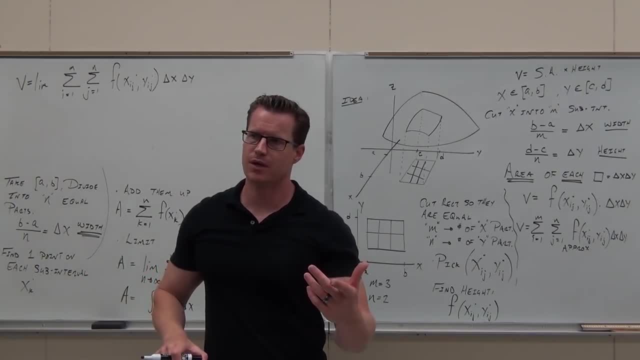 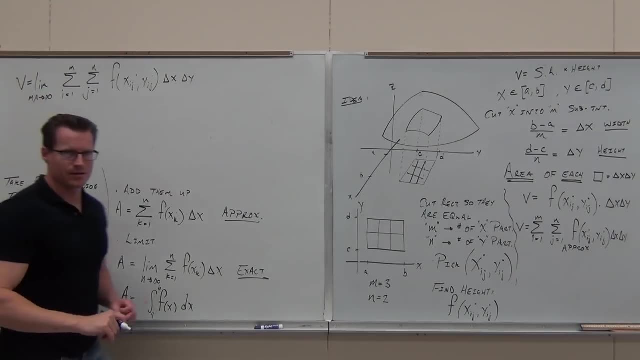 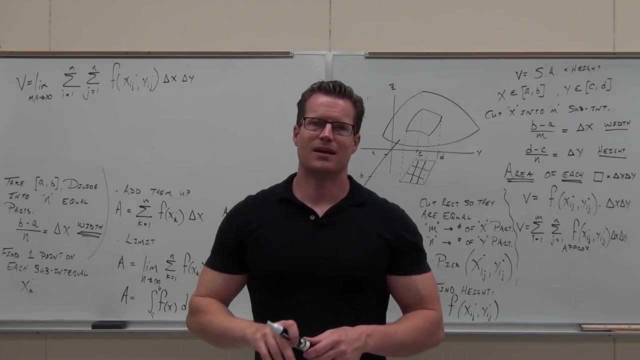 However, the limit does two things. The limit lets both m and n. m and n both go to infinity. Cool, right Now I'm going to pause right here before I give you the final punchline, which is it? and then we do like two examples and we call this thing good. 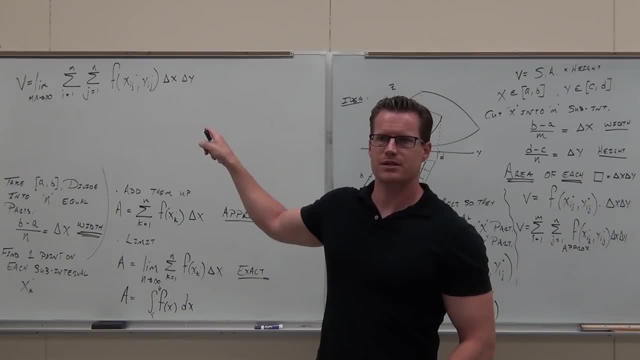 Do you see where everything's coming from? Because, honestly, a lot of people get to this level and they've never even seen this before, which shames me. I do it in Calc 1.. It's there, But some people don't. They just go: oh, this is how you do integrals. That's crazy. okay, You need to know where that comes from. That's why I gave it to you. Do you see where that comes from, though? Let's look at it. What is that? 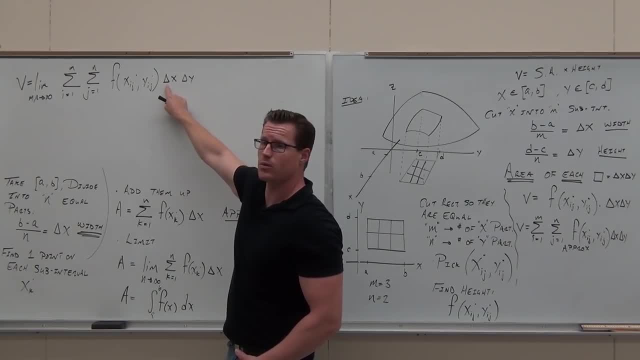 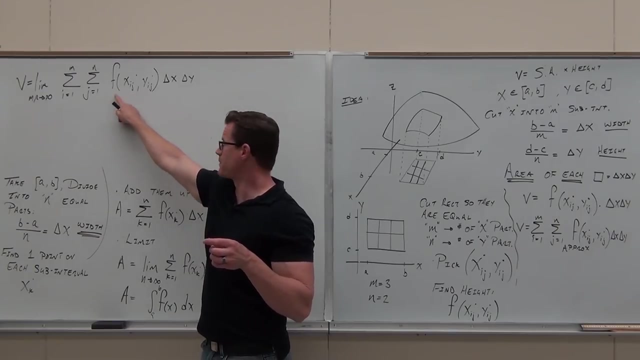 It's the area. This is not the area, This particular one With along the x. What's that? This is the area of each rectangle. This, What's this? Without the f, Without the f, Without the f, That's an arbitrary point on each rectangle. 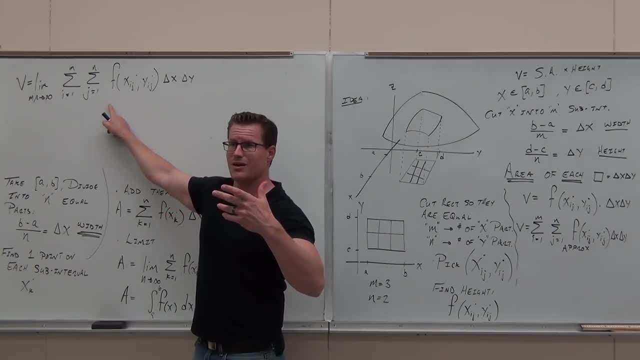 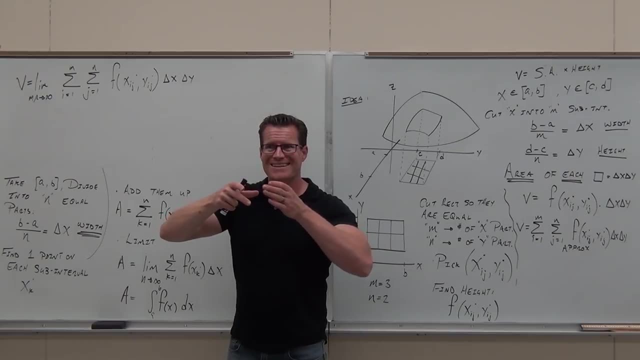 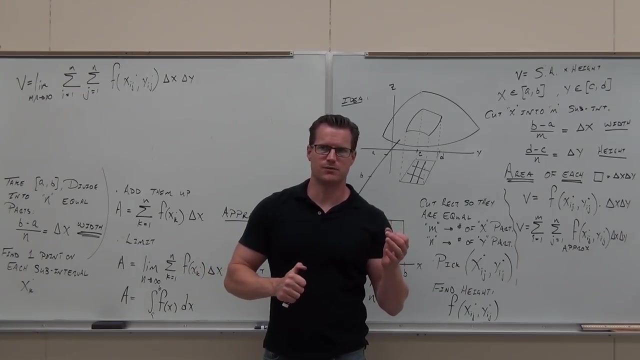 The f gives us the height. So this is area of each rectangle times height. That's the volume of each little prism. As I add them all up across the grid and let the number of them go to infinity, the arbitrary point doesn't matter wherever you pick it, it's going to end up being squished in the very middle of that. it doesn't matter, it's so small, it's in there somewhere. and then I add them all up after taking that limit. that gives me not an approximate volume anymore, that gives me an exact volume. 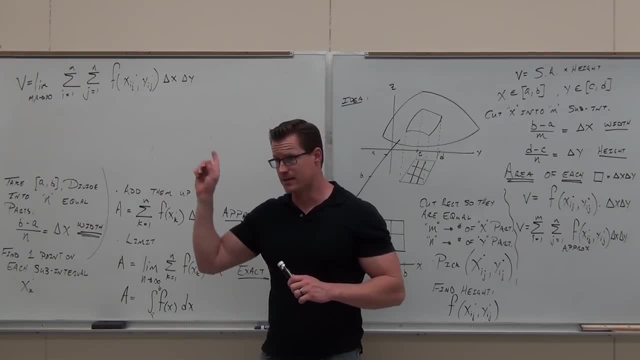 That's calculus. That is what it is. It's that idea right there. And we make it easier, We do some definitions to say you know what, every time you take a limit of a sum- we talked about it right here- the limit of a sum gives you what. 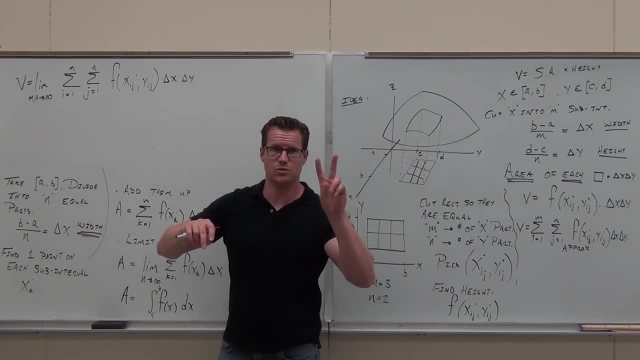 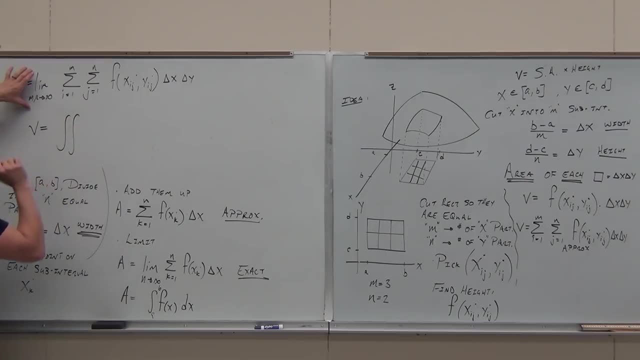 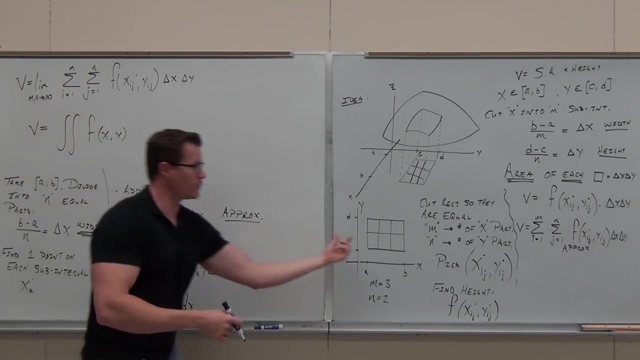 So the limit of two sums gives you two integrals. This is two integrals. A function of an arbitrary point gives us a function with two variables. Every time we have a Delta x going to notice, if m and n go to infinity, the width between them go to zero. 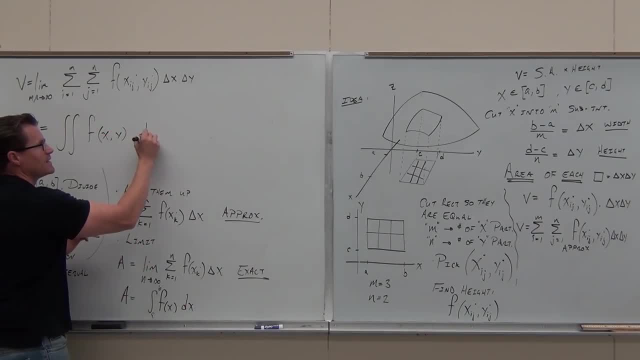 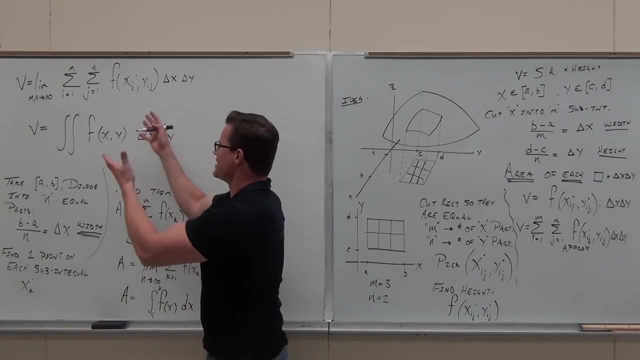 Every time we get a delta x and a delta y going to zero, we have a dx and a dy. That's what that represents. It says the distance between them is going to zero and you're adding them up. This is exactly what this says. 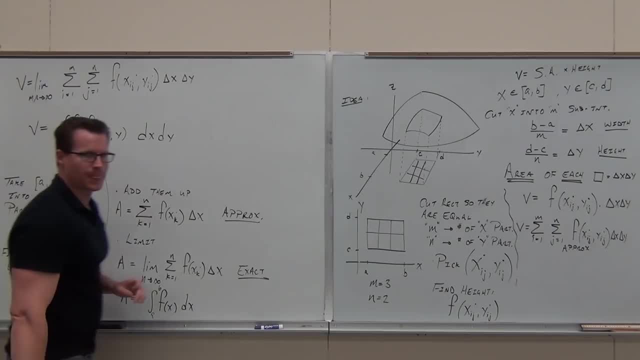 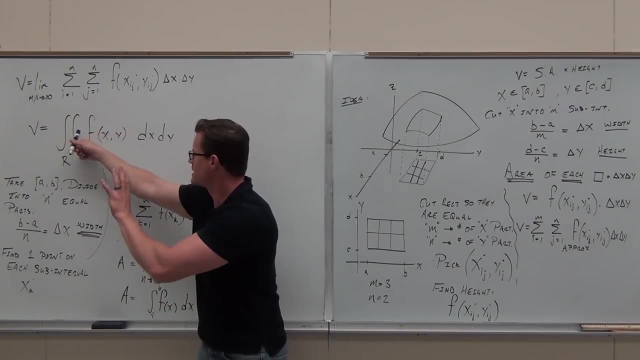 It says that over some region, over some region, I am going to add up, add up across the grid, a whole bunch of rectangles where this is the height of each rectangle And that is an area that's approaching zero of each rectangle, double integrals. 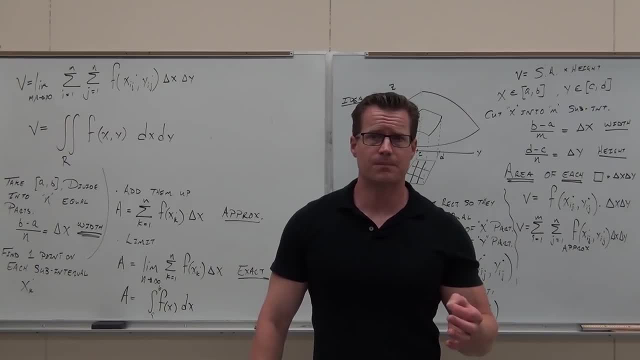 Both. That's what double integrals mean. So don't lose it, Don't just start doing calculus and be like: oh, I'm just doing double integrals, What do they mean? What are you doing every single time you do a double integral? 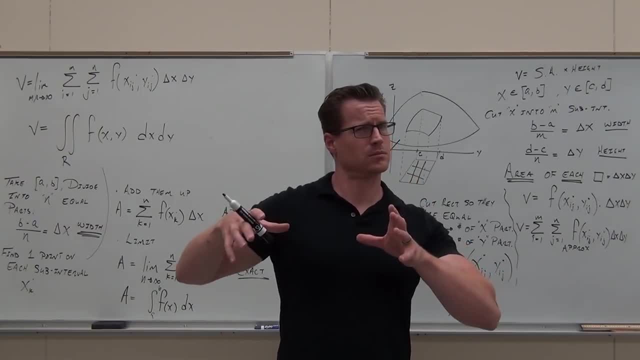 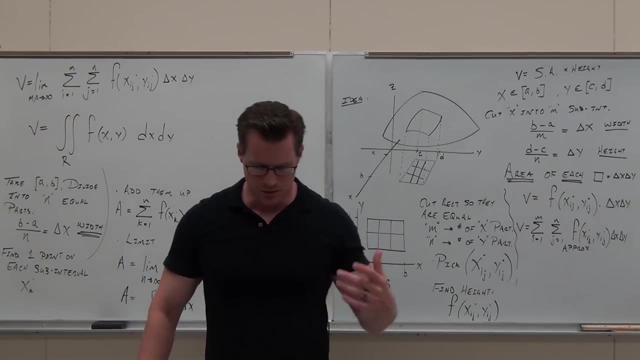 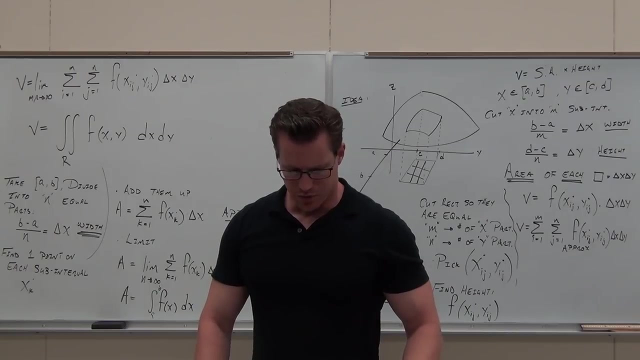 Finding the volume under a as bound by whatever region that says. So far we've dealt with rectangular regions. I'll show you how to deal with non-rectangular at the very end. We're not done yet, But that's it. I'm also going to try to kind of prove Fubini's theorem right now, which you don't even know what that means, but you will shortly in 14.2.. 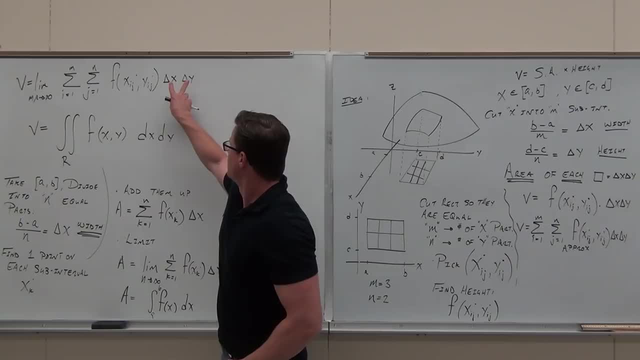 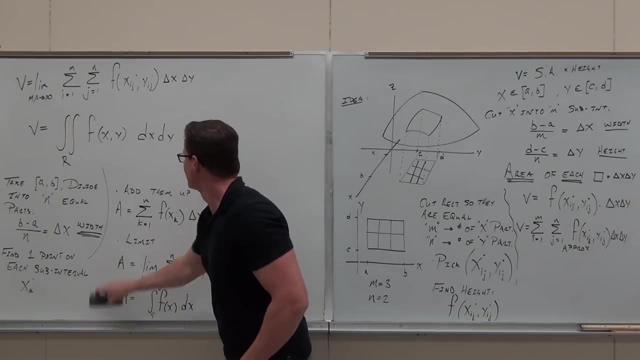 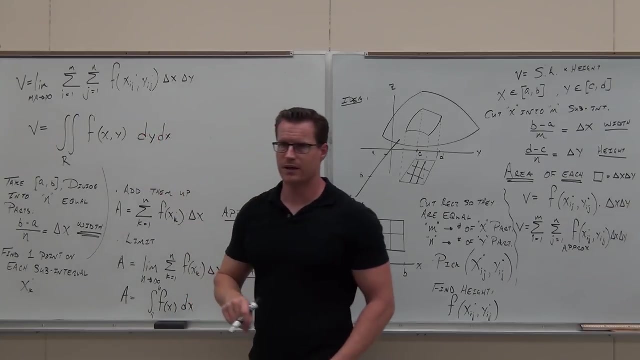 Here's a question: Does area matter in which order you multiply? No, So if I have this or this, will I get the same result? Fubini's theorem for rectangular regions Proved It's basic, It's multiplication. 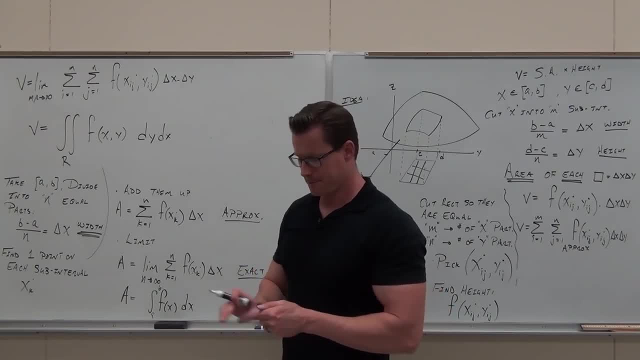 Multiplication is commutative Proves Fubini's theorem right there. Yeah, Since we have two variables when we integrate that, are we going to have to integrate with respect to y and then integrate with just respect to x? Now, that's a question for the next section. 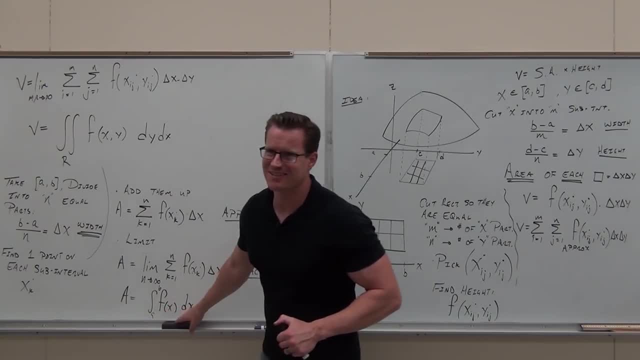 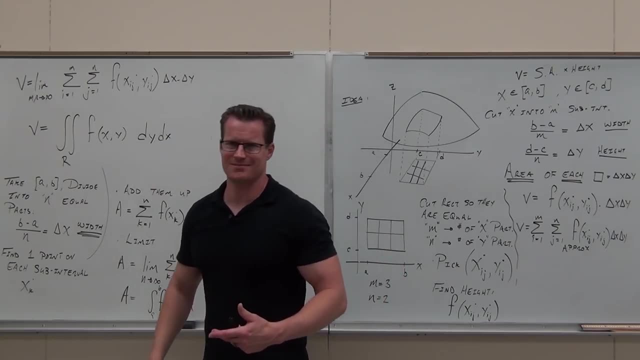 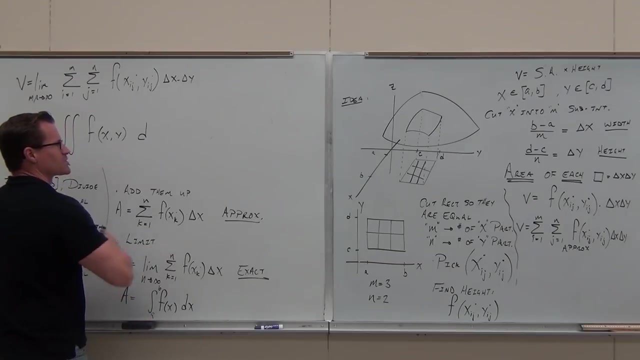 Yes, Remember partial derivatives. How would you do the opposite of a partial derivative One, then the other? Piece of cake, Sort of, But the idea is the same. Ladies and gentlemen, do you understand where double integrals come from at this point? 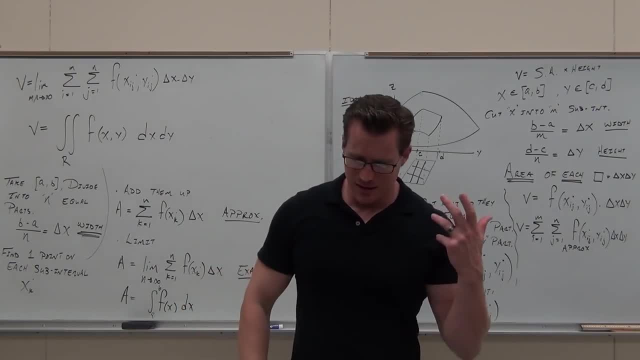 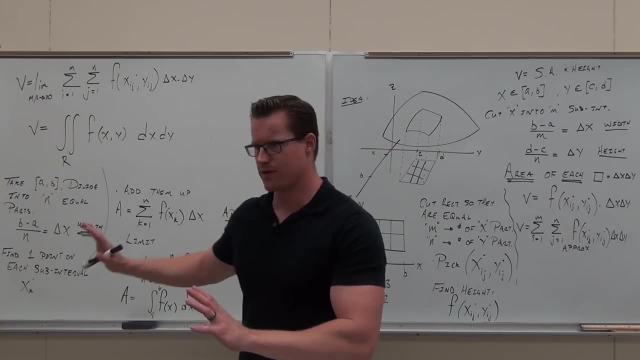 Now I would be remiss if I didn't give you at least like two examples of how to actually do this with the Riemann sum sort of idea. So we're going to do that. It's going to be fast. Leonard's version of fast. 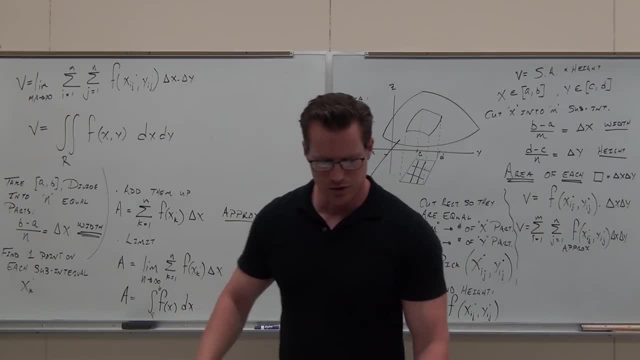 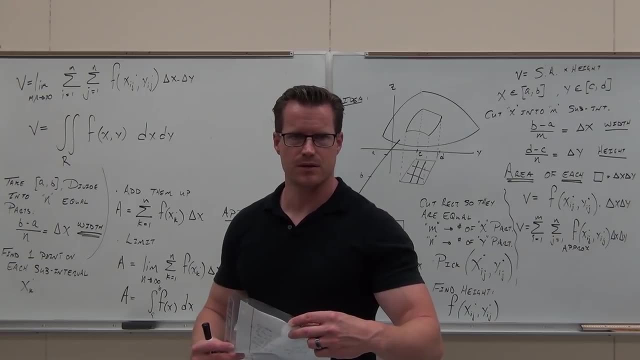 I'm going to show you. Well, You'll see. So let's do one example, because I want you to at least see it where it comes from and see the working of it. Are you guys with me on this, Too bad. 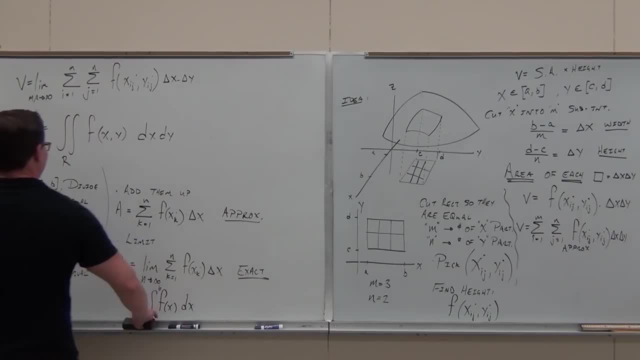 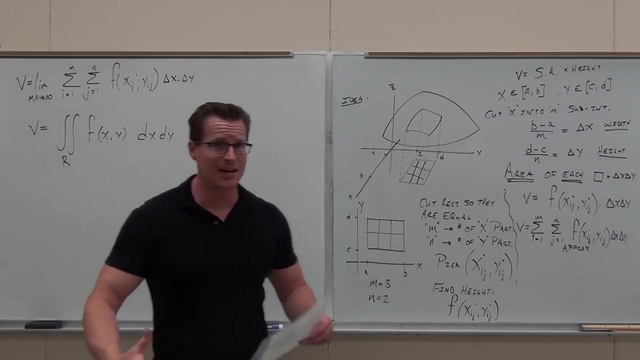 You're going to do it anyway. No, Please, Why? Because I want to, Because this is the good stuff, This is the, this is the bright point in your math day, Right here, When we get to practice Woo. 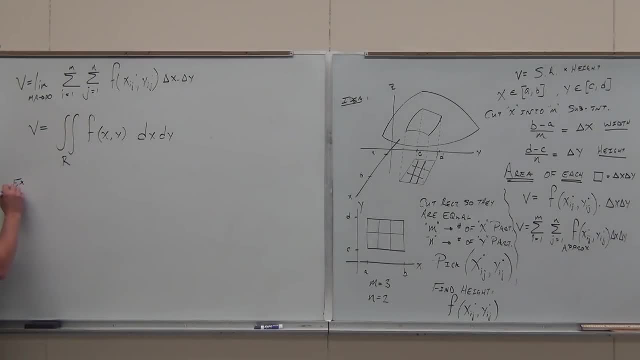 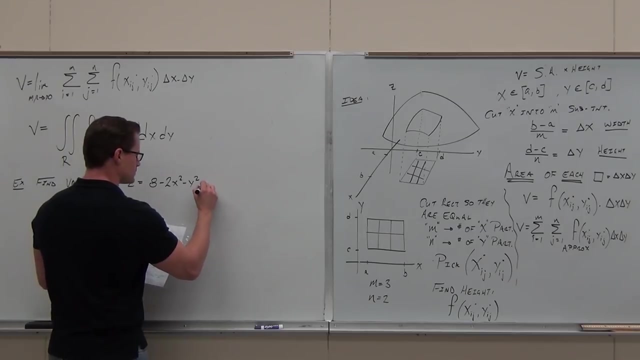 This is the bright point in your math day Function. I want to find an approximation for the volume of the following function on a given rectangular region. I will find an approximation for the volume of the following function on a given rectangular region, Of the following function: 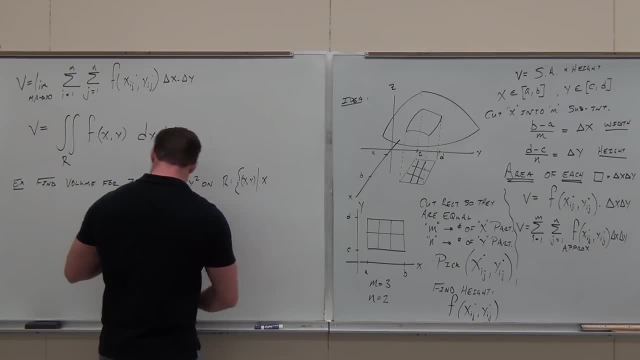 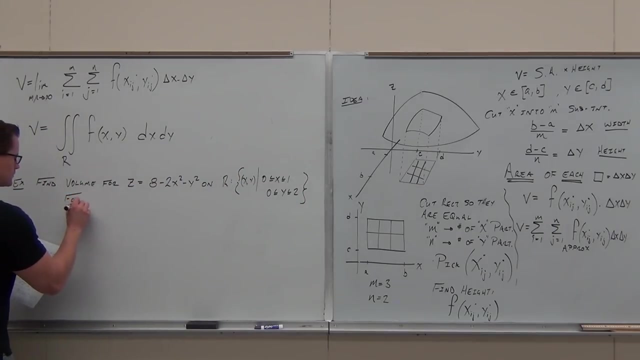 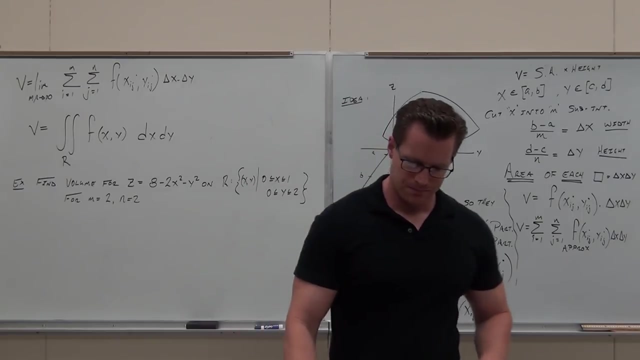 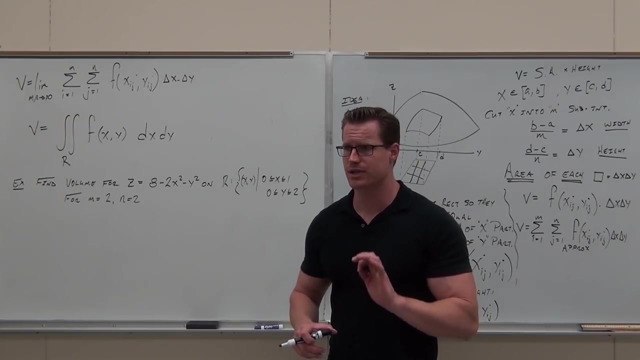 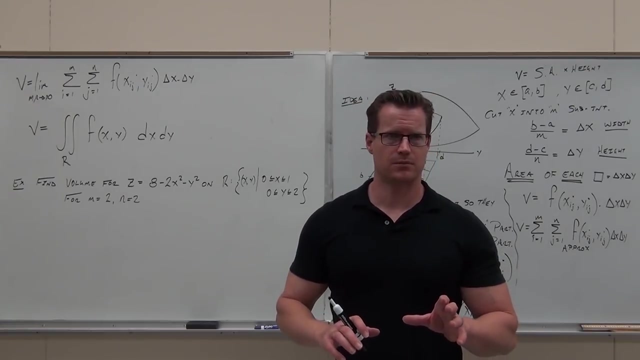 It looks pretty wordy. Trust me, this stuff is really easy because you are literally just plugging in numbers and adding things together. It's really easy. However, just like before, in order to do anything, you're not listening now, but you should be. 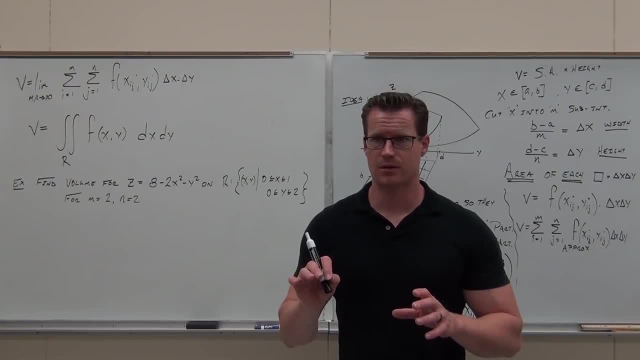 Put this in the back of your head Anytime you do anything with anything involving a region, just like in 13.8, anything that means double integrals. that means, right here: draw the region Every single Single time. draw the region. 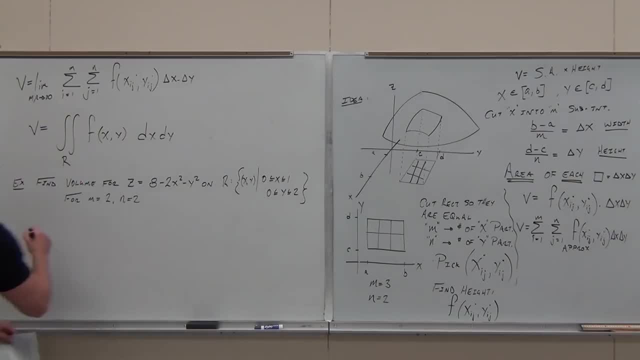 So we're going to start that right now. Let's draw the region. Notice how X and Y create for you this nice rectangular region. X goes from 0 to 1.. Y goes from 0 to 2. And we have this semi-rectangular region. 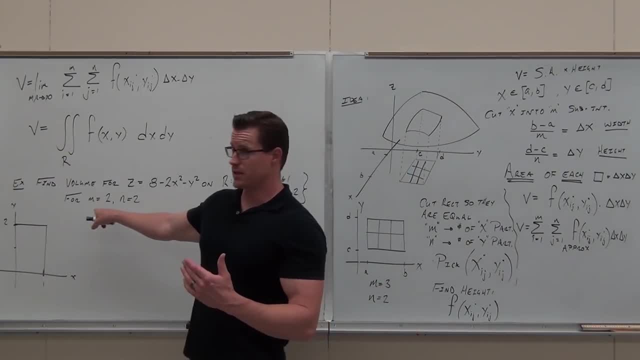 It also says this: I will, I want to cut this, And this is why you need to know what M and N means. I want to cut the X axis into two segments- equal segments, And the Y axis into two segments- equal segments. 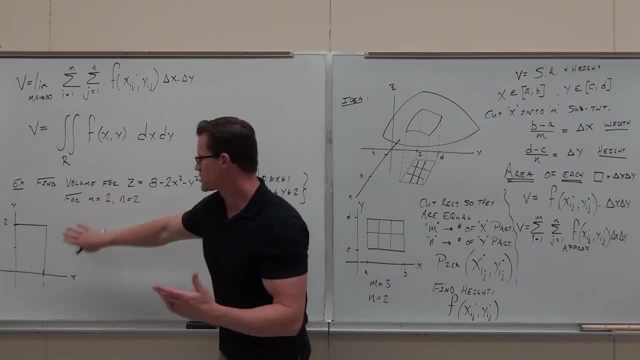 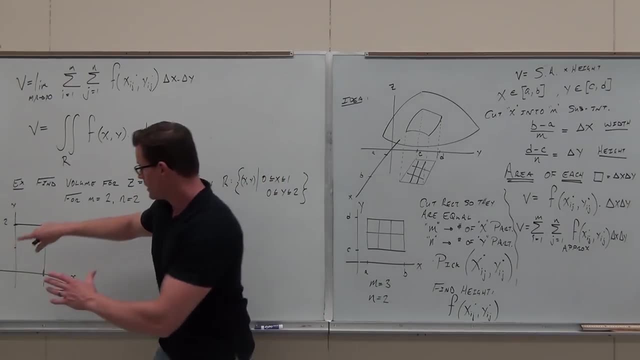 We're now creating this. Look, look, look. Here's a picture, a bird's eye picture of the XY plane. The surface is over that. somewhere You can tell it's a surface over the XY plane. Now I'm saying, well, look at that surface. 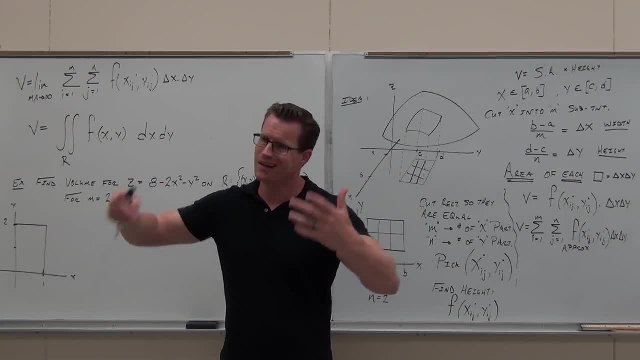 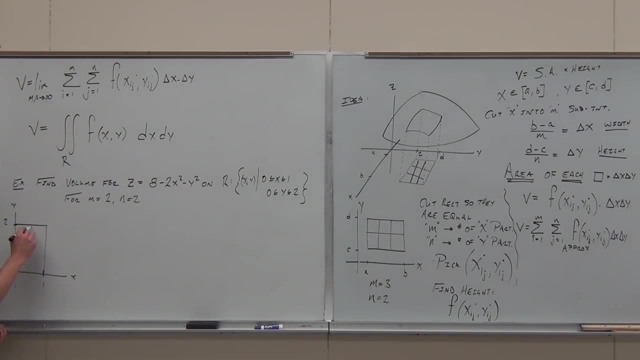 It's going to make a cutting on the surface. Find the volume beneath it. How do we do it? Let's cut that region underneath the surface. Let's cut that into some rectangular. How many? Two each. So two cuttings each. 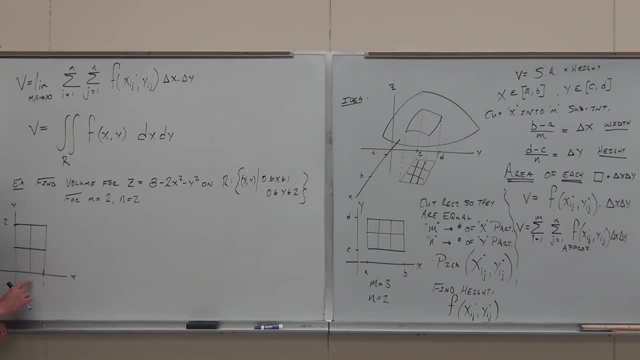 Hey, how about this? Look at the board. What's that if I cut this in half? What's that? What's this if I cut this in half? I can do it, Just cut it in half, No problem. I could cut it into tenths if I want to, but I'm not that sadistic. 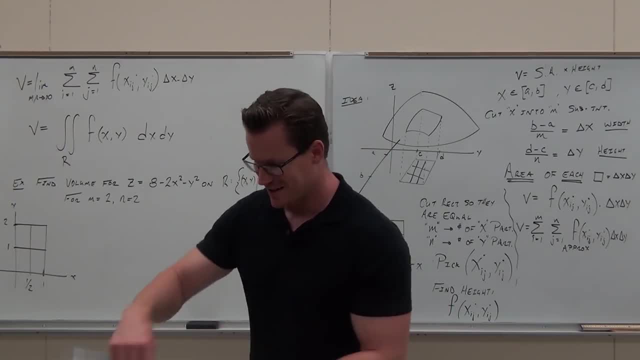 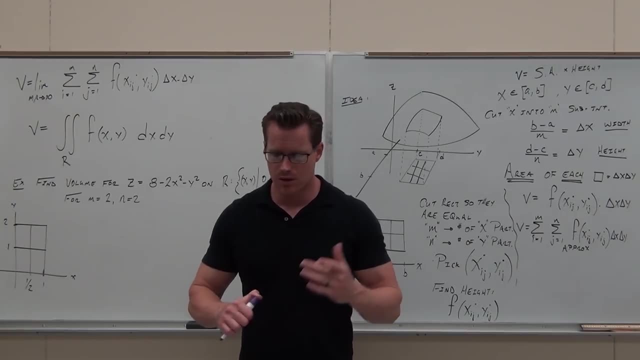 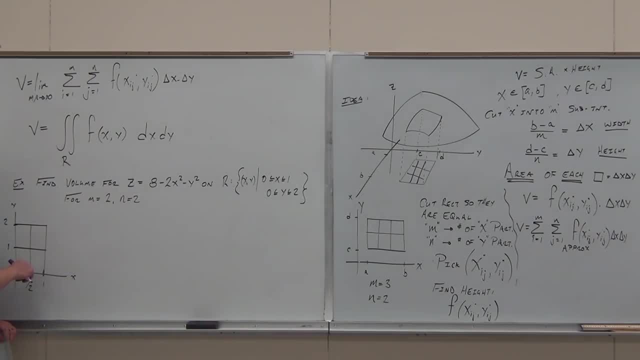 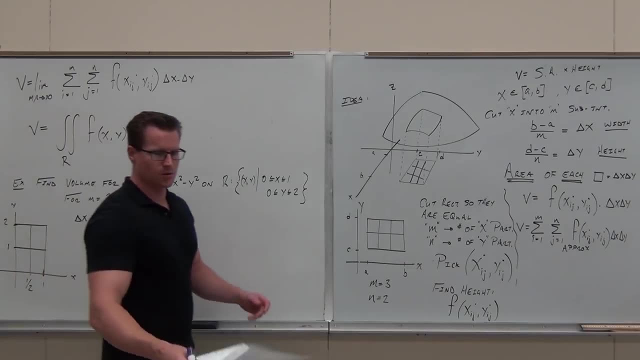 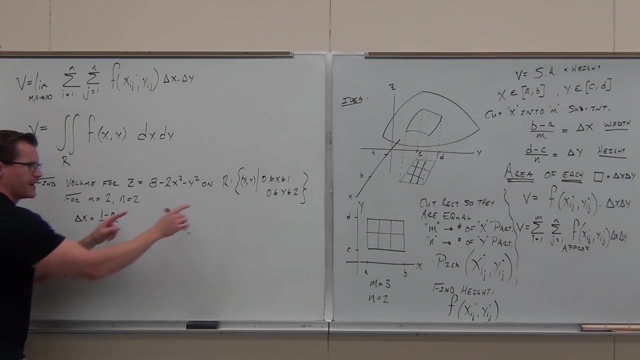 You can tell it's going to be one half. The width is one half, The height is one. Do you see it? If you didn't know how to look at the picture and do that, you could do just from delta x You go. well, delta x says that I'm going to take my x bounds here and divide by the. 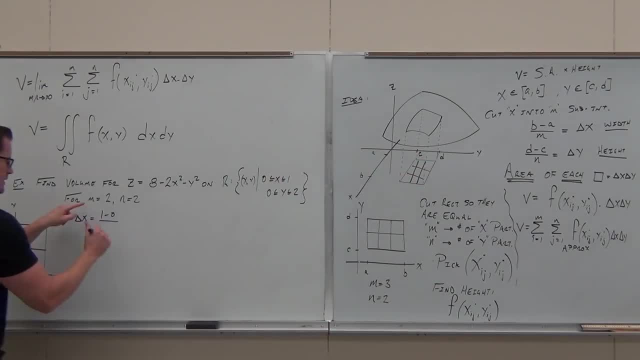 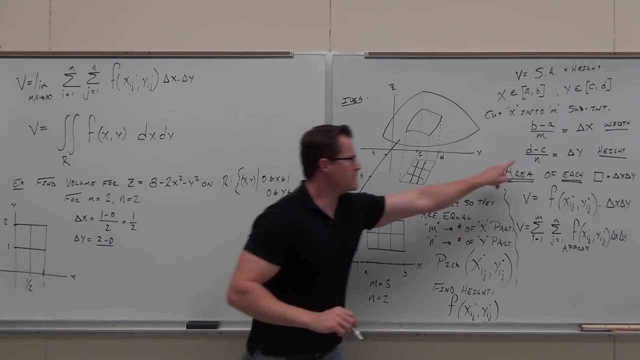 number of cuttings for x. That's two. You have to get one half. as our picture shows us, It's got to be Delta. y says: let's take our bounds for y, Let's cut them by the number of cuttings for y. 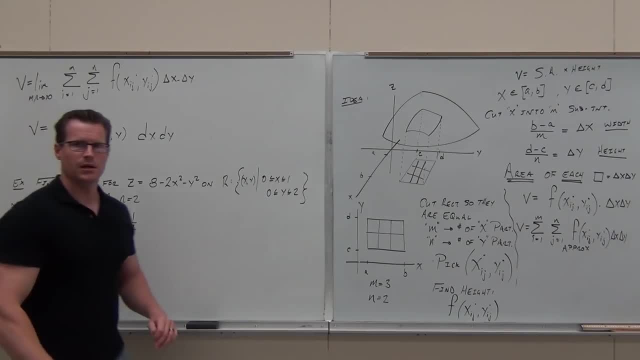 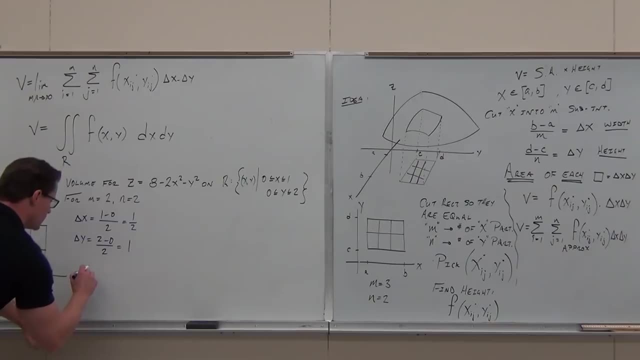 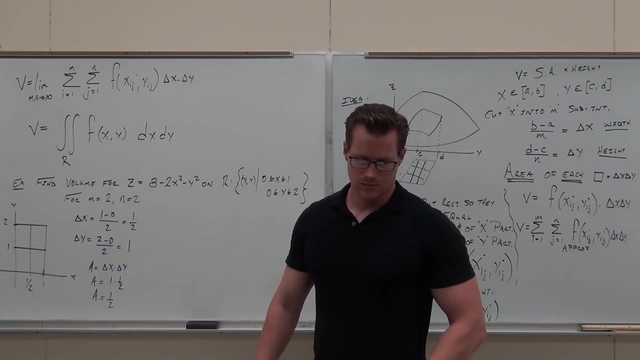 Hey, it's given to you two, And that gives you one. Let's, furthermore, find the area for every one of those equal rectangles. That's easy. Okay, Y'all okay with that. We have a special special thing for this. 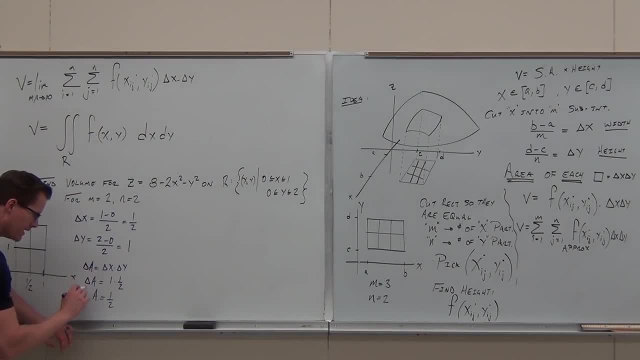 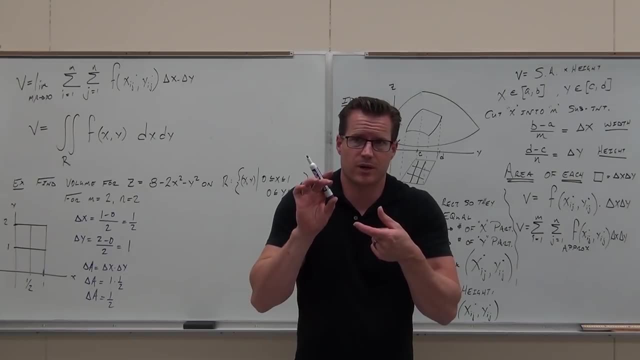 We typically don't call it just a. We call it delta a. Okay, Because that area is. if we let it go to a limit, that area is going to shrink to zero. also, If delta x and delta y are both shrinking to approach zero, delta a is going to shrink. 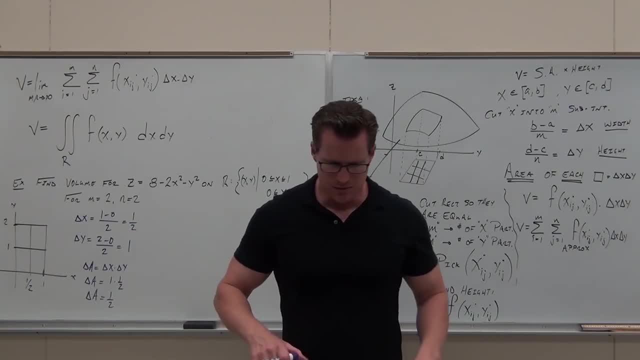 to approach zero. Does that make sense to you? I know it's new notation, but it doesn't really affect us that much. Now, how many rectangles did this create for you? We're going to find the area using lower right corner points. 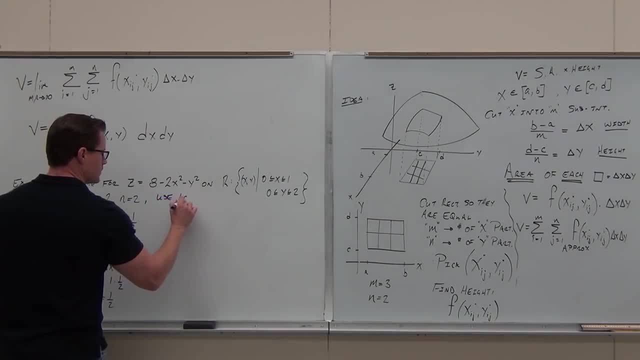 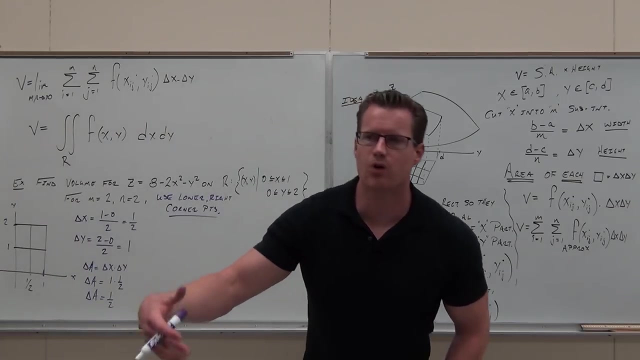 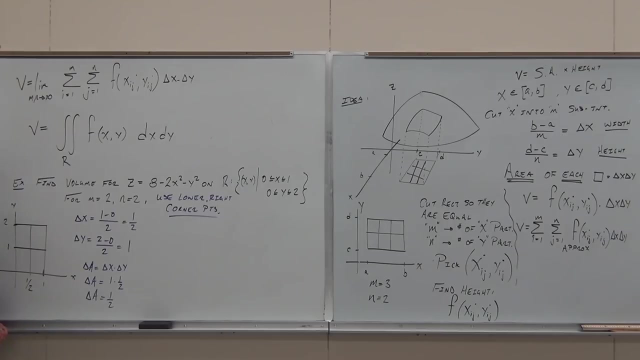 Okay, Okay, Okay, Lower, right now that I just really have this clear lower right corner points. So on your grid, why you draw a region on your grid? let's look at this. Can you tell me where the lower right corner point is? 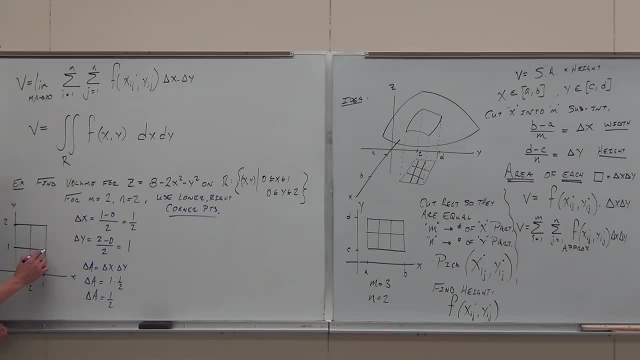 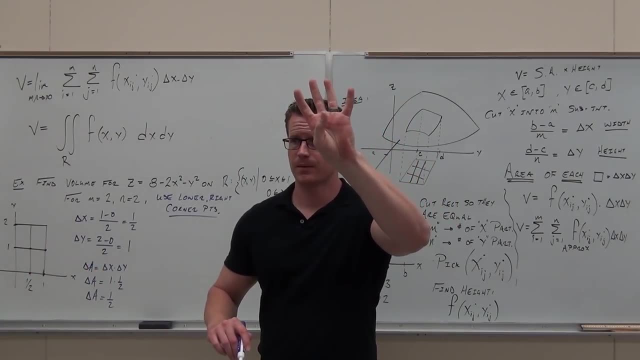 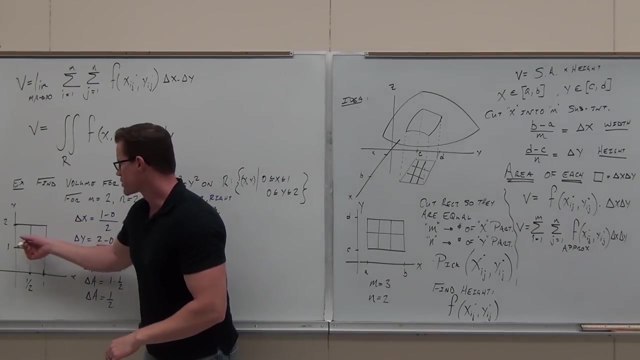 There, there, there and there. If there's four rectangles, you may only put down four points. Points equals rectangle, Number of points equals number of rectangles. Does that make sense? We typically choose corner points, one of these- or center points. that's the hardest, not super hard. 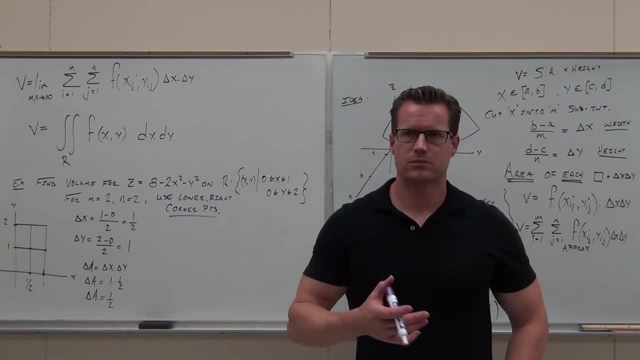 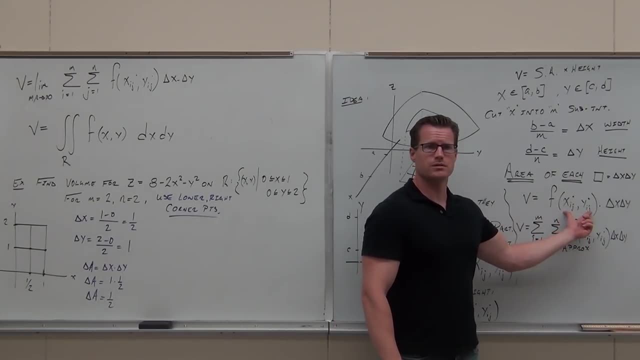 but it's the hardest to do, And then, well, follow the formula. What the formula says is: hey, I want you to plug in those points, which is final height. add it up first, because all the areas are the same. 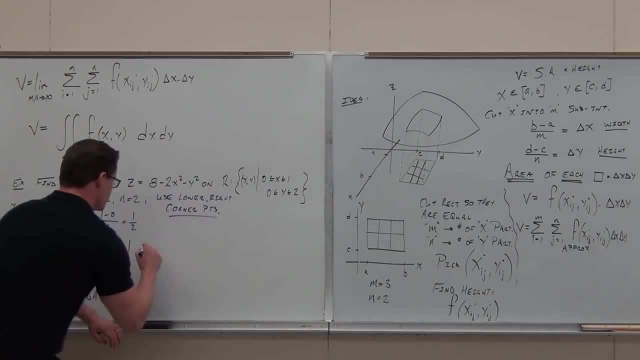 multiply by the area last. So our volume- I'm not going to put equals because it is an approximation- Our volume is going to look like this: Let's find f of list out. let's go slowly but list out my corner points. 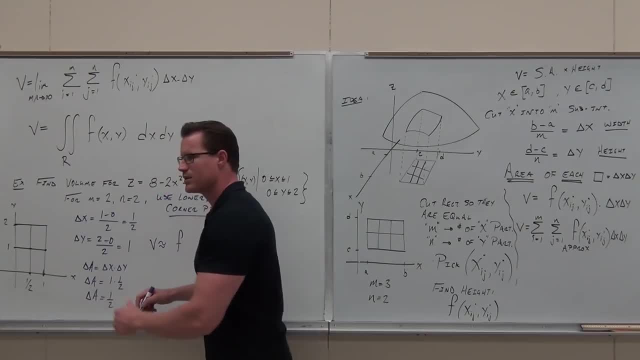 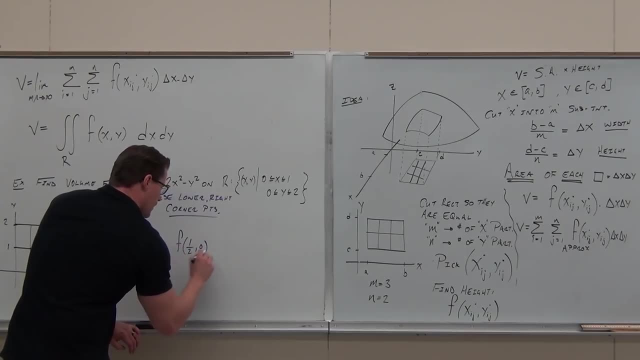 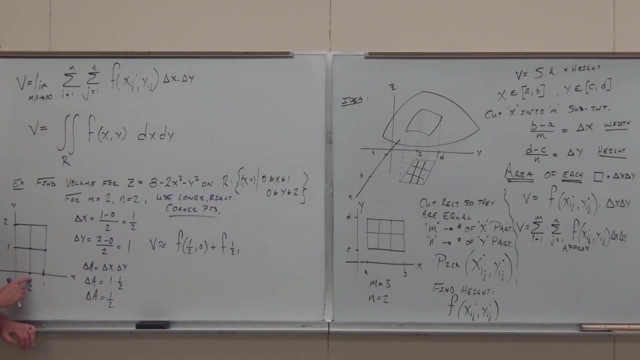 The first one, then second one, third one, then fourth one. Can you list out the coordinates for me please? Yeah, one One half zero, okay, and then the next one I'm going to plug in is one half zero. this coordinate is one half one. 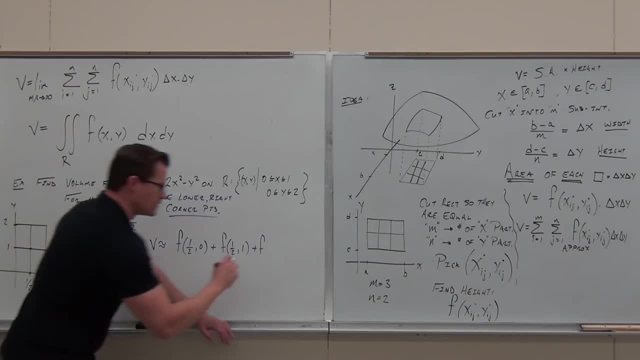 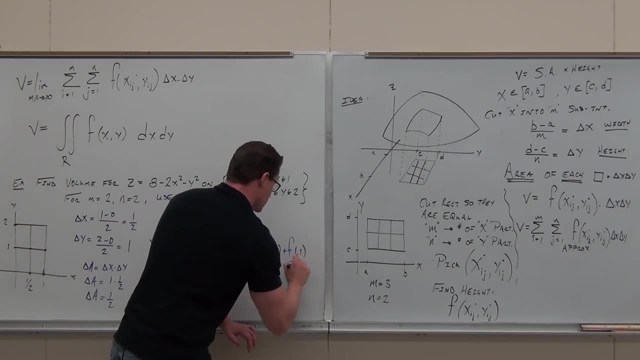 Okay, let's practice this one, everybody. What's this? coordinate One half zero. And then, lastly, this coordinate One half one. Okay, let's practice this one, everybody. What's this? coordinate One half zero. 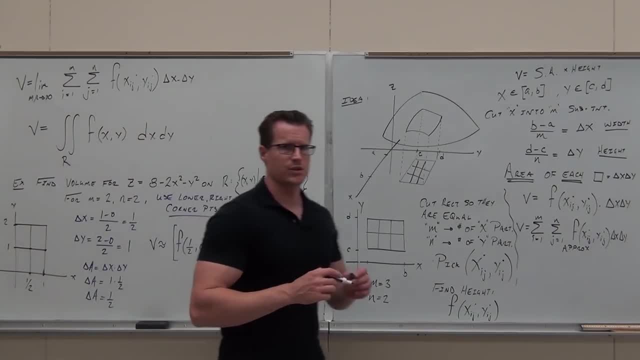 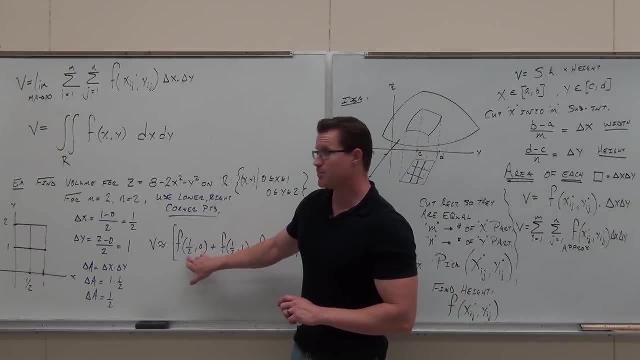 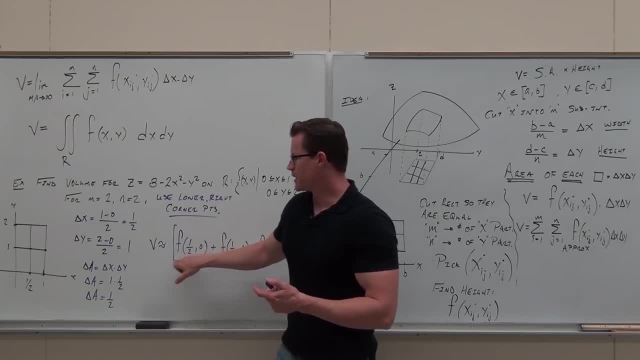 Now I kind of picked it. Does it matter? We picked a point for each rectangle. Did you see it? For rectangles, for points, we plugged in the points to the function. What's it do? When you plug in a point to a function, what's it do? 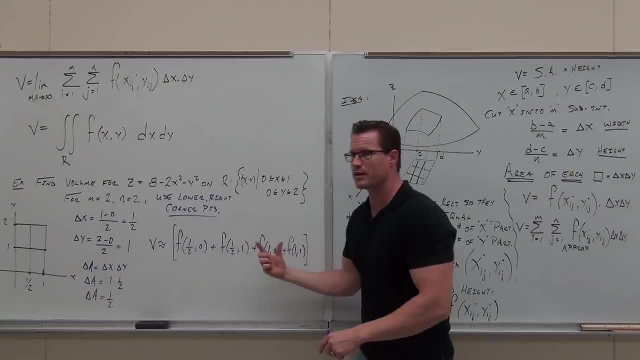 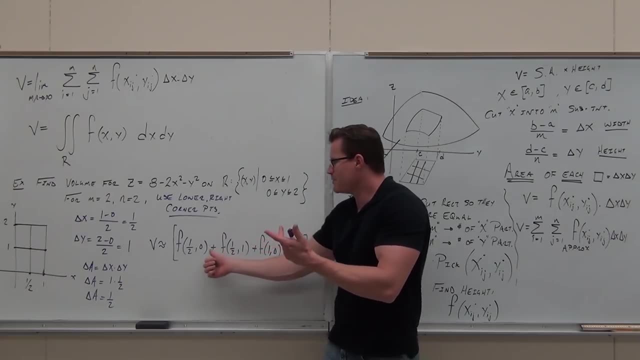 It's height Height. We just found the height at each point. How we find volume is height times area. Okay, Only I'm not going to do it every single time, because if I multiplied every single one of these by the same area, I could easily factor it out. 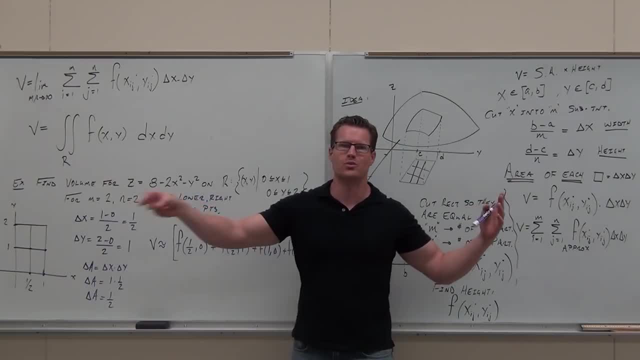 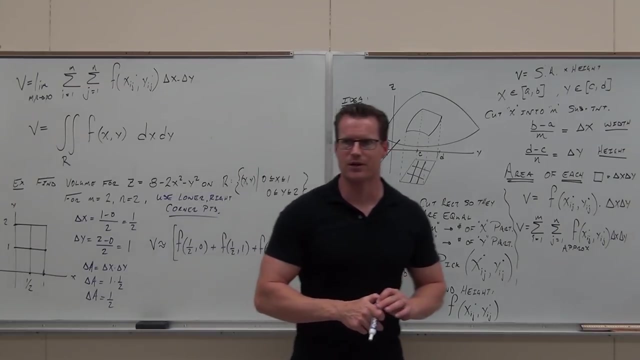 So I'm going to add up the heights first and then multiply by what. what area, Come on. what area Specifically, what area, Specifically what area? Because that's my area for each rectangle. Does that make sense? Now, I've done the one half. 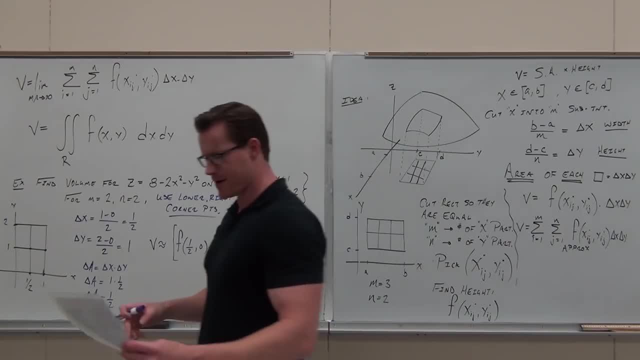 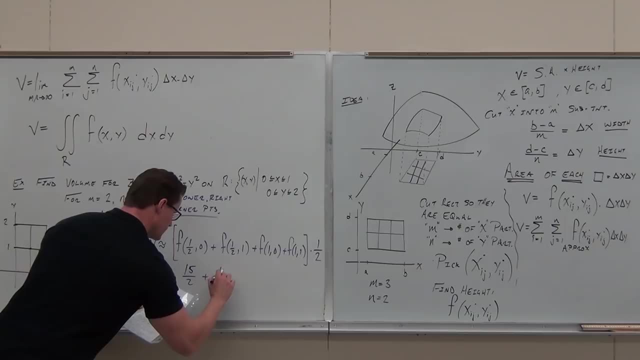 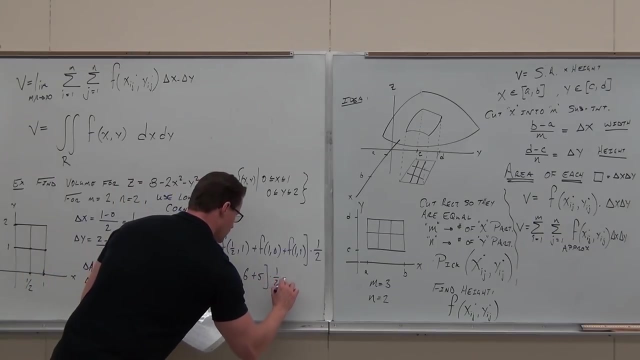 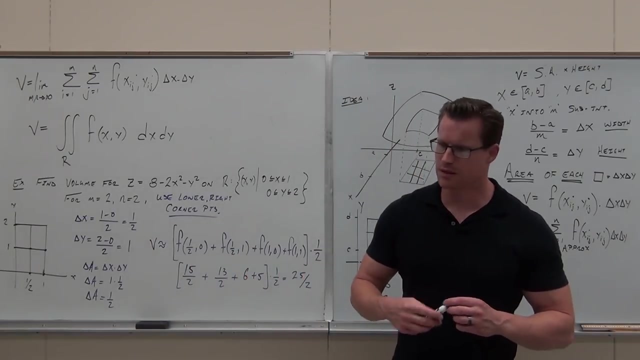 I've done the work ahead of time so we don't burn up our calculator batteries and stuff When you plug all this stuff in. if you want to check your work later, Give me 25 hats. Plug it in later if you want to. 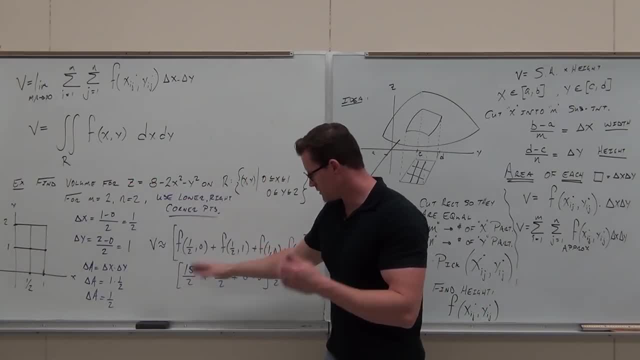 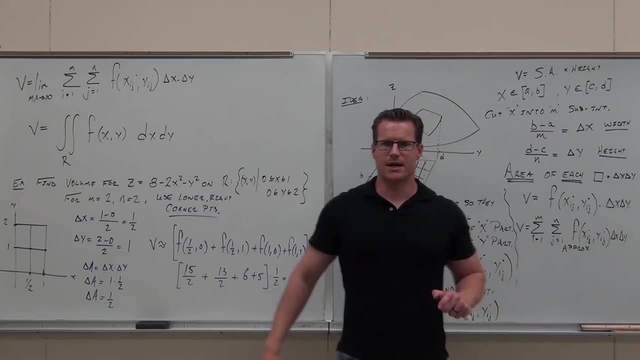 All I've done is took this, plugged it into the function and figured out the results. It's just plugging numbers in. I don't want to waste our time doing that. okay, What's it represent? What is that? What's the whole idea of a double integral? 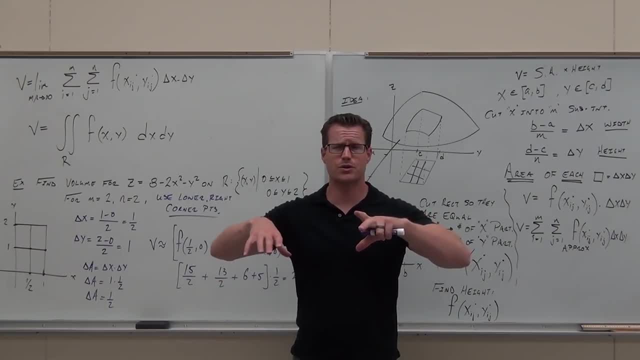 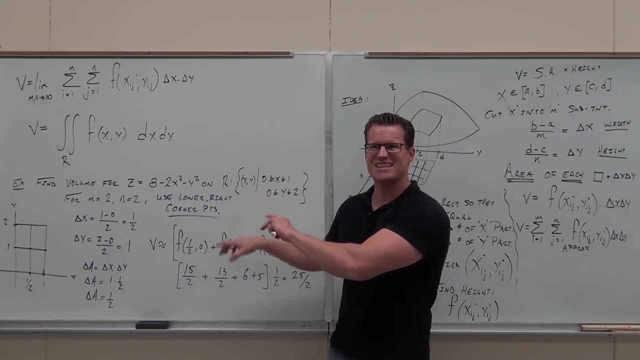 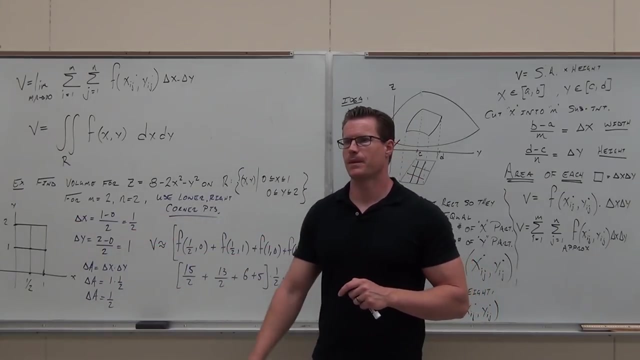 What are we doing? Volume under that surface, but only over that rectangular region, Make sense, Is it exact? That begs the question: If I change my points, will it change my volume Absolutely? Because if I change my points and plug in different values, 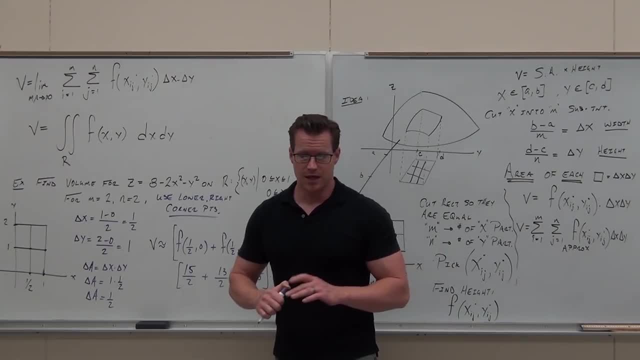 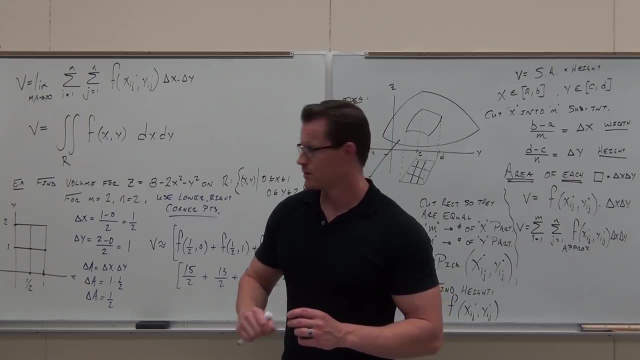 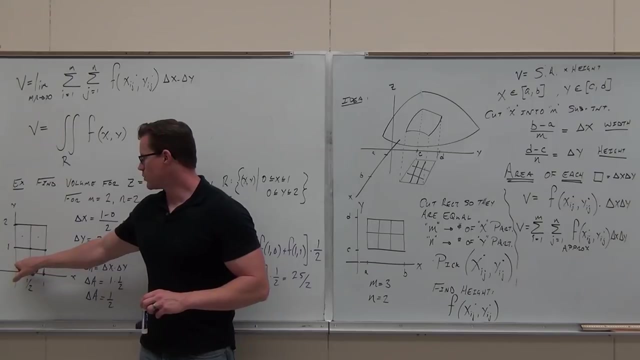 to that function, it will change. As a matter of fact, if you want to try this on your own, if you plug in center points here, here, here and here, that would be one quarter, one half, three quarters one half. 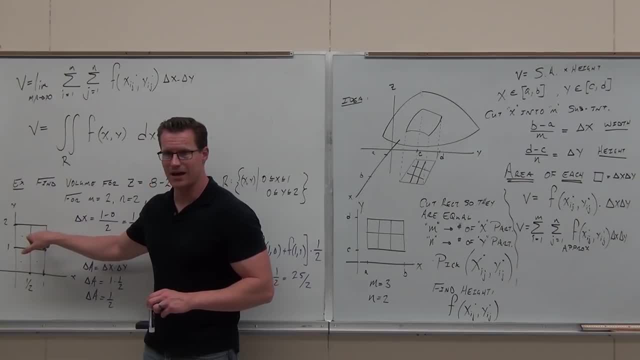 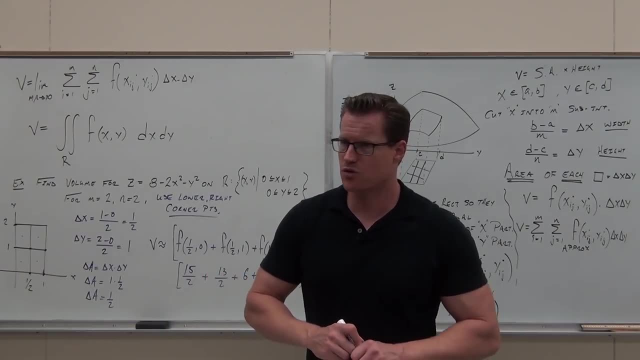 one quarter, one and a half, three quarters, one and a half. Do you see it? Plug in those values. the volume is approximated by 49 over 4.. If you want to check your work on that one, try it. 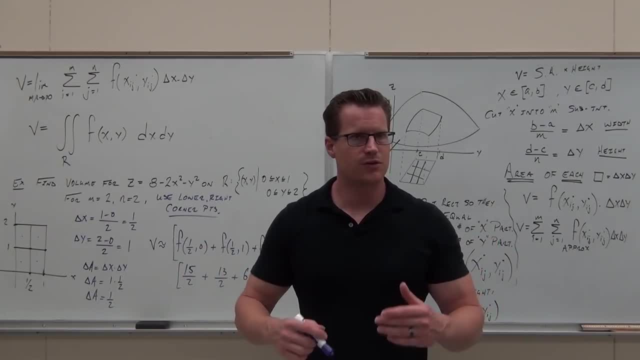 Try it later on your own. I don't have time to do it now. Try it later. See if you can plug in center points and get 49 over 4.. It's off a little bit. It'd be off a little bit, but it's not the same. 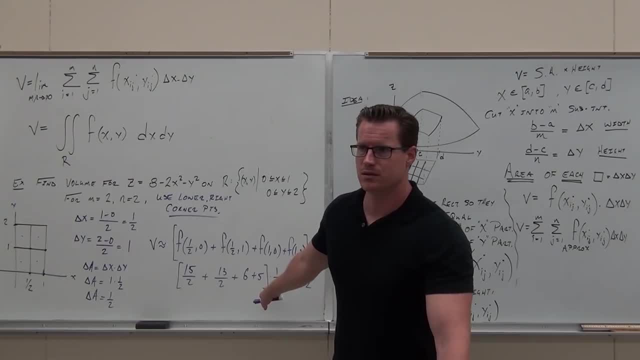 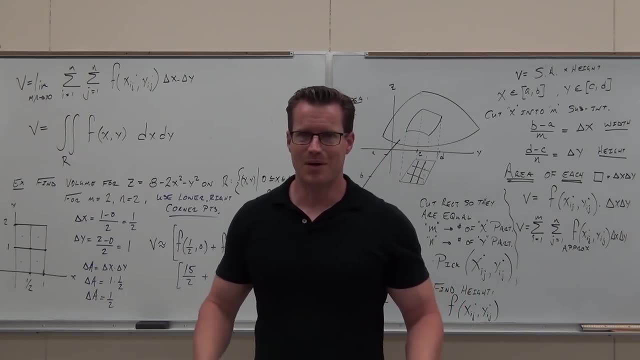 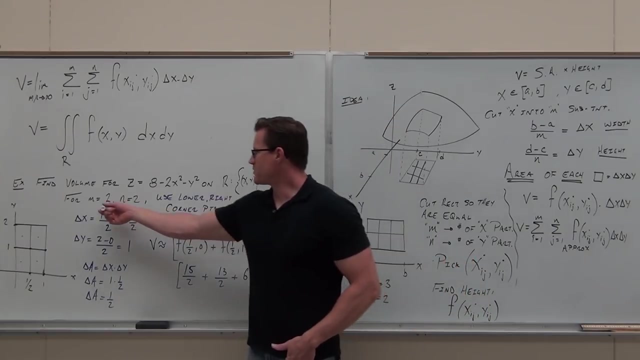 It's close, but it's not the same. This is 50 over 4.. Center points gives you 49 over 4, slightly different. Try it. Am I making sense? Yes, Kind of cool. Yes, If I changed that around and gave you 4, could you still do it? 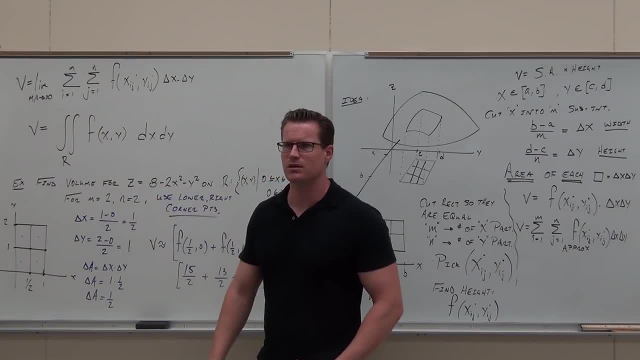 Yes, If I changed that around and gave you 6,, could you still do it? If I changed this around and went from 1 to 5, could you still do it? Picture looks a little different. You have a different number of rectangles. 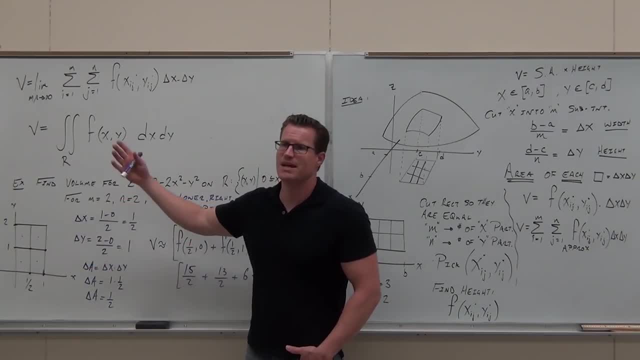 Here you have 4.. 4 rectangles 2 times 2. If I gave you 4 and 6, you'd have 10 rectangles. That's 10 points to plug in. But the idea remains exactly the same. 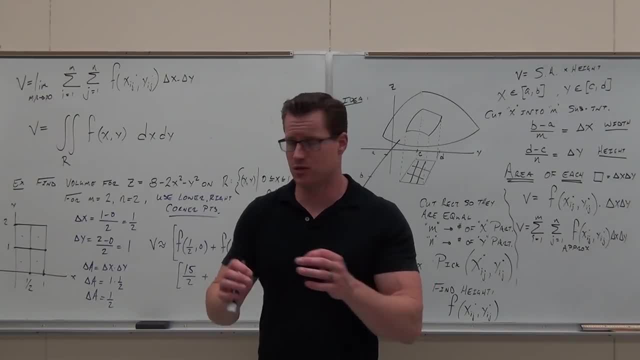 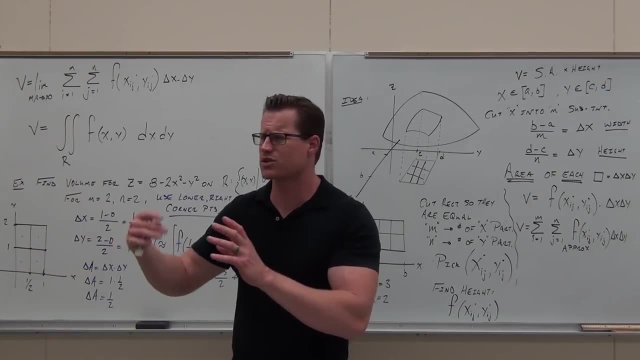 I don't want to do another example because they remain exactly the same. If I choose, you tell you to choose left, lower left corner points or upper left corner points, or upper right or center points. do you feel like you could do the work on it? 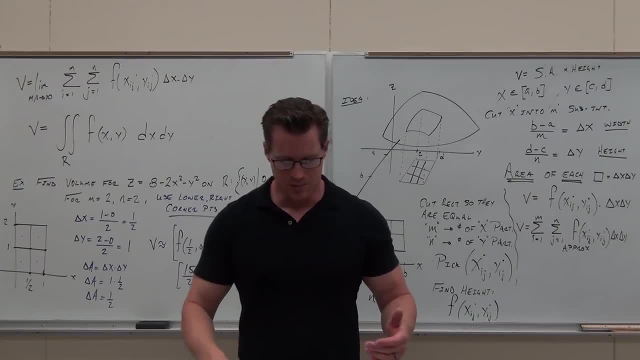 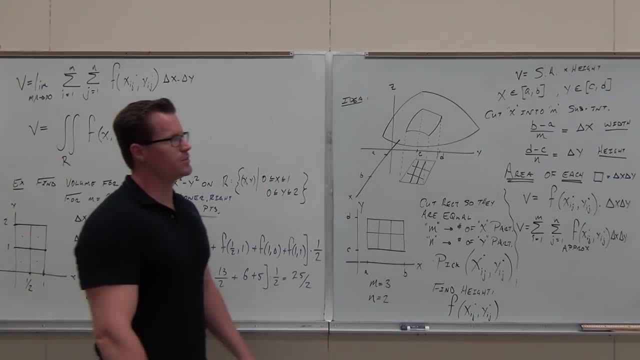 Because actually I just wanted to get down to here and do 1 to show it, And I'm going to show you one more thing and I'm going to answer any questions after that. okay, So This also. basically, you guys probably have the question in your head. 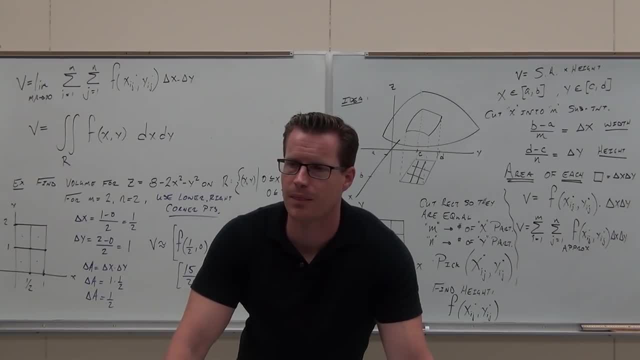 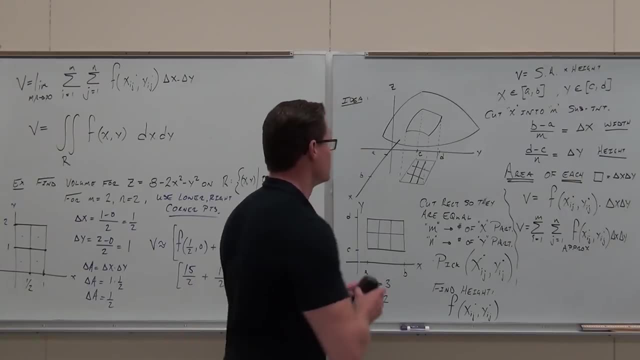 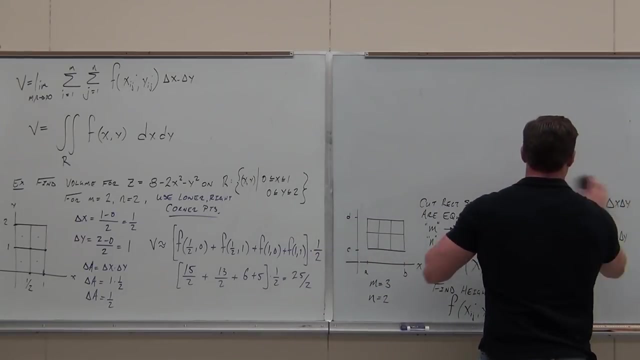 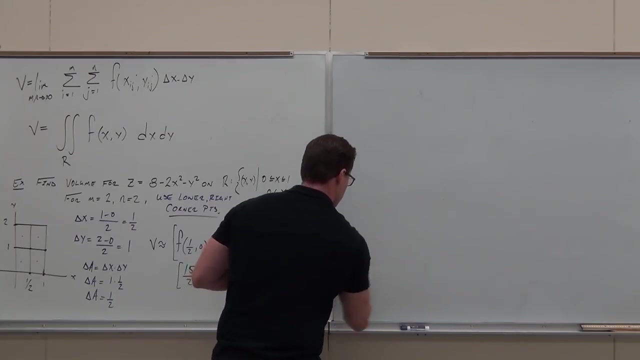 Are all regions rectangular? Yes, Okay, Can you draw me a region that's not rectangular? Yeah, I can. No Rectangular? Yeah, Yes, You think so. Yeah, We learned a lot in geometry, Oh wait. 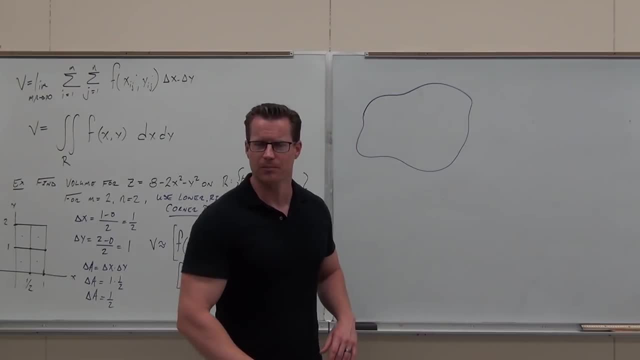 Oh wait, We don't teach geometry here. All right, Ladies and gentlemen, I'd like to introduce to you a closed bound figure which is not a polygon, nor is it even a rectangle. This happens to be just a simple closed curve. a region on the xy plane. 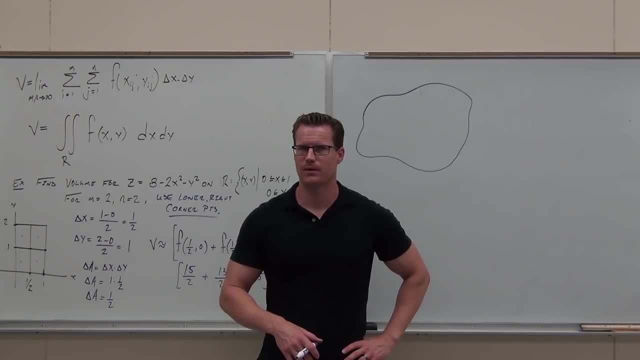 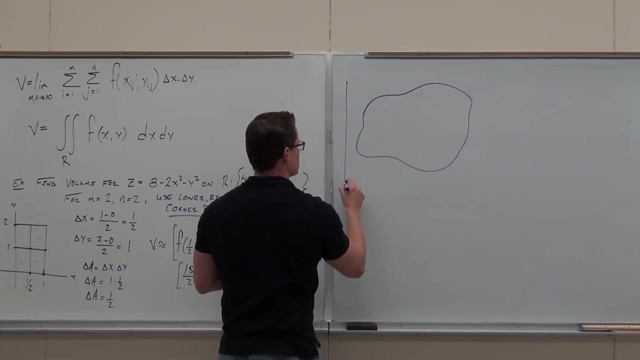 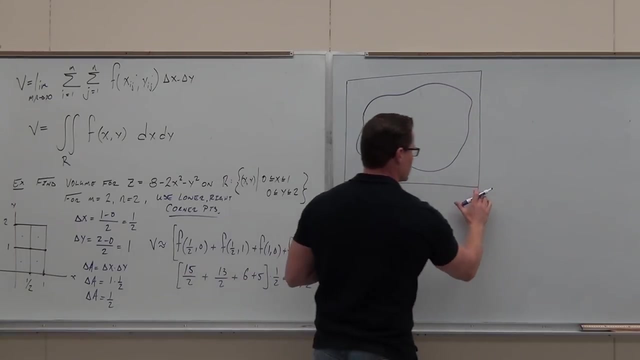 With me, Not a rectangle. However, verify this, just logically. if it's closed, it can be bound by a rectangle. Put a rectangle around it. I try my best to do a big rectangle. It can be bound by a rectangle. 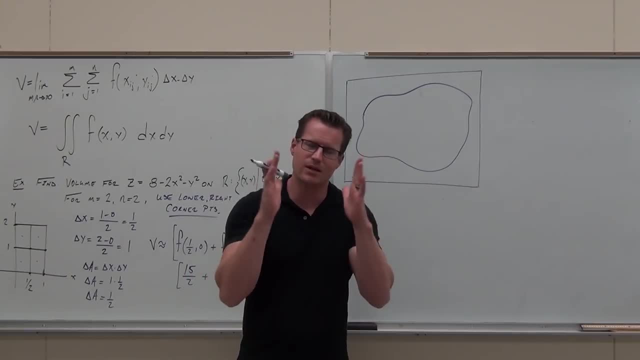 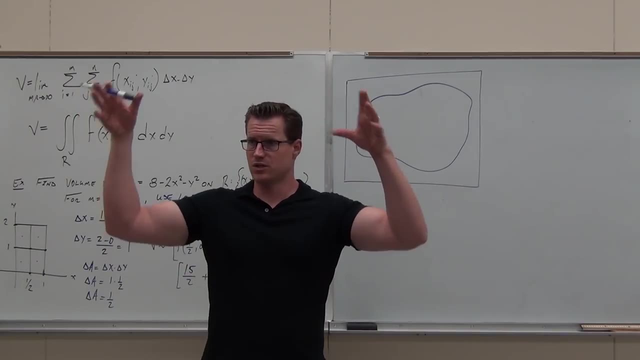 We make it as close as possible, We try to contain it on the edges- I just got a little sloppy here, just to show you something here- And then we go: okay, let's take the rectangular region that has bound, this non-rectangular region, and let's cut it up into some rectangles. 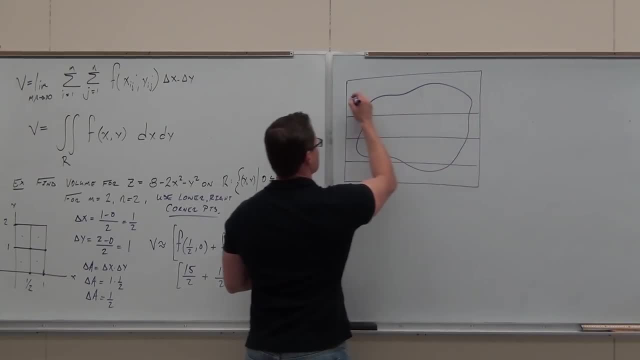 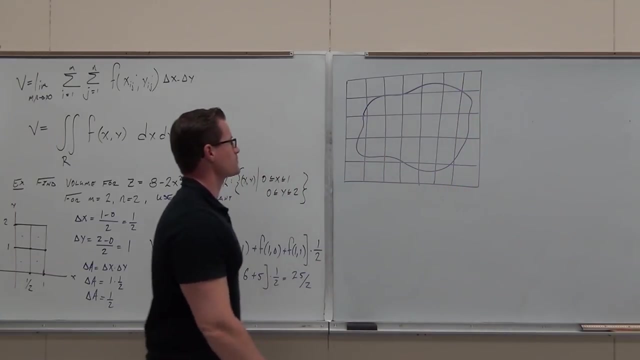 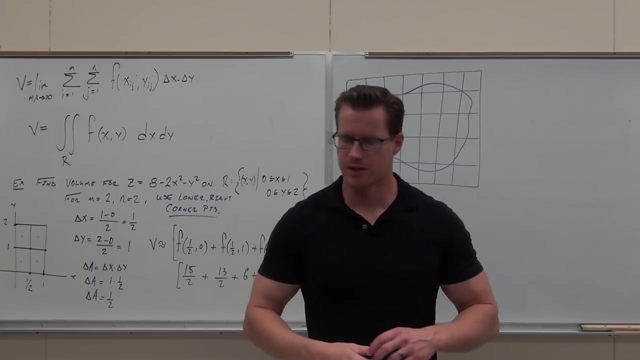 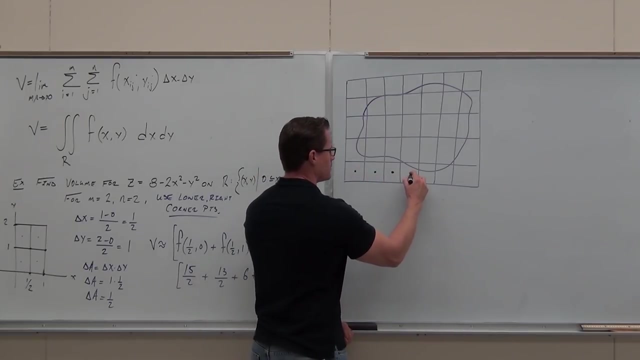 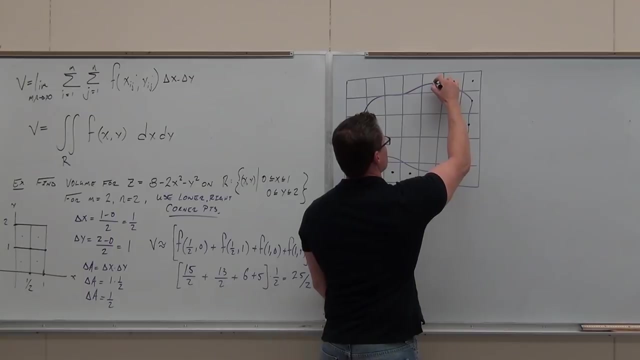 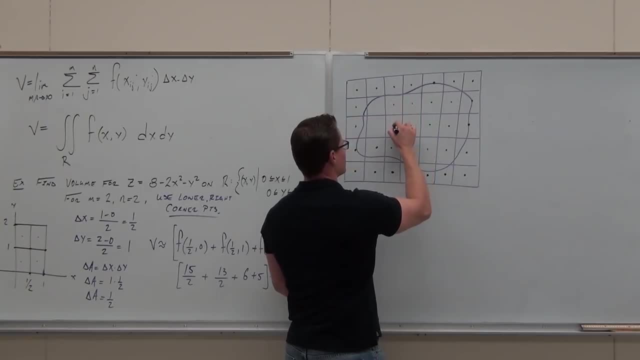 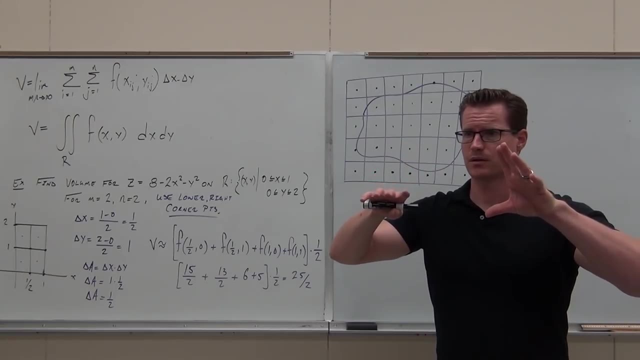 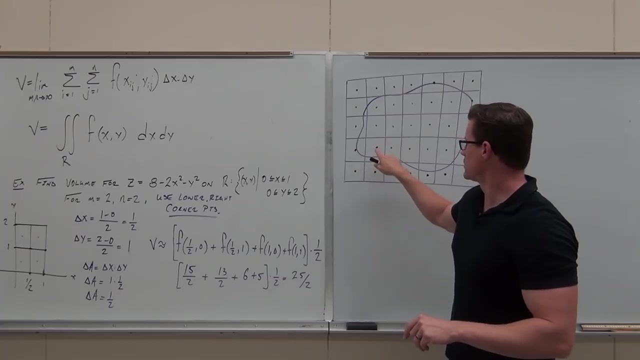 I'm sorry, Here's your idea. here's your idea. Even if it's not rectangular, we can put a rectangle around it, correct? Now here's the magic of it. Could you still, given this rectangle and this grid which you have, could you still plug? 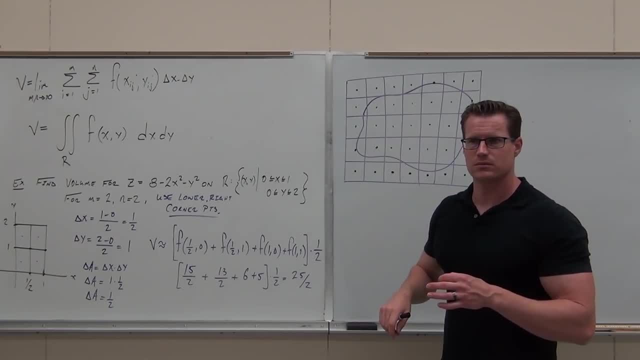 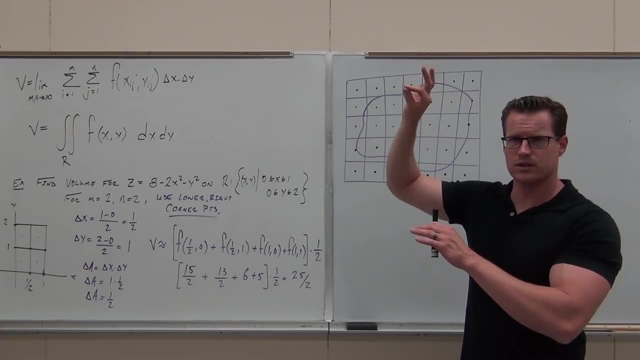 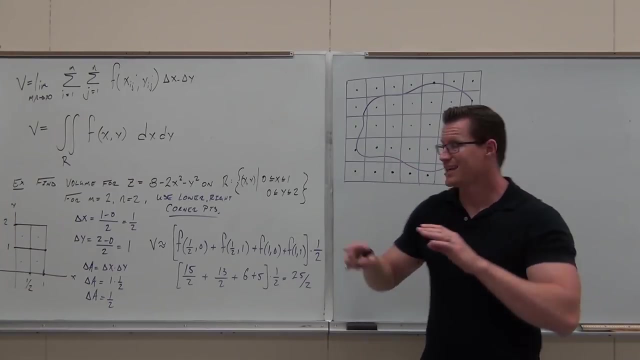 in these points from that rectangle. I'm going to have coordinates for those points. yeah, Could I still find the height of the function above that point? So here's the whole deal. If, even though this goes outside of some rectangles, if the point you're evaluating is in the region, 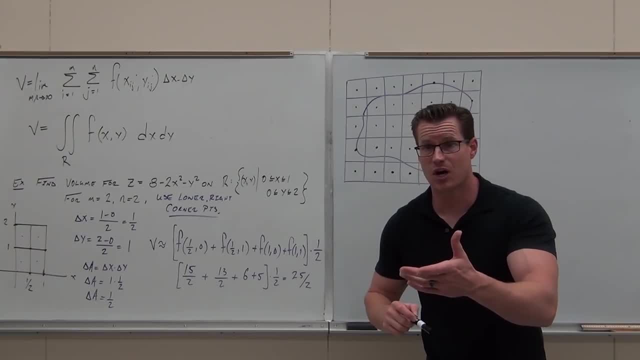 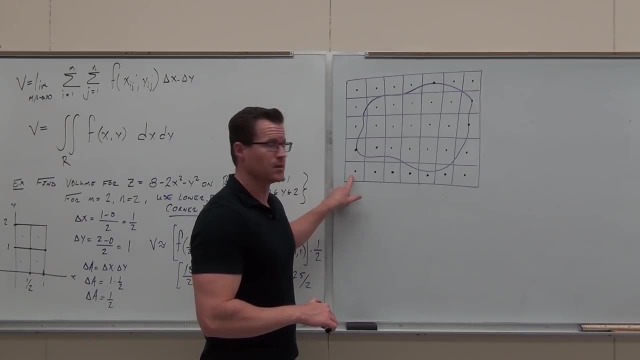 or on the boundary, you include it. If it's not, then you don't. So would we include this region or this rectangle's volume in the sum? How about this one? how about this one? this one, this one? 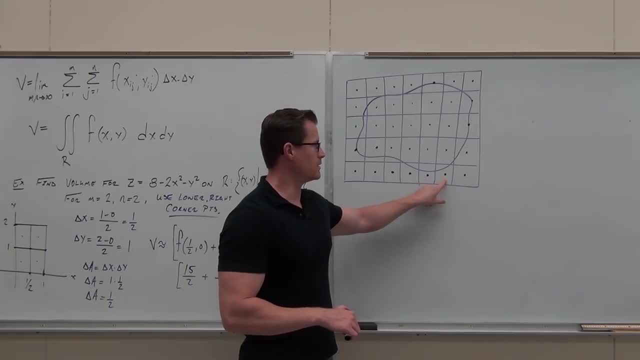 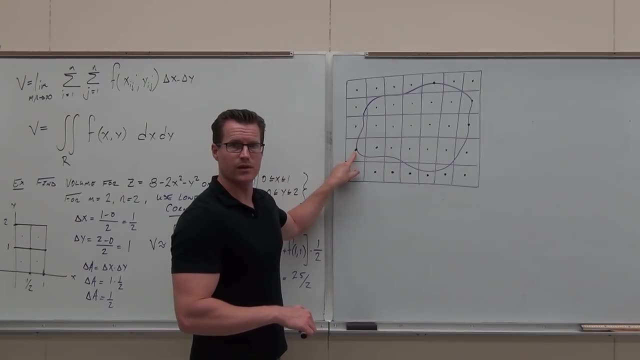 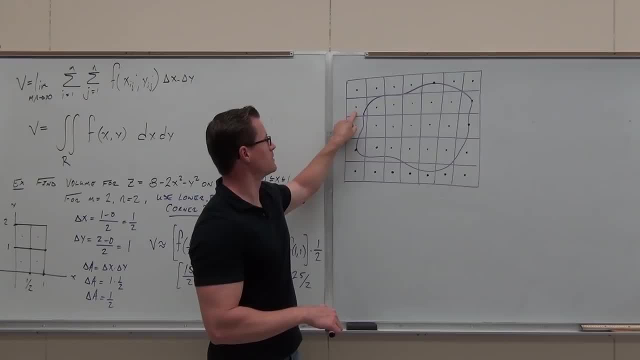 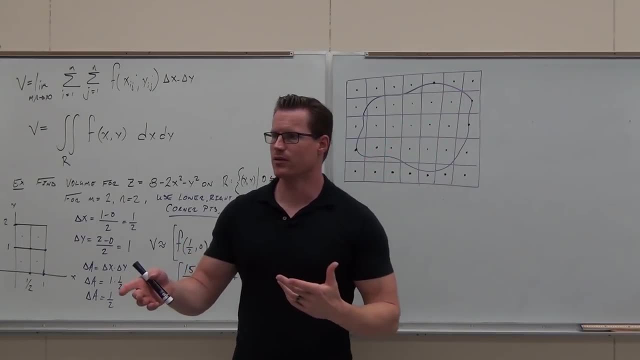 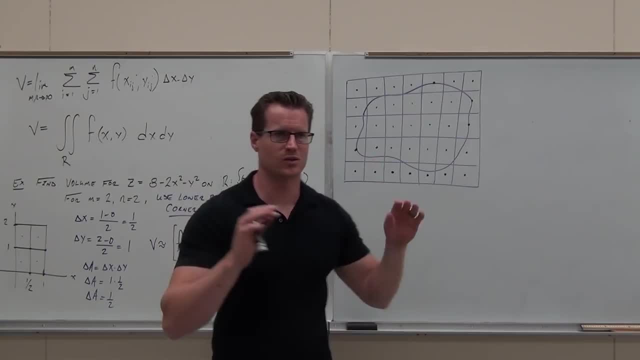 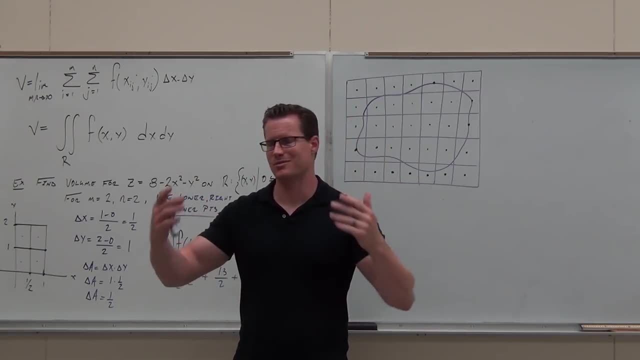 we're going to have an infinite number of rectangles in there, right? Infinite number of rectangles means those boundaries are all going to be center points. Every point is going to be some center point of a rectangle. They're all going to be included, everything. 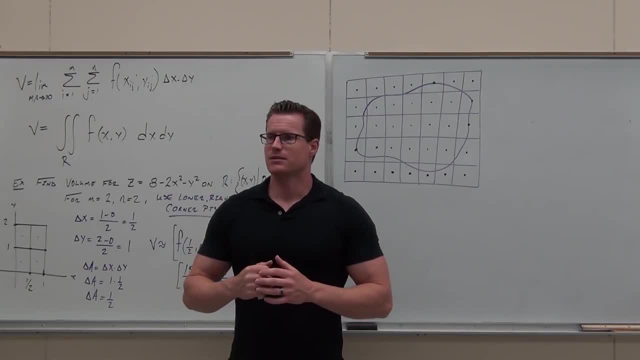 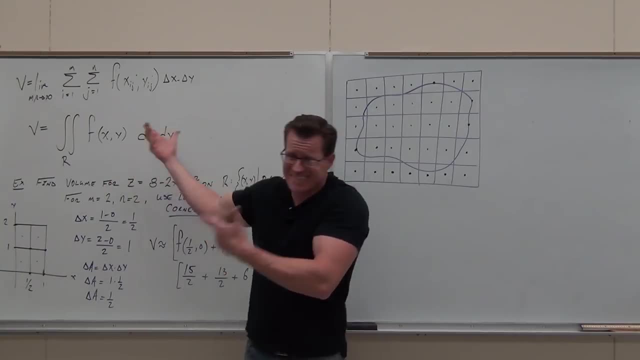 And then, if there's an infinite number of them, we add them all up. that's a volume of a surface over a non-rectangular region, And it's exactly the same. It's the same. You can see it. You can see the same thing. 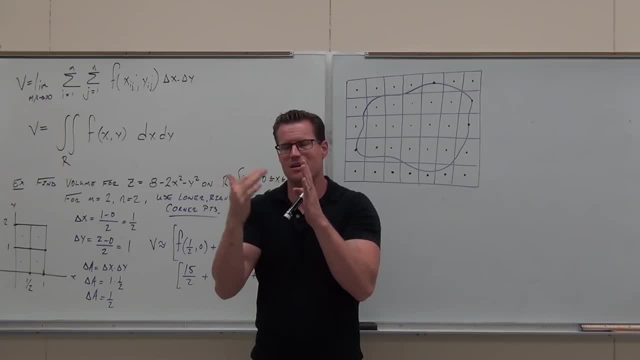 It's taking all the rectangles. There's still rectangles, guys. There's still rectangles Still adding them up across big old grid. It's just, if the points you choose aren't in there, you don't include them. Well, that doesn't matter, because if I take infinite number, 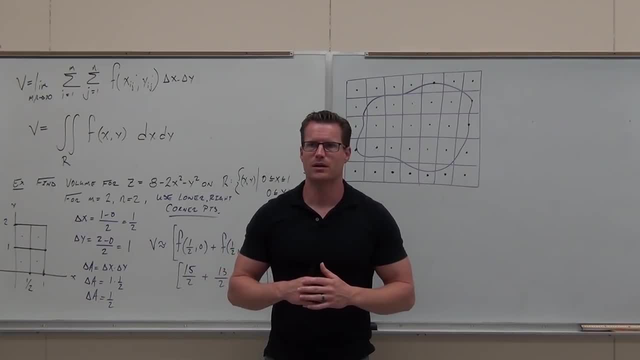 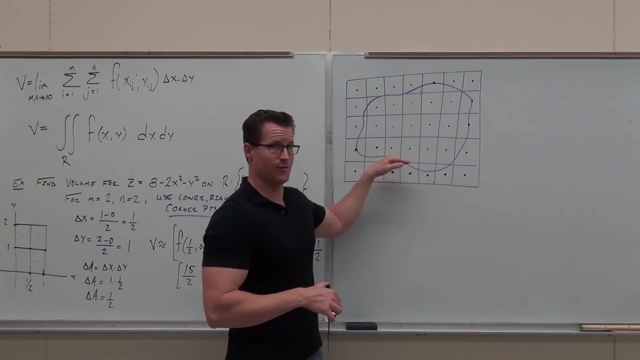 all the points are going to be included. That's the point. Also, I'll prove Fubini's theorem for general regions. You ready for it? Does it matter if I add them up this way, or if I multiply? does it matter? 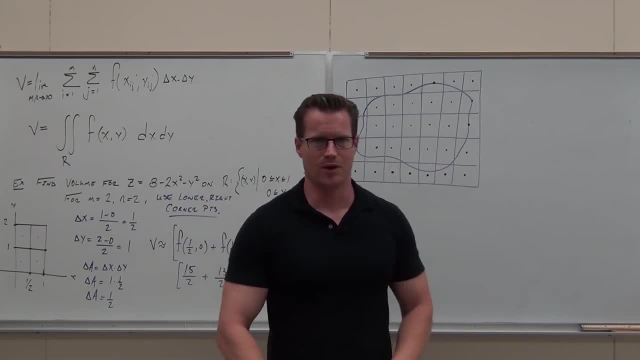 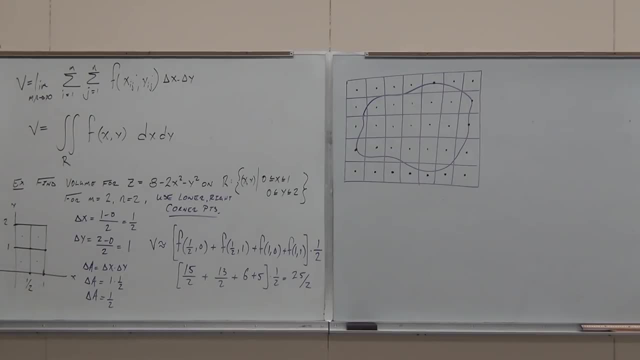 Switch them around for non-rectangular. There Prove Fubini's theorem twofold. What Is this stuff cool, or what? Yeah, Oh, it's cool, Oh yeah, And we're done, So that's good.